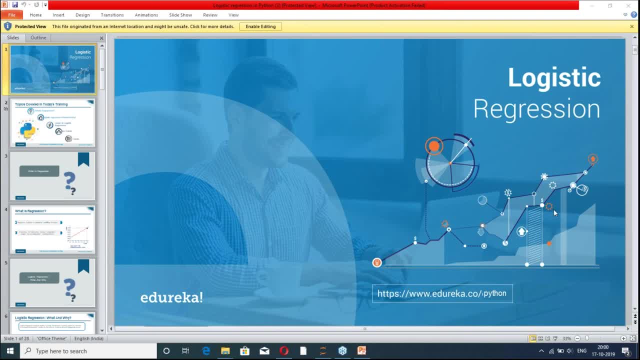 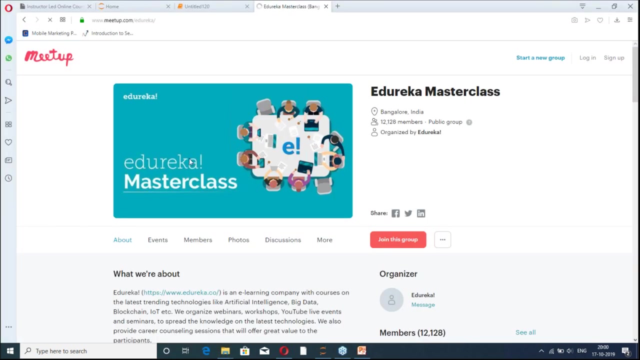 Am I audible? Yes, Okay, great. So let me just Okay. so let me show you first of all this meetup page. I hope some of you already who had been to earlier lectures might have already enrolled for this meetup group or joined this meetup group already. 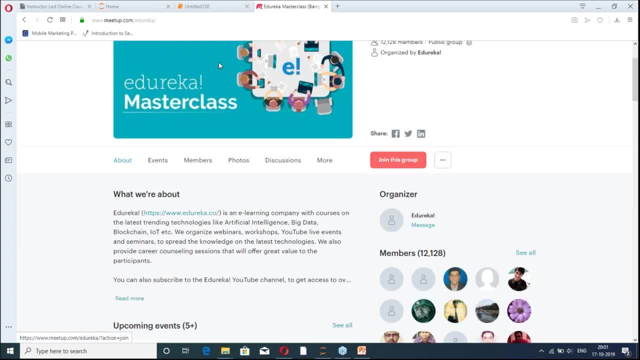 And other people also who have not joined yet. they can also join this group by visiting this particular page, which is meetupcom, And then you can click on this particular link, which is join this group Right, And after joining this group, what you will get: 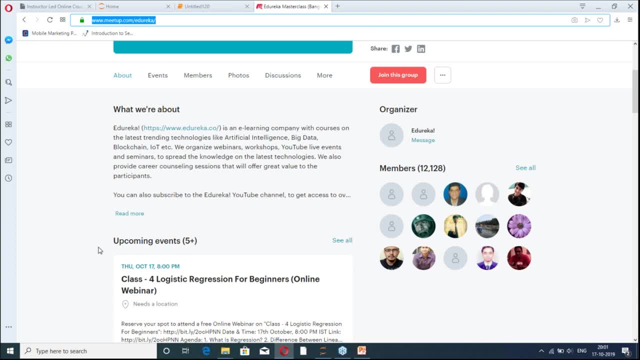 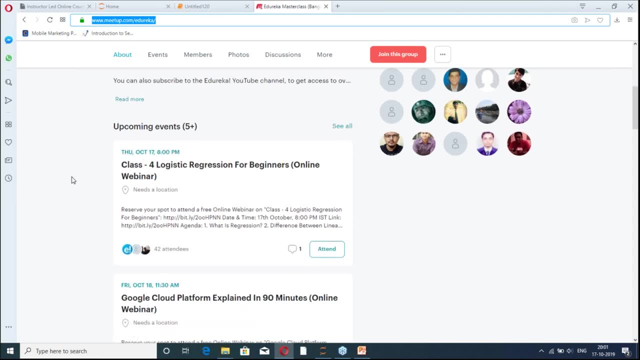 You will be able to get a lot of free webinars And you can ask the questions to the instructors as well, And there are around 100 plus webinars which are being conducted every month. So if you want to take the benefit of these webinars- free webinar series- you can enroll for this by joining this group. 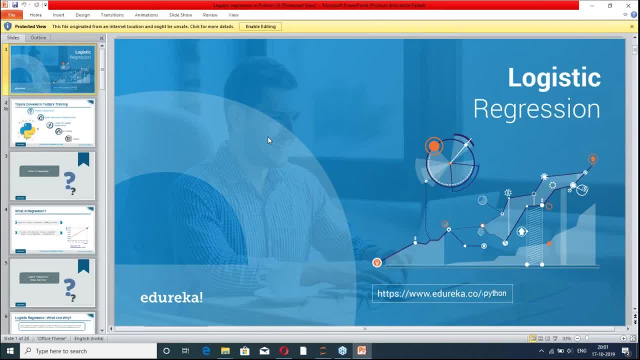 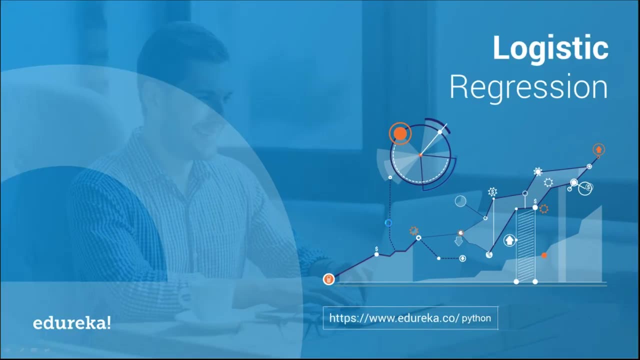 Okay, so now we are going to start today's session, And today's session is about logistic regression, Right? So let's see, Let's see, exactly, Let's just get the full screen here, Okay, so what are the topics we are going to go? 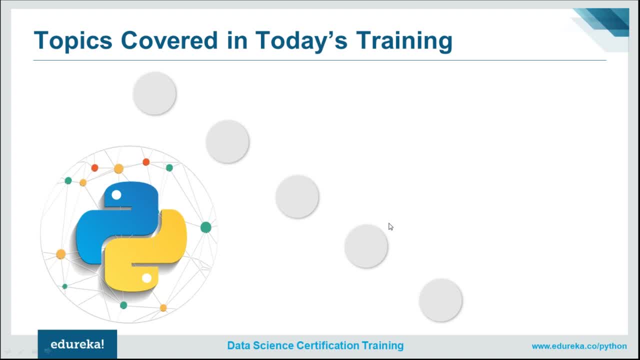 We will start with the regression Already. some of you might have understood what is the regression, Right? So we will start with the regression only, And we will see that after that. logistic regression here, Right? So what is special about the logistic regression? 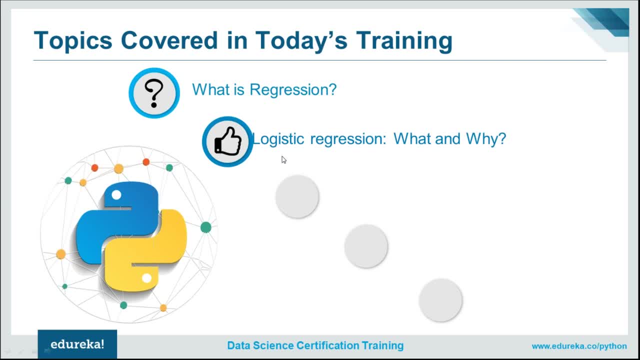 Yesterday we started studied about the linear regression, And when we studied linear regression, we studied about the linear regression. I told little bit about other things as well, Like if sometime it might not be on linear curve but it might be polynomial curve. 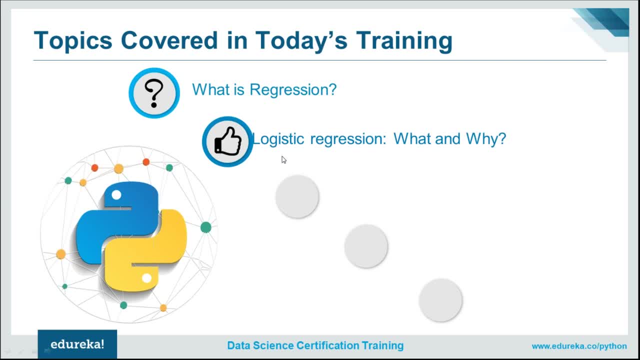 Okay, so we understood. Okay, linear regression is there, polynomial regression understood, But what is that special thing is coming, which is logistic regression, And then we will discuss about linear versus logistic regression. What is the difference between both of them? 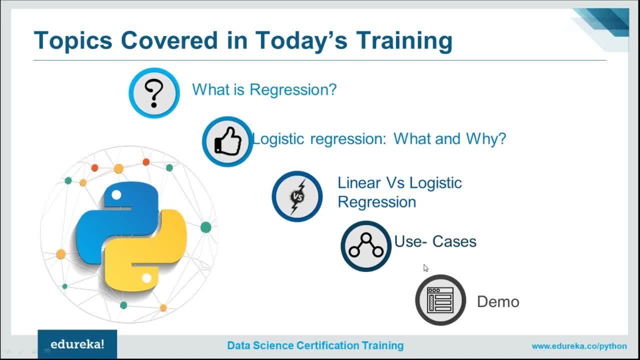 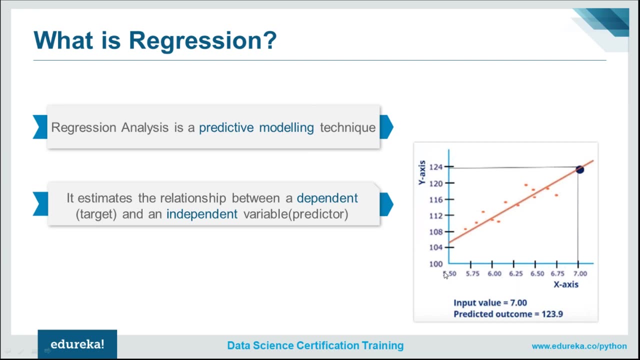 And then we will see some use cases And at the end we will have action in life Where you will be applying on to some data set or your logistic regression. So let's discuss about what is regression. So regression analysis is one of the predictive modeling technique which we have discussed in yesterday's class. 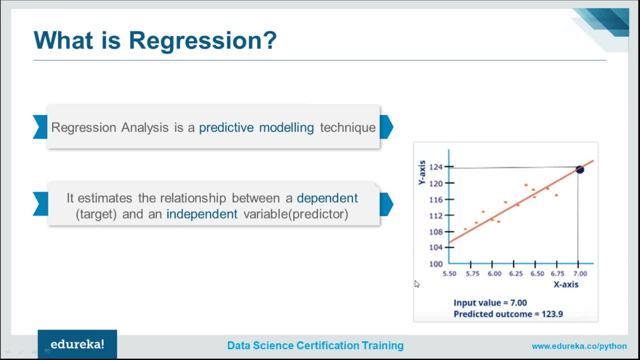 And the whole aim for this particular technique is to estimate the relationship between a dependent target and an independent variable Right. So, like yesterday we were discussing about and we were taking one example, Let's say if tomorrow's temperature depends on what is the today's humidity, for example, 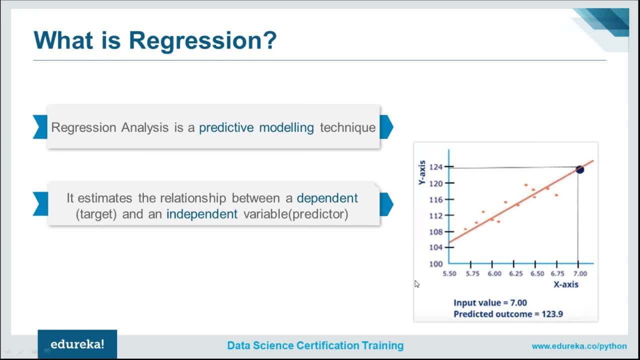 Let's say so, we want to find out the relationship between the humidity and the temperature, right? So whenever we are saying the relationship is linear in terms of like, if there is only one input variable, which is, let's say, humidity, one output variable, let's say, which is temperature, then in this case, if we say, let's say this is a linear regression we are talking about, then you will try to find out a linear curve. 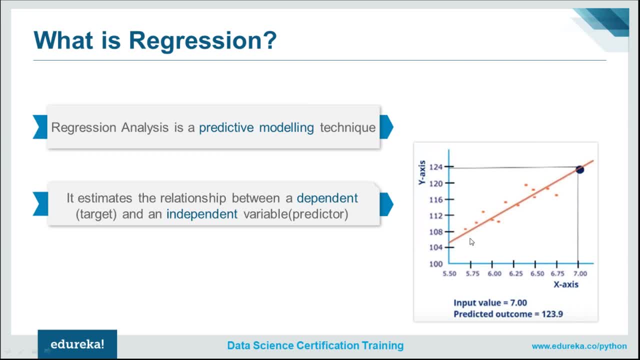 So if it is only a one dimension input value, then it would be A linear line. if it is more than one input variable we have, or more than one independent variable we will have, then it would be a plane or hyper plane, we can say. but it would be only linear only if we are talking about linear regression. but regression doesn't mean linear or just simple linear. if we are talking about it means linear as well as nonlinear. 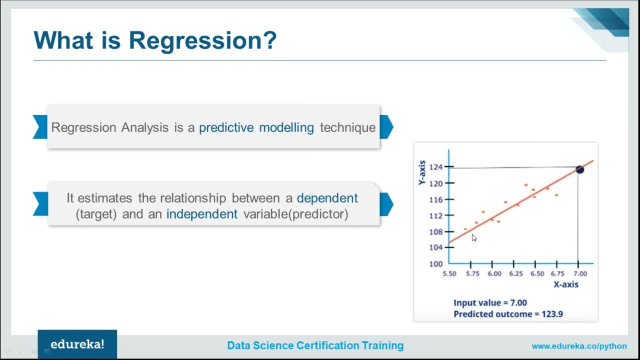 It's not necessarily that your data will always be following a linear pattern. Sometimes it might happen. Your data is following, let's say, sign Wave as well, right? Some of you might be knowing already that what is sign curve, right? 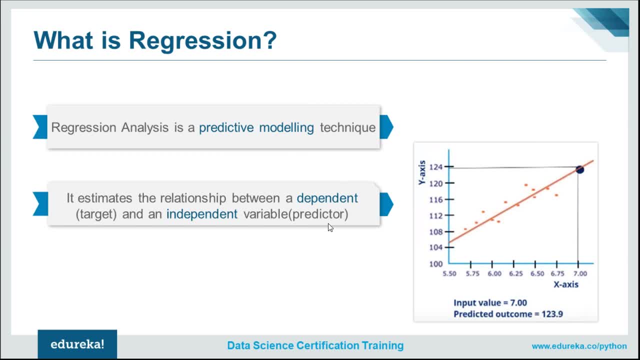 So it might follow any pattern, right? So it's not necessarily that regression need to work with the linear way only, but it might have some polynomial degree or higher degree curves might also be there, right? So the whole thing we can say it is all about finding the equation, how our output variable is dependent on the input variable. 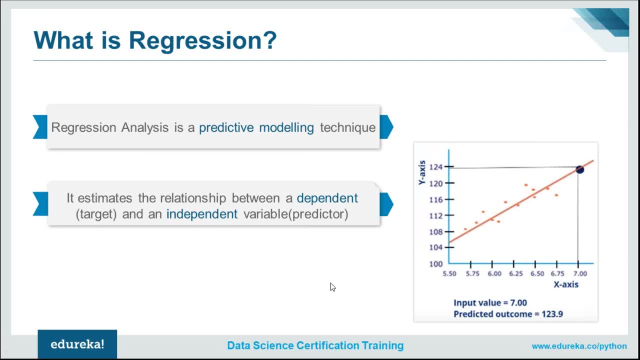 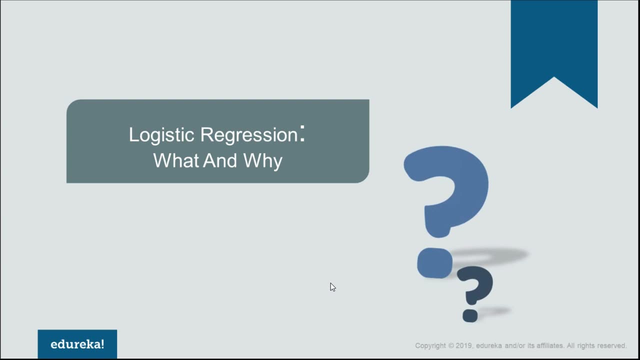 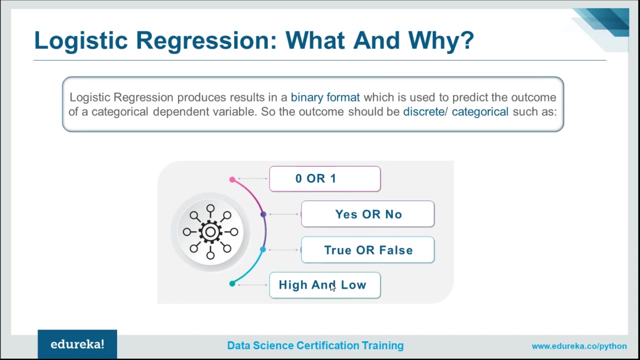 What is the relationship between that? right? Or we can say, finding such kind of equations okay, fine, That's great, but why the logistic regression came into the picture? or what is logistic regression? So if we talk about logistic regression, then it is going to be a little bit different regression, that is, that regression name is coming, but it's still. this is not a regression technique. 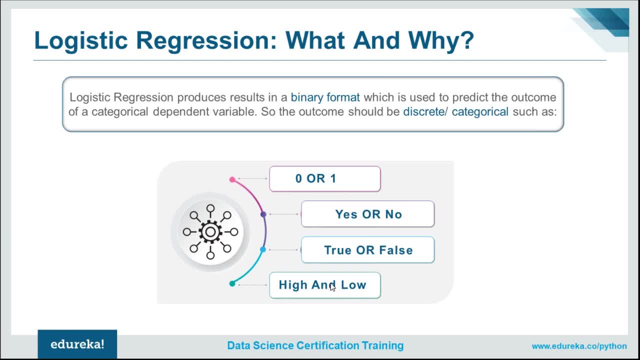 It is a classification technique, right? So we'll be discussing also, then, how it goes, What the name of regression if it is not the regression technique at all? Okay, And so whatever is the classification technique, what we say there, we have limited number of classes, right? 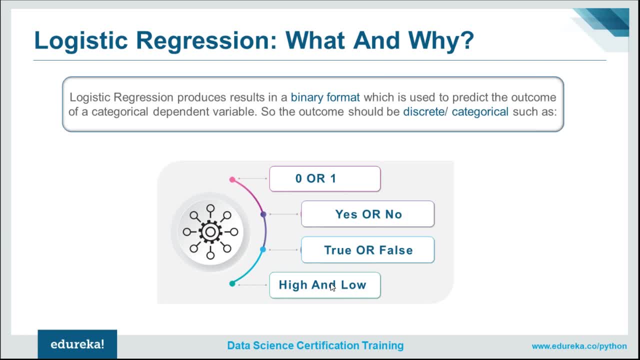 So we saw output classes on there which are limited number right, And then we have talked about logistic regression. It is being used for binary classification actually means the output variable can have only two values, like output variable can have zero or one. 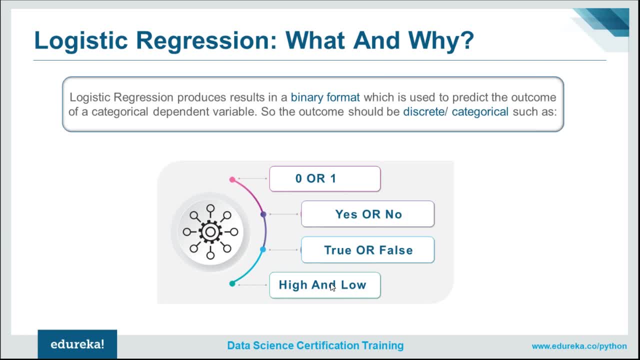 Let's say you are making a model. You will be reading a facial expression of a person who is speaking in front of you. Let's say you make a one machine which will read the facial expression while a person is speaking and it will tell whether it's he's saying lie or truth. right? 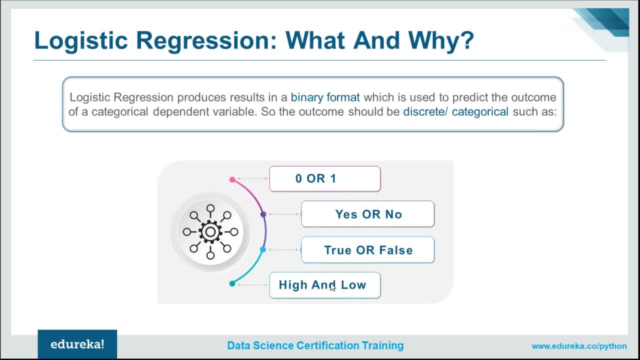 So there is only two outputs. So only two values can be predicted, whether it will predict yes or sorry, it will predict lie or it will predict truth, right? So any such case where output value can be two, that becomes our classification technique. 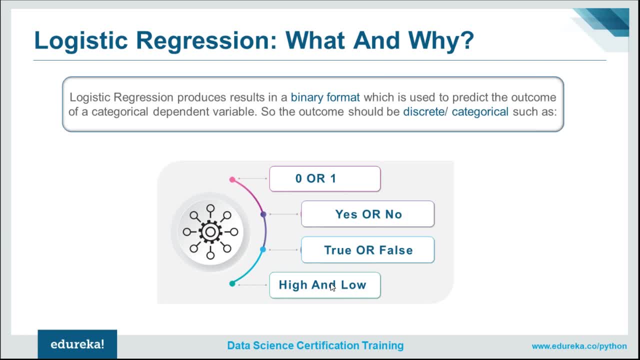 Definitely. But for logistic regression we always say it needs to have only binary classes of means. maximum It can handle only two classes. even though there are ways, if you are interested you can just remind me how you, using the logistic regression or any classification techniques, which is binary classification technique. 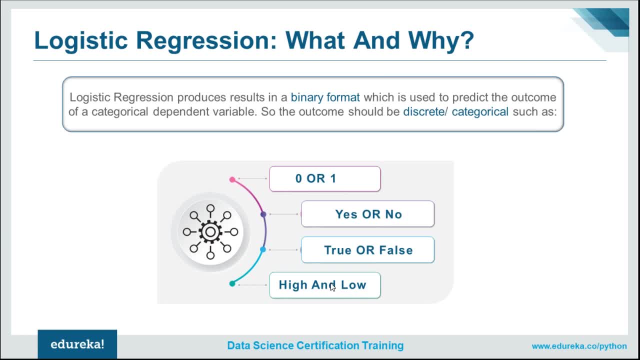 You can handle the multiple classes as well, right? So, even though this is especially for the binary classification, but you can use it for multiple classes classification as well. But you need To do a little bit, which we can discuss at the end, if you remind me. so here this is we, like your case might be zero one, or it might be yes, no, maybe true, false, high, low, right. 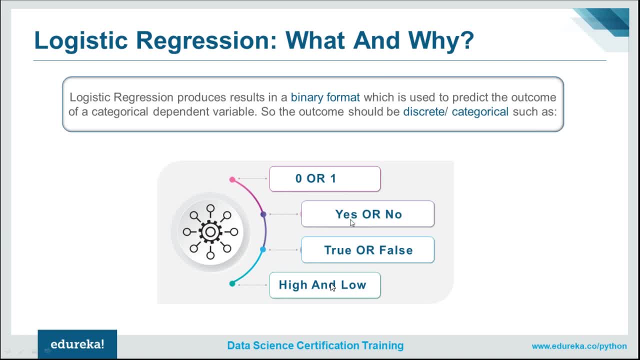 Any case, wherever it can be, two values like truth lie, or it might be having cancer or not cancer, right. All those cases, that is, where we use the logistic regression or classification technique. This was So. now first question arises: 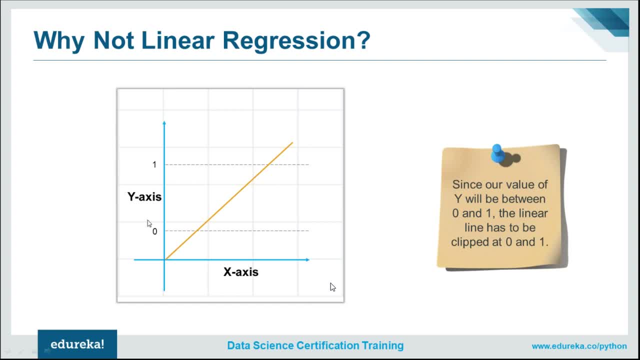 Why I can't do. Leave me a regression in such a case. So if I talk about linear regression, it is like, let's say, if I'm talking about only two dimension again, where one is input variable, which is X, and another is output variable, let's say, which is Y- 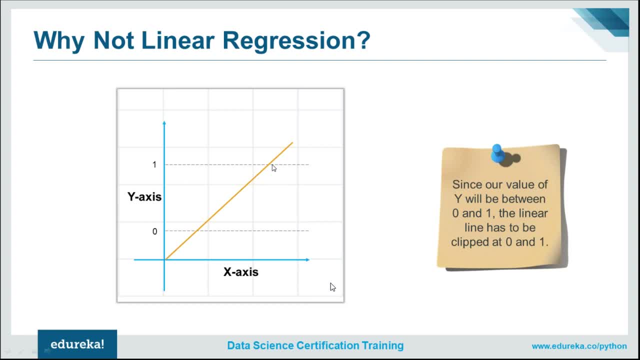 And if I'm drawing a line, so line you know always is going to have infinite venues, right? So if you're talking about why, so how many values it can take over, Why it can take infinite value any line, you talk about only other than one line, right? 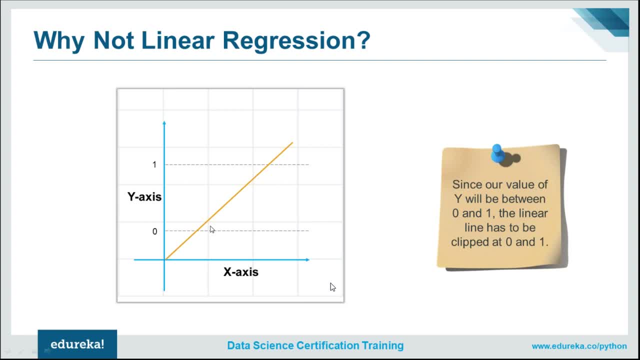 When you say why is equal to some constant values, You will do. five, You say. or why is it going to six? You say: only in that case, why will you speak? That is one. You take any other line, It will always have infinite values of why it can have right. 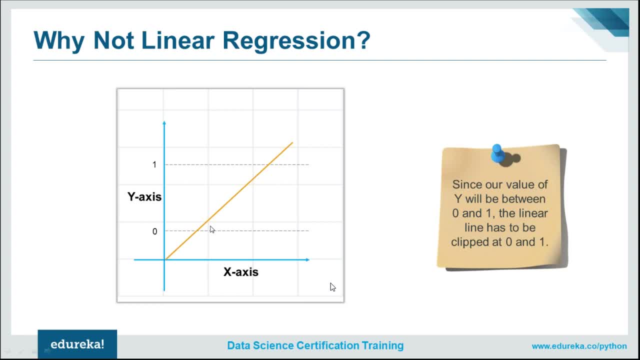 Whenever you write by, is equal to M, X plus C, Then as you change the value of X, your Y is starting right. So if X varies from minus infinite to infinite, so your Y will also vary from minus infinite. But what kind of output we are looking is not infinite possibilities, which is 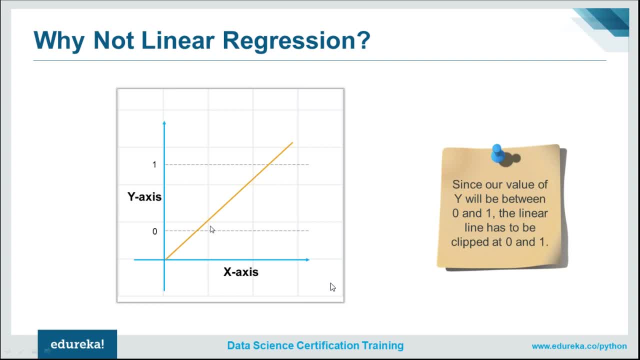 Not infinite possibilities, which is Not infinite possibilities, which is The case in the regression right. We discussed about regression that the regression is all about having infinite number of values It can have right now, because discuss about temperature, We discuss about house prices and so on, but here we can have only two values, right. 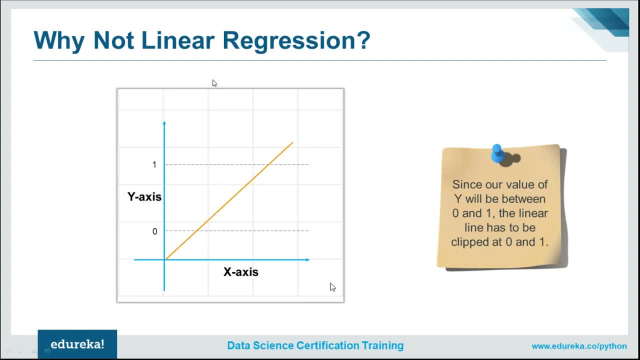 That is zero and one. So one of the way you can convert this linear regression it's itself is that you click this nine right. So, like this line, it is going on. So what are you going to do? You click here so that once it reaches zero, then it is all the zero. 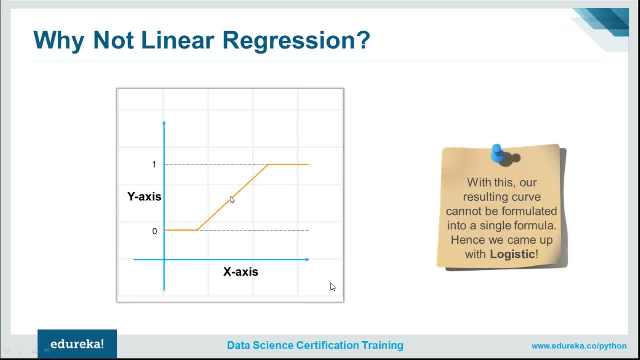 Once it is, it reaches one, it is all this one, so that it lies in between of zero to one And you can set some threshold value as well in between, like you can say: okay, above of this, I can say this is one below of this. 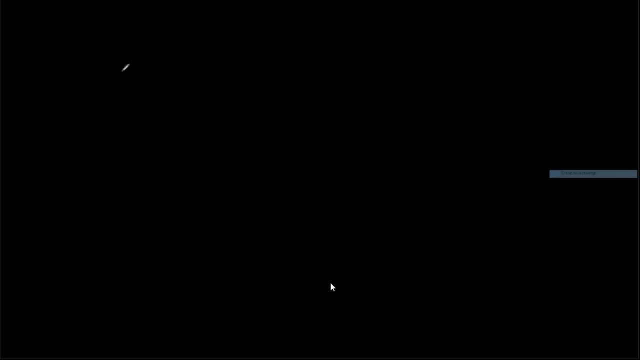 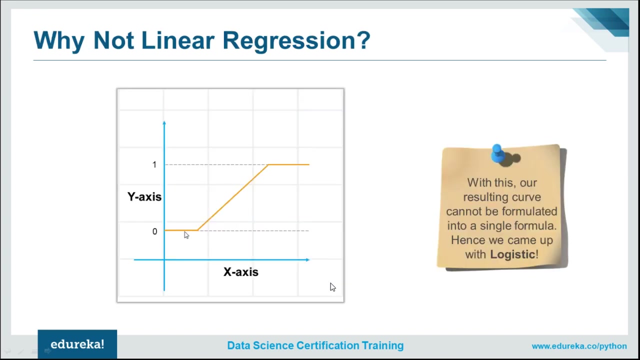 I can say: this is zero, right. So this is what, uh, so what you can do, even with the linear regression. But what is the problem with such technique is that you need to have three curve equation. now, right, One is this: so there are discontinuous curve, we call it. 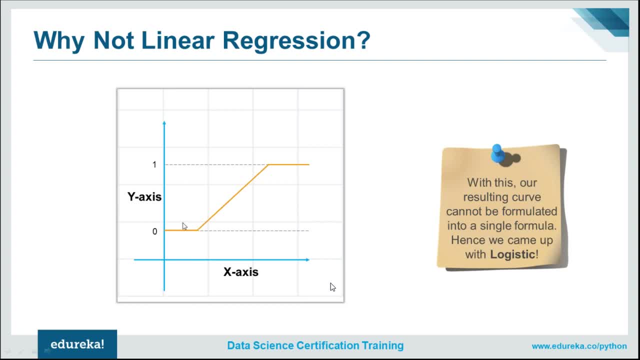 So, in reality, you will leave the curve, But we function to define it. One would be defining this line, Another would be defining this, Another would be defining this right. So this is not a good idea. So what is a good idea? 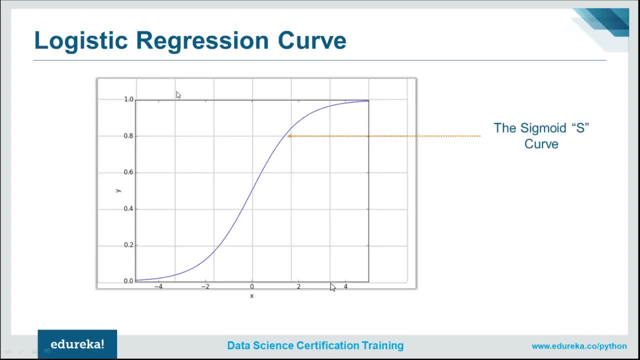 We have a better curve, which you call it the logistic regression curve, or we call it also the sigmoid curve, right? So uh, this sigmoid curve, we this is a kind of having as shape. So what way it has shaped as safe is basically at the bottom line. 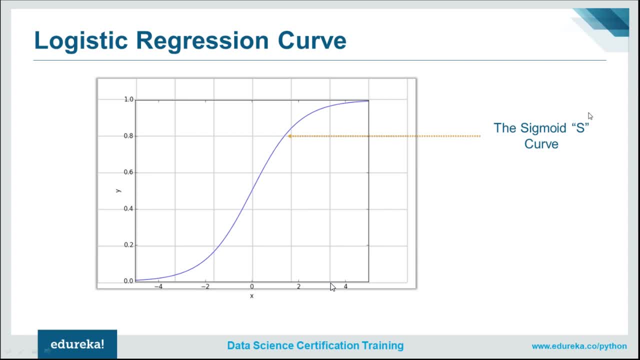 It reaches only to zero and at the top it reaches to one right And it is a kind of as shape. It is a continuous shape actually, right, There is no discontinuity anywhere. Uh, at the bottom it can go only zero, at the top, 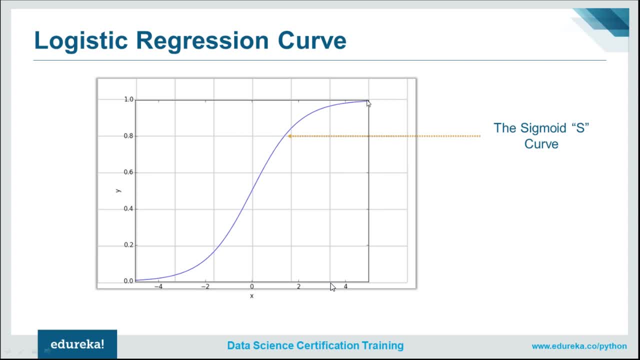 It can go only one right, Beaching one at the infinite here. very slow We leave, it will be reaching one downside Also. it reaches to zero when X becomes around a minus infinite right. Yeah, But you can see very soon it. it is very much close to zero and one right. 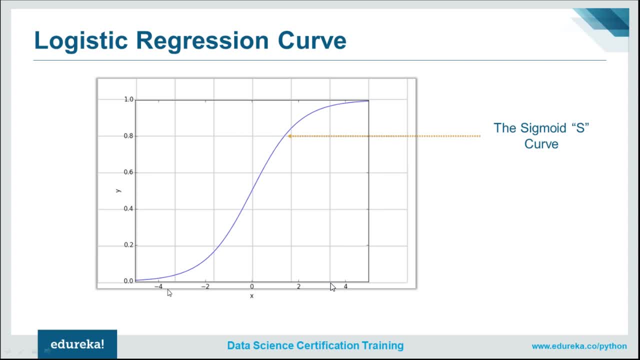 Only that much part you can see. uh, you know that much few values like minus four to four, depending on what equation you're using here. is your uh. you know, having your values uh, which are not uh, zero or one, but the other values you'll be seeing is touching other zero or one completely. 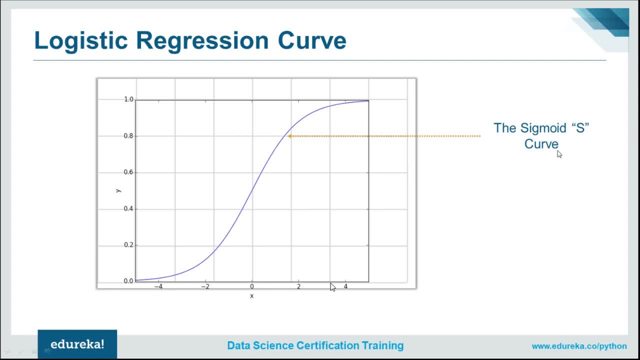 Yeah, So some people are raising hand. If you have doubt also, you guys can ask the question and YouTube people can also ask the question and keep looking, also YouTube chat as well. So if I get some question, I will try to answer that as well. 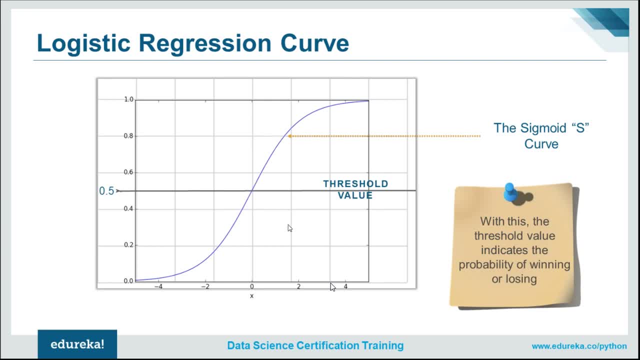 Okay, Right. So now what you will do after taking this curve. you will be having one threshold value in between right And for example, you can say: okay, fine, Five is my threshold. If my value is coming greater than 0.5,, then I will set it as one. 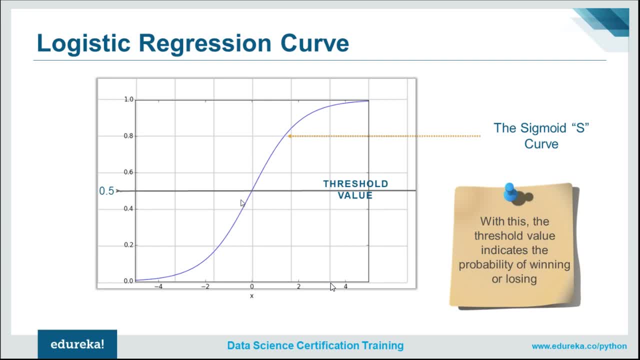 If it's value is coming less than 0.5, I will set it as zero. It can be anything, right. So it might be more than 0.5 or less than Uh, 0.5, right. But you need to finally give your results in terms of zero and one, right. 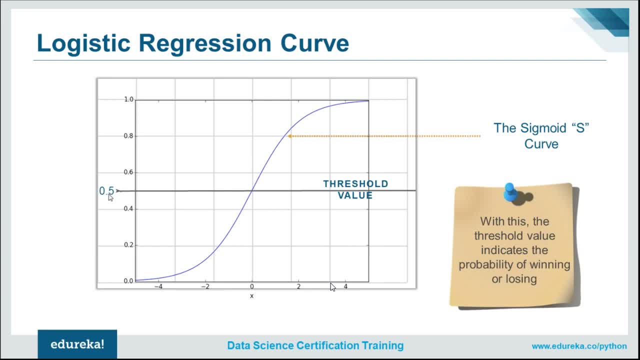 And it's not necessarily that your threshold will always be 0.5.. It can come little downside or it can go a little upside as well, right? Depending on what kind of data right. It might happen that the data points which belong to class one is basically till this place, right? 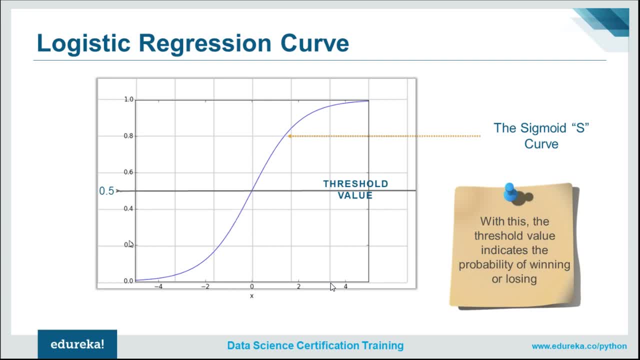 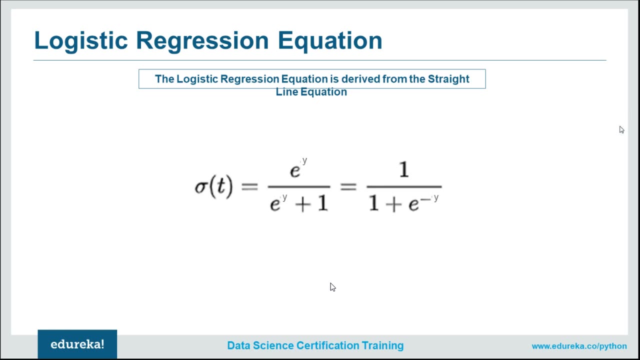 Where X value is minus one. in this case, your threshold will be shifted downside around 0.3,. right, So this way It, uh your threshold can be anything in between zero to one. So what is the logistic regression equation? is this one actually? that is actually here. 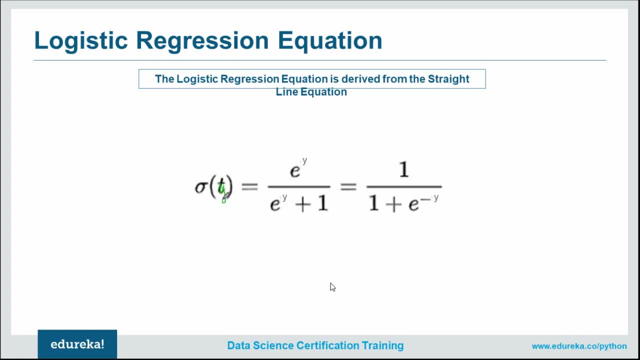 We can write Sigma T, or actually this can be written as a Sigma Y, right? So so here we can write is as a Sigma Y is equal to our E to the power of Y divided by E to the power of Y plus one is equal to one upon one plus E to the power of minus Y. there, 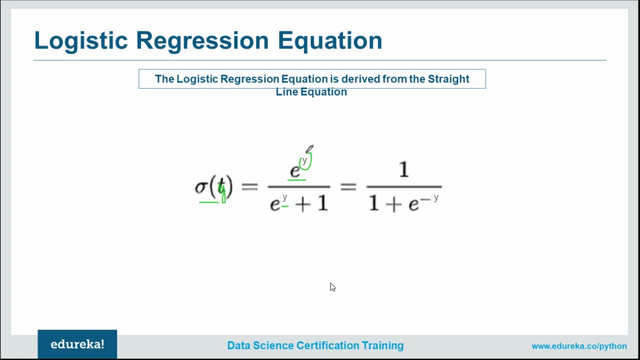 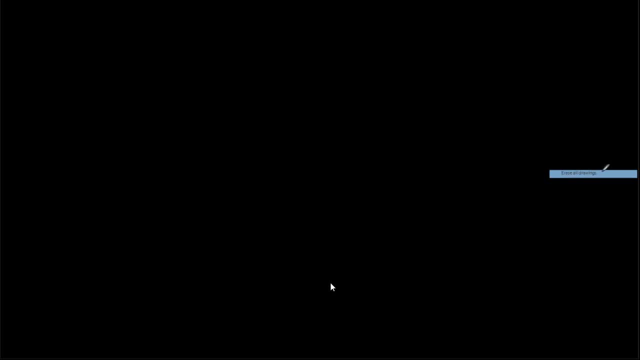 What is this? Y is actually. Y is our linear line equation. only that which we were discussing about in, uh, linear regression, right? So yesterday we discussed in linear regression, right? So you guys might be remembering the Y equation was something, right. 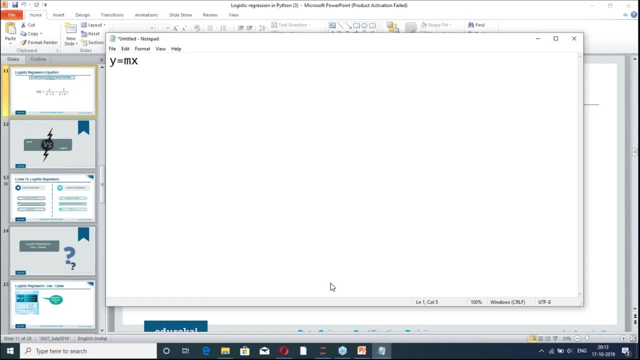 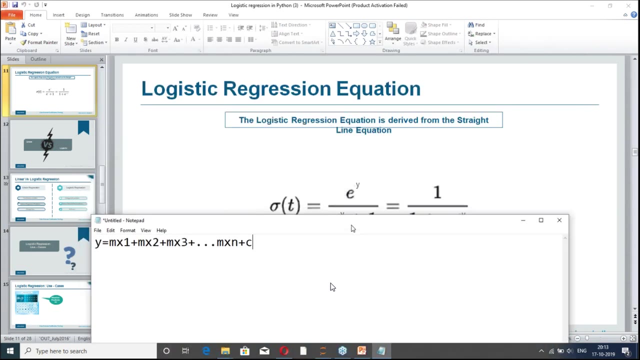 You're writing like: Y is equal to MX, one plus MX, two plus MX, three plus so on, and X and plus C, Right? So this was our Y equation, that is our linear regression equation only. So here in the Y we are coming: the same equation only that is linear regression equation only. 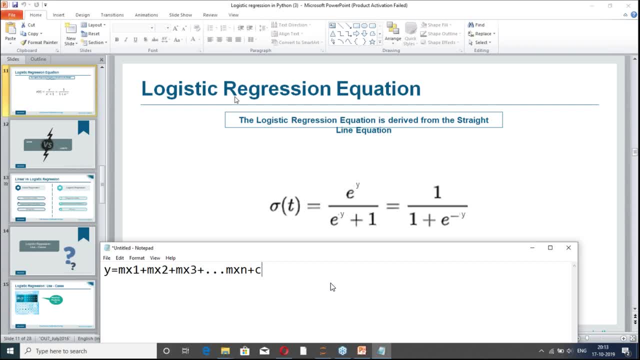 And that is why it is getting the name of regression right. Your question might be: even though this is a classification technique, but it's still. we are calling it as a linear regression right? So why? why are we doing so because of this reason only that this is a regression technique? we are saying, because Y is again the same equation which is coming from the linear regression. 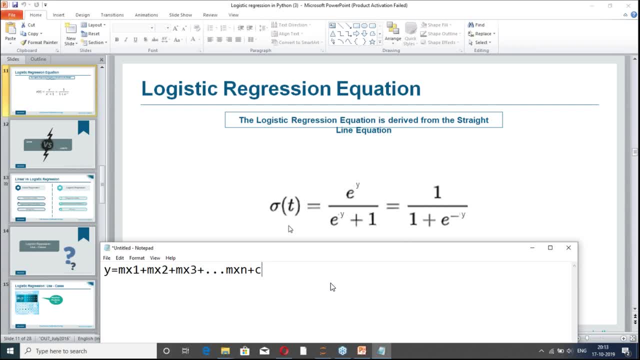 Right, But overall output would be given in terms of zero to one. So let's see now why is okay. So if we see here why, why seems to look like again that Y would be changing from minus infinity to infinity, right? 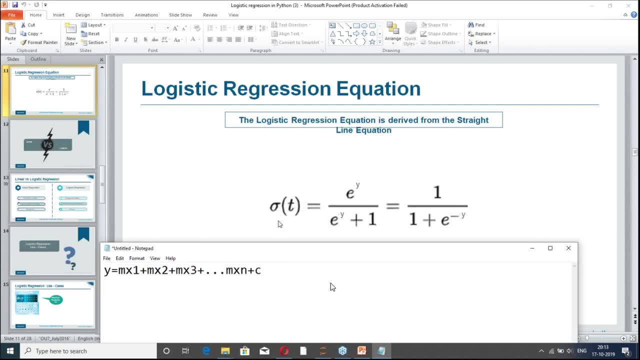 Then how this Sigma T value would be changed from minus one to plus one, right? So that might be sorry. zero two plus one, how it would be changed? So let's see both the extremities here, Right? So let's see both the extremities here. 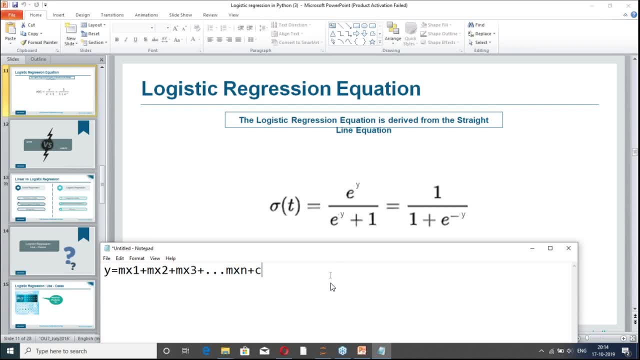 Let's say Y value is equal to. if we take Y value is equal to minus infinity, right? So if we take Y is equal to minus infinity, then what do you be seeing here in this equation If I put one upon one plus E to the power, minus, minus infinity, right? 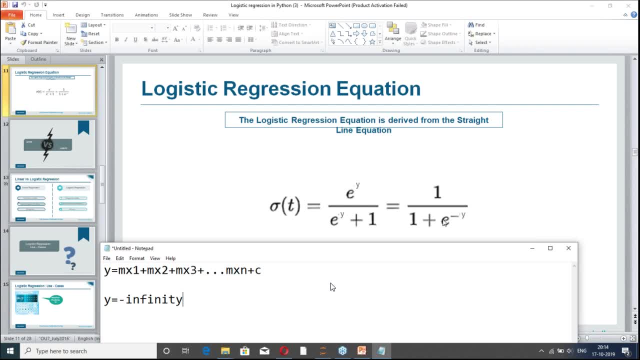 So minus minus become plus right, So it becomes E to the power infinity, and E to the power infinity would be infinity. So it becomes one upon infinity. So one upon infinity will be what. My Zero right, So my Sigma T become what? 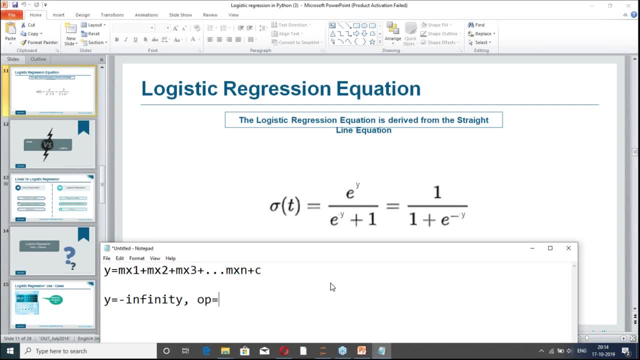 In this case, output would be zero, right? That is when our Y is becoming minus infinity. Then we saw here: this is becoming zero, but let's say Y is becoming plus infinity, right? So if we talk about Y is equal to plus infinity, what would happen in this case? 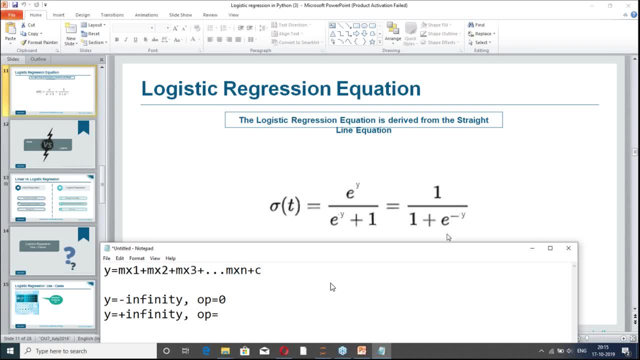 So if you see here, in the same equation now, what we are saying is Y is equal to plus infinity. So it becomes what It becomes: one upon one plus E to the power minus infinity. right, So I will just write here: 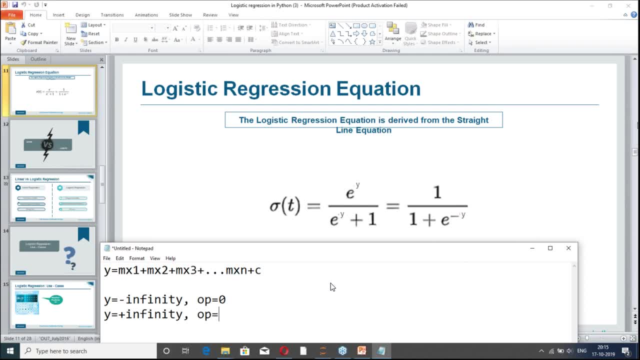 So E to the power minus infinity, So E to the power minus infinity. how you can write, I will just use a little bit of a pen here. So here we will write one plus one upon E to the power infinity. right, That would become our equation, right? 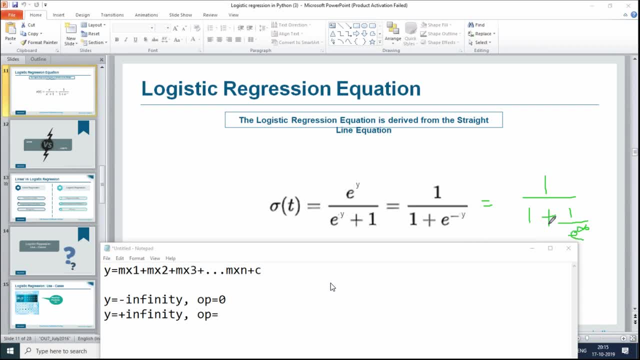 So E to the power of this, because here it is a minus, So I can write it One upon E to the power infinity. And this one upon E to the power infinity becomes what It becomes zero. And then one upon one plus zero becomes one. 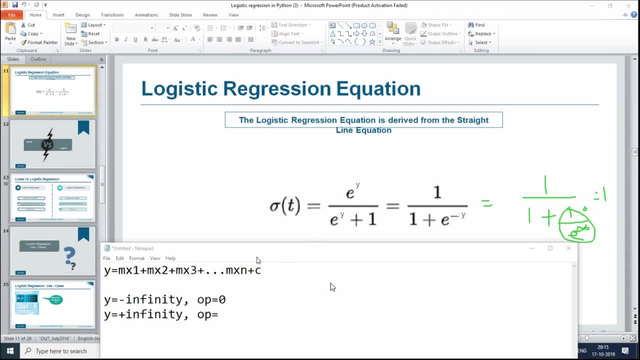 So what you can see here, that, as we are changing the value from minus infinity to infinity of the Y, but it's still our Sigma T, or the output value is changing from zero to one only right. So you can see how this particular equation, which is our logistic regression equation, 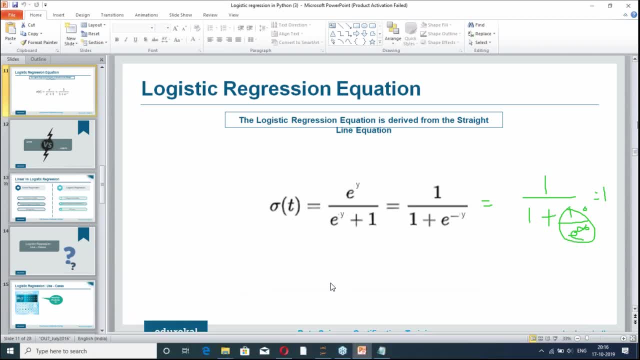 is changing this thing. Okay, So let me see. There seems to be a few questions on the YouTube. Harsha is asking: so does it capture nonlinear pattern as well, as the function uses nonlinear functions. in my function Right, It captures nonlinear pattern. 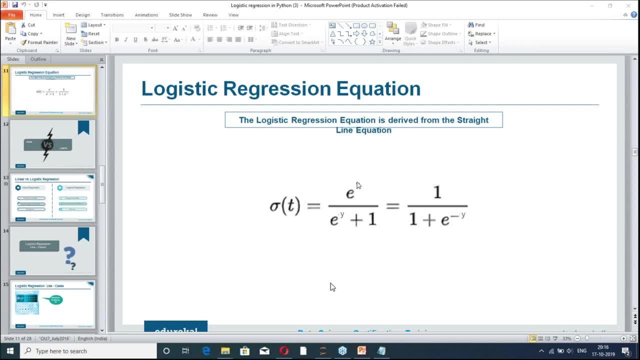 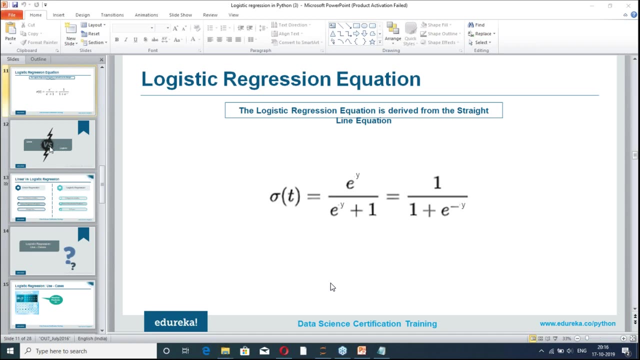 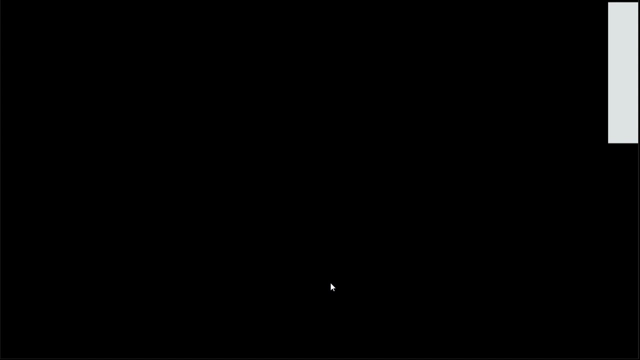 Okay, So yeah, definitely, This is non nonlinear. Overall function is nonlinear only. So, yeah, it is capturing the nonlinear pattern as well, completely Okay. So now let's go to the next slide. Okay Now, linear versus logistic regression. if we discuss 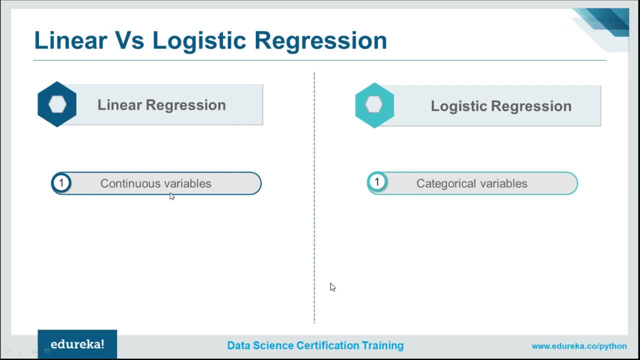 So this is for continuous variables, right? So output variable is our continuous variable only. This is for categorical variables, right? So it's not necessarily that always it has to be a completely categorical variable. Input variables can be continuous as well, right? 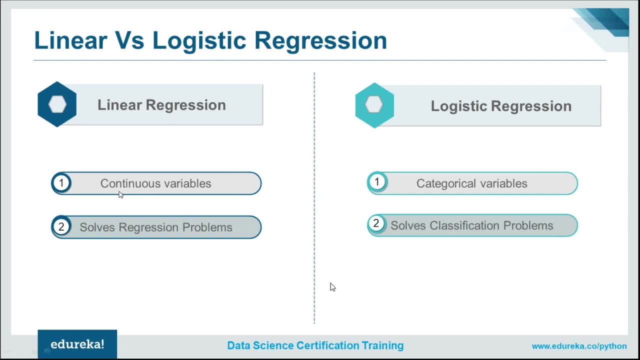 Linear regression It can be. again, output variable can be only continuous, but input variable again can be categorical or continuous. It solves regression problem, while it solves the classification problem, And when we talk about its curve it is a straight curve, Right. 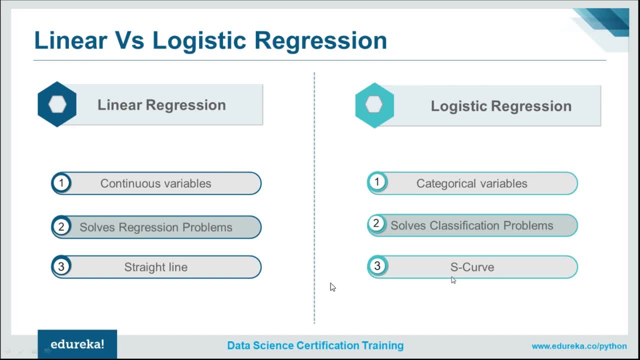 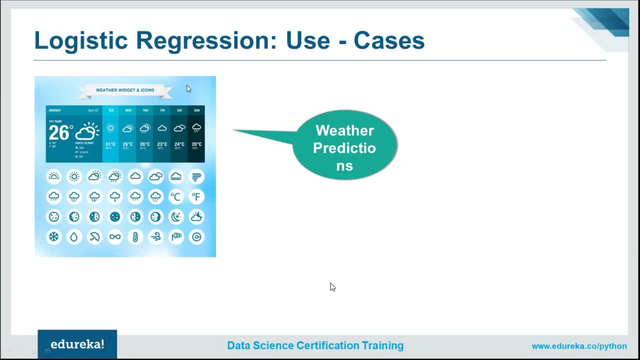 Or linear curve it is, while it is of shape of S curve, Right. So let's see one simple use case here. Let's say so, let's say weather prediction we want to do Right. So so one is, if we talk about simple weather prediction. 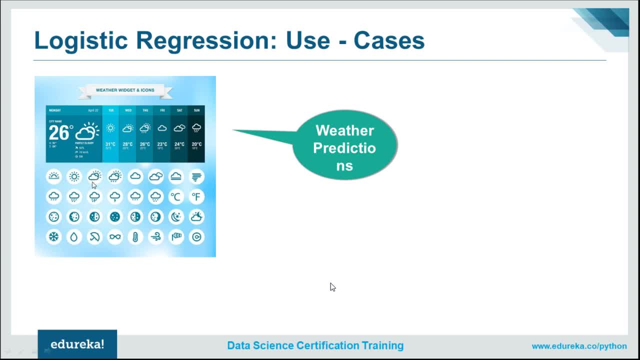 So if we want to do this thing, only weather what would be the temperature of tomorrow? Right, This would be linear regression equation or maybe polynomial regression. It is a regression technique, Right? But if I want to find out whether tomorrow would be a rain or not, 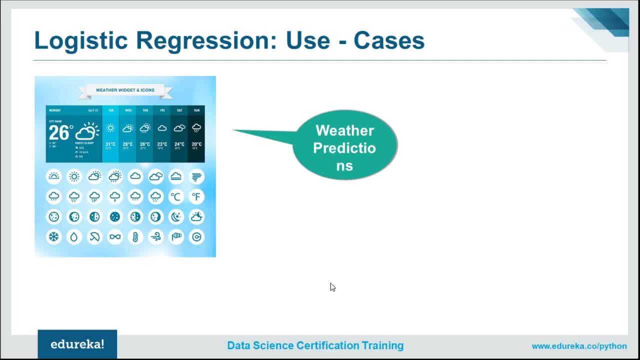 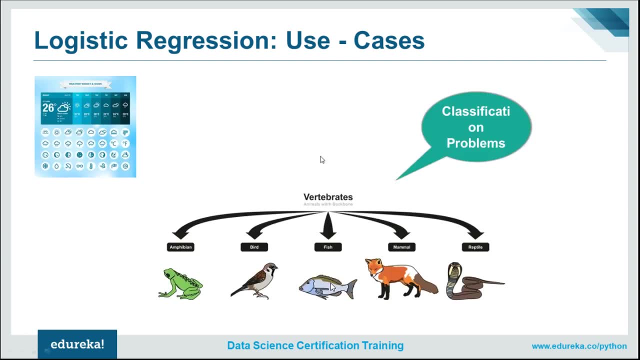 Right. So tomorrow would be rainy day or not. So this would become a logistic regression case, because here we have the two output classes, only Right, And similarly maybe, if our cases might be some time, maybe more than one classes we want to do. 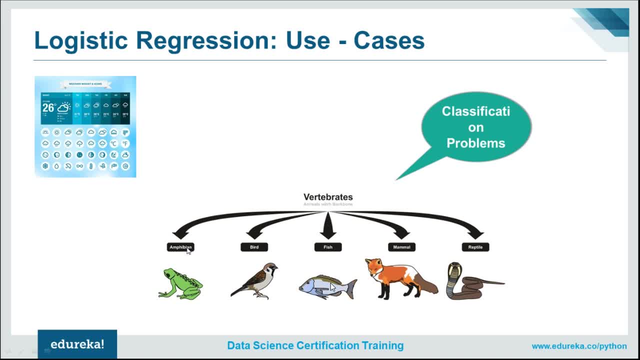 So, for example, let's say the images are given and we need to predict whether it's an amphibian, bird, fish, mammal or reptile. So here we want. we might be interested in doing this classification, or it might be. 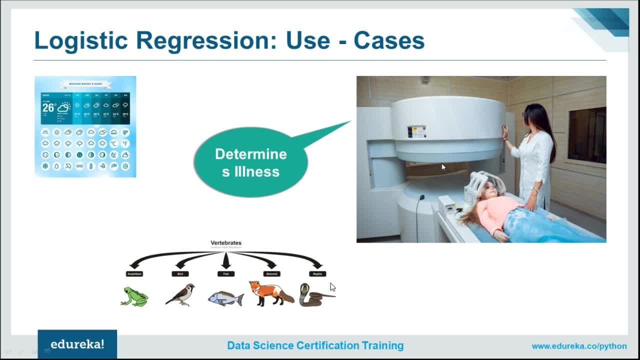 let's say, a patient is going to, you've got a patient report and by looking patient report, this is a simple patient report which is telling about blood pressure and some other such kind of values only reports, only hemoglobin, blood pressure and these kind of things. 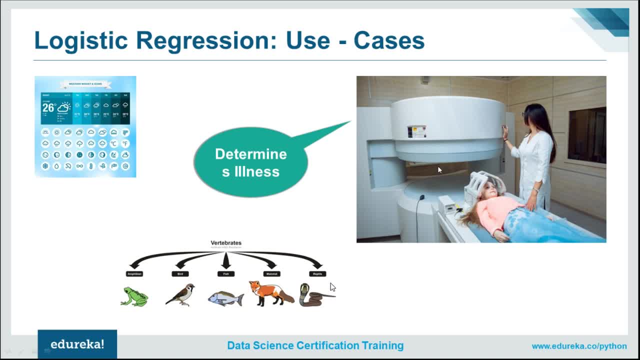 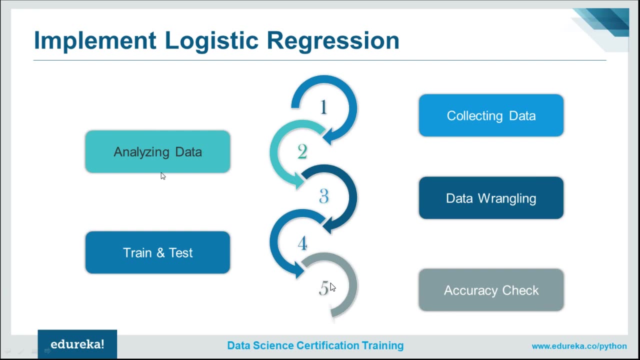 And you need to predict whether a person might have, let's say, this particular illness or not, Right? So this becomes again a logistic regression case. So we are going to see a demo, So let's see exactly how we can do the apply the logistic regression. 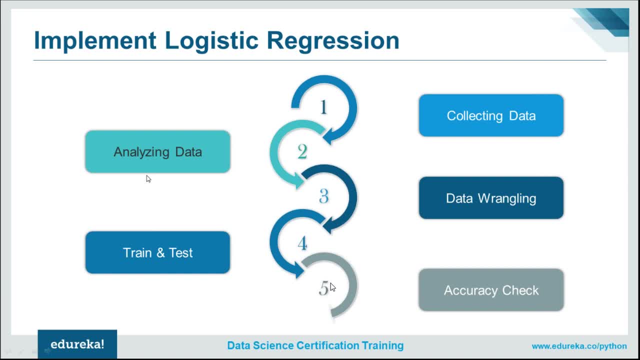 So initially we will see very simple way. So normally what we do, we need to collect first of all data, right, So we need a way to collect the data. Once we get the data, then what we need to do: we need to analyze the data. 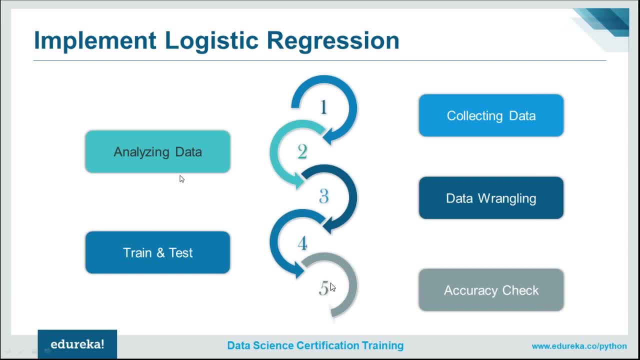 We look into it, We see what can be changed. What are the issues with our data? Noisy values are there or what? And once we get that, then we manipulate the data. right, That is our data. We manipulate the data. 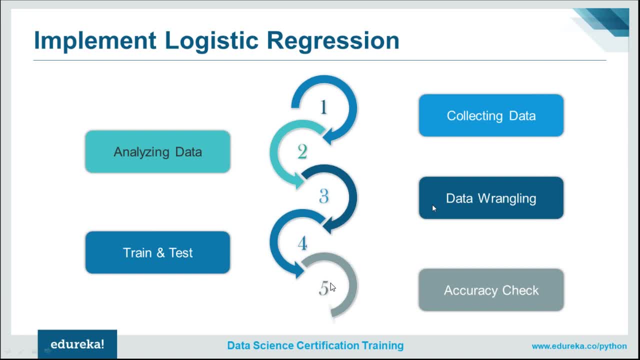 We find out if there is a. whatever issues were there like noisy value was there, outliers were there or some missing when he was there. we need to handle all those things in doing the data And then staff, And after that we divided our data set into two parts. 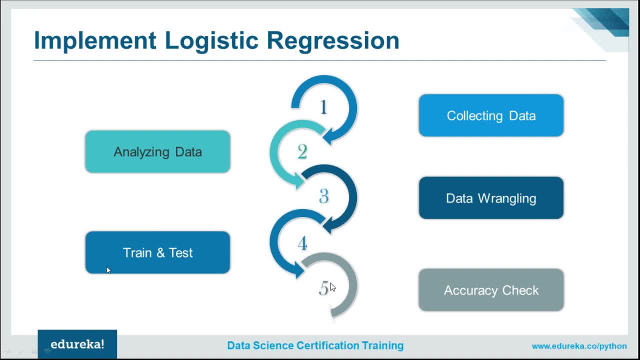 One is training and testing set as yesterday also we saw right. So training first of all. when we do the training, It will be. it is equivalent that I took a one analogy yesterday. the same analogy, just quickly We can take that. 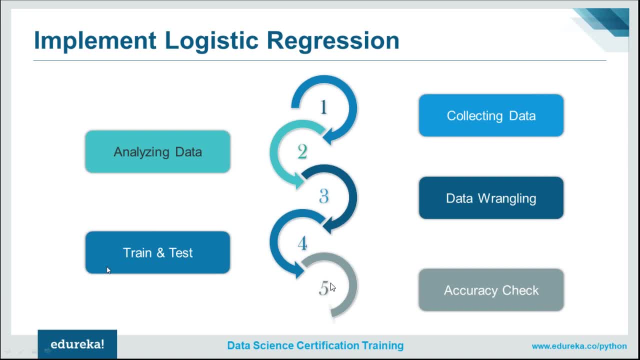 Let's say, if I have a book in which a hundred questions are there, I want to teach you And then I want to test you also how you're working. So what I will do, I will take 70 questions out of those a hundred questions, with the 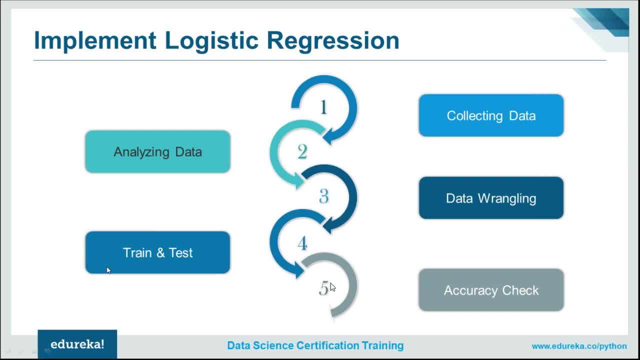 solution And I show you those 70 questions as well as the solution to you and the rest 30 questions I will give you as a test and keep the solution with me. I do not show it to you And when you give the solution for them, then I check the solution which I have, which. 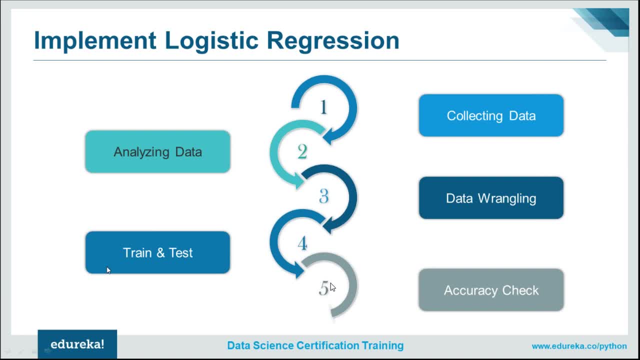 I kept with myself, And then I see exactly how good you are working in the past, right, And the better you work. that is your accuracy check. only we'll be finding exact what is the accuracy that you are getting. So they are just showing one simple case. 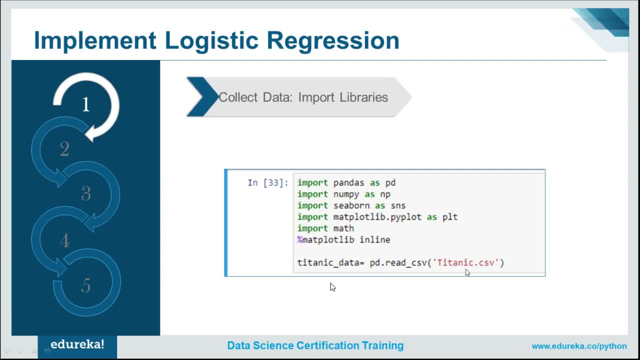 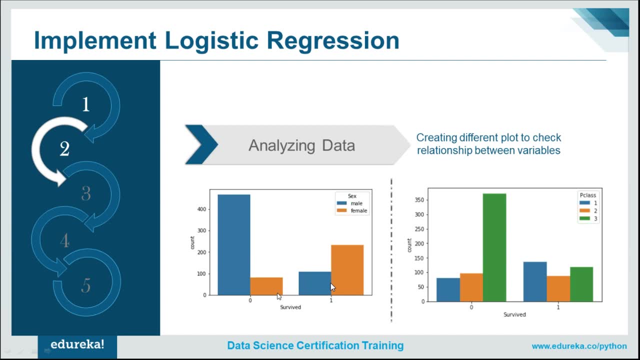 Let's say it was a Titanic data set, which is which is, let's say, stored into this file- titaniccsv file- And And then they analyze the data. They look exactly, uh, let's say, in this titanic data set it was having how much people survived. 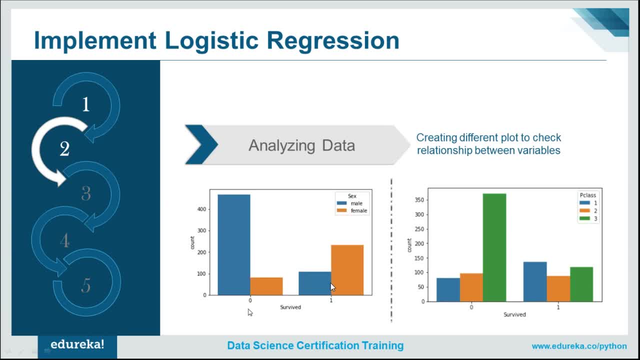 and all. So let's say: zero is saying for uh, not survive. One is saying for survival and a blue curve blue bar is showing the male and this orange bar is showing the females. So you can analyze the data Okay. 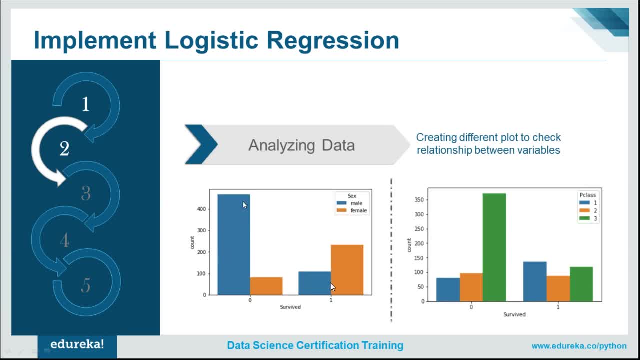 This is my how many meals, uh types where you can see a lot of male died actually and compared to females, right, So very few females died And if you see how many people survived and you see it's completely opposite: very few. 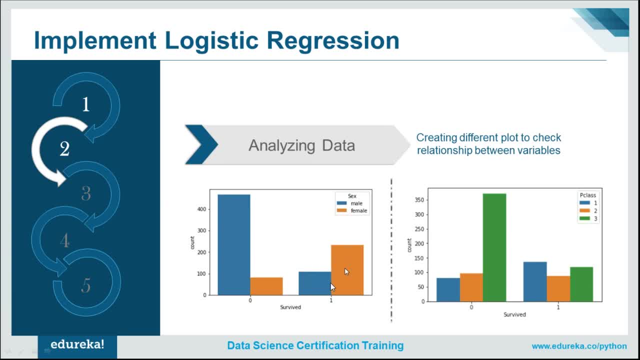 males survived by the. lots of females survived right. So this way you guys can look here and similarly, so you can do it on the basis of sex or you can do it on the basis of the class. Let's say this is a class in which particular class a person was craving right. 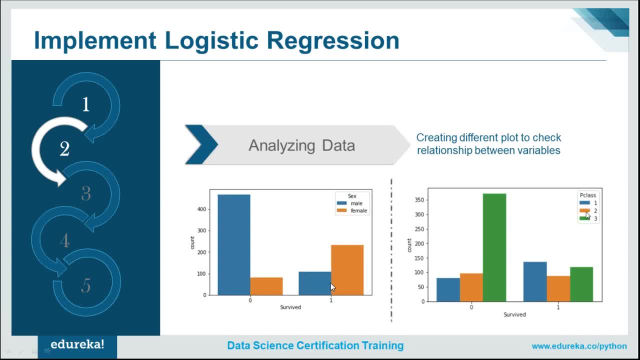 So the person might be trading it First class ticket. We are on the second class. All right, So you can see, the person who died mostly belong to the third class. Okay, Right, So this is. you can see. this is a bigger bar rate, showing that most of the people who died 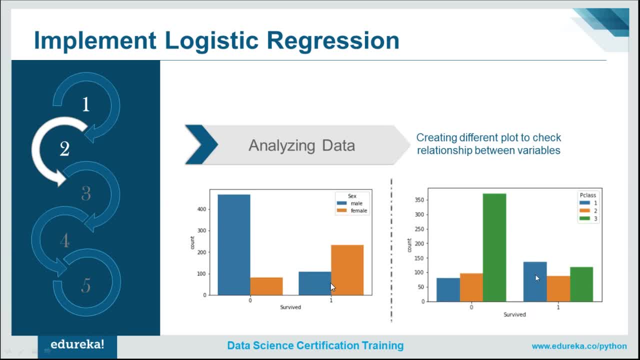 were belonging to the third class only, And while if you look at the survival rate, you can see most of the people who survived was belonging to the blue class, That is, the first class people, right? Yeah, You might remember from the movie, they were giving more preferences to the people who? 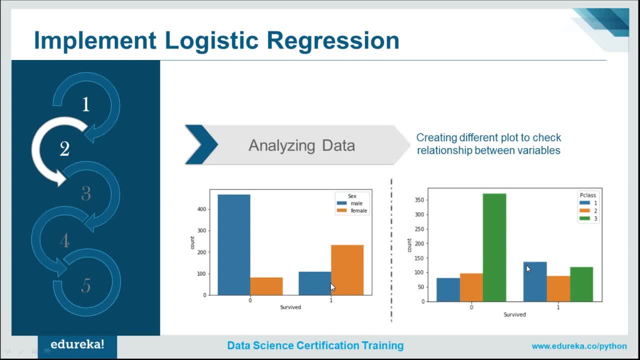 were in the upper or higher classes, Right? Not, they were taking, they were not taking care of the people who belong to lower classes. So this way you, let's say you, analyze your data. this is just a you know example, for 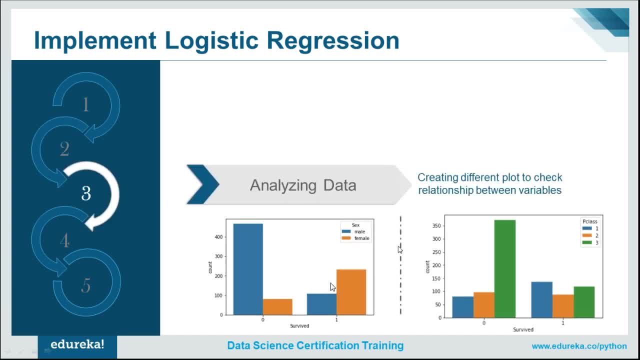 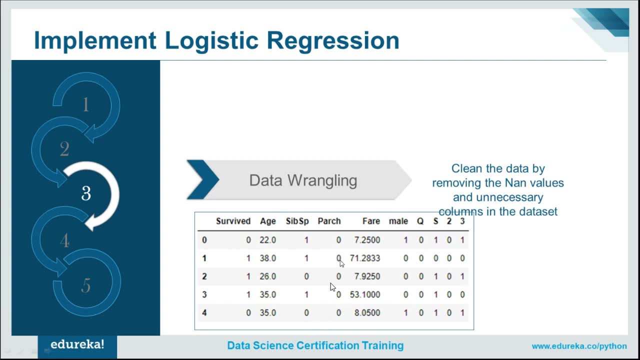 showing what are the steps you might need to do. Okay, And then you do data angling. doing data angling, Let's say there were some- uh, none values were there or missing values were there. Then you remove those missing values. 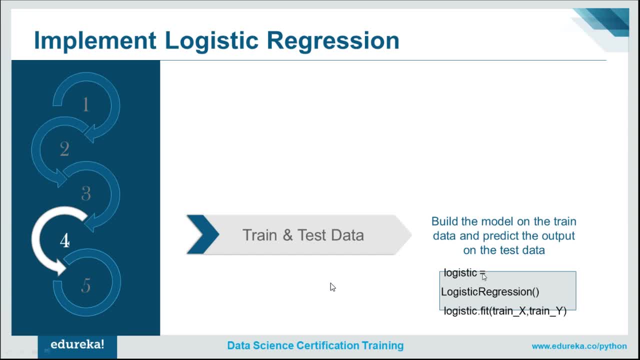 Right, And after that you do the training. So how do we do the training? We call this particular class, we create the object of logistic regression class object which we, let's say, calling as a logistic, and we call the fit function logisticfit. 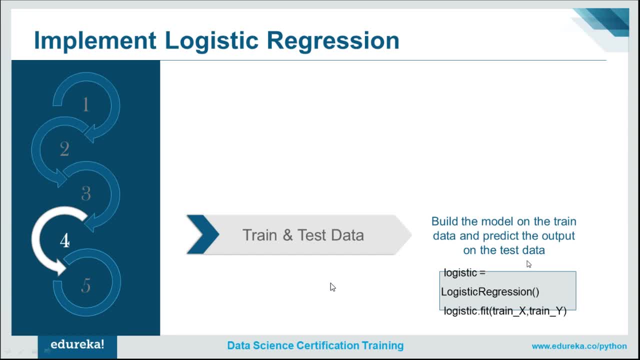 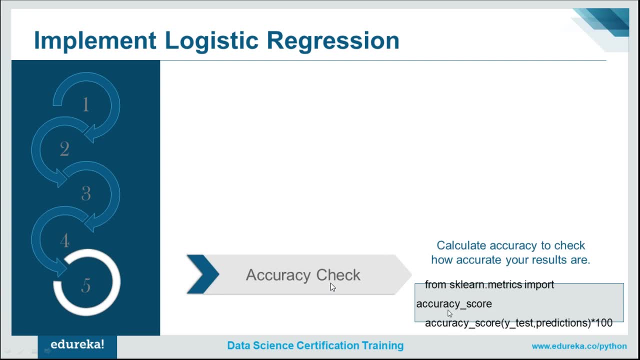 and we pass the train x from our train by right And then you do the normally accuracy check from this particular model, which is a skill and dot matrix. We import this function, which is accuracy score, And within this we pass that. 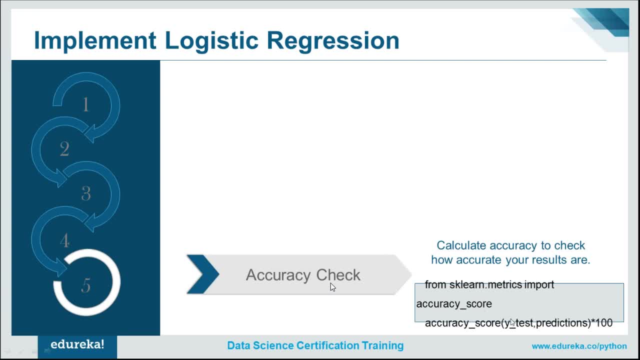 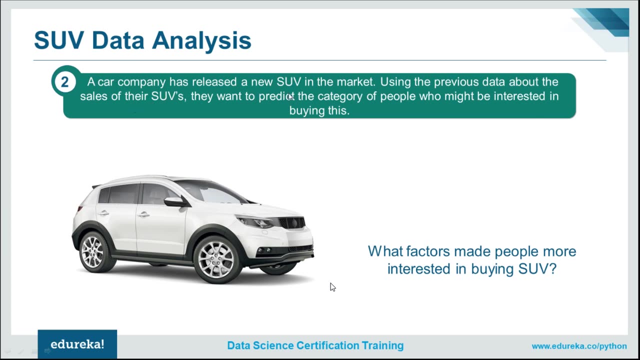 We pass the predicted output, predicted by our system, and what is the correct output, and that we remove accuracy check. Now we are going to see one particular case ourselves and you will take the data set of a SUV data analysis. A car company has released a new SUV in the market. 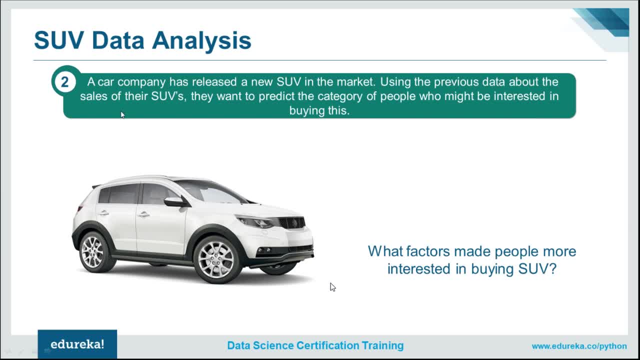 And, using the previous data about the sales of their SUVs, they want to predict the category of people who might be interested in buying this right. Okay, So this is what we are going to do now. So let's see, We will predict who might buy, and all right. 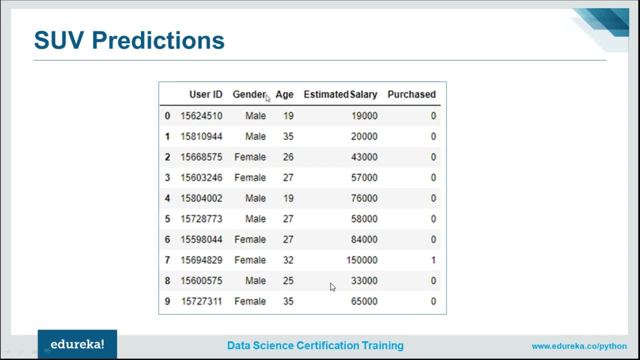 So let's say this is our data set is given. let's say this is a user ID, this is a gender, like male and female. age of the people are given, like 19,, 35 and so on, And what are their estimated salaries and whether they purchase the car or not. 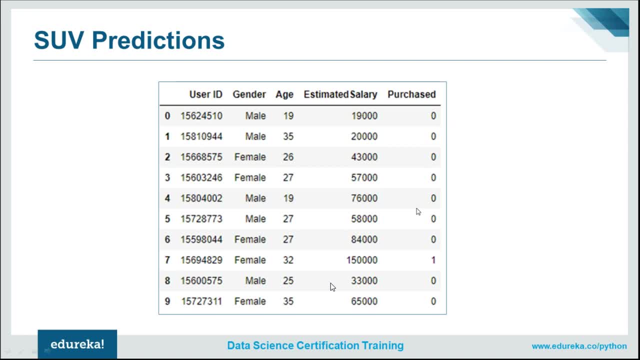 So let's say this is our data set, Let's say this is a user ID. This is a gender, like male and female Right. So this is a past data so that you can think which kind of people may buy the car right. 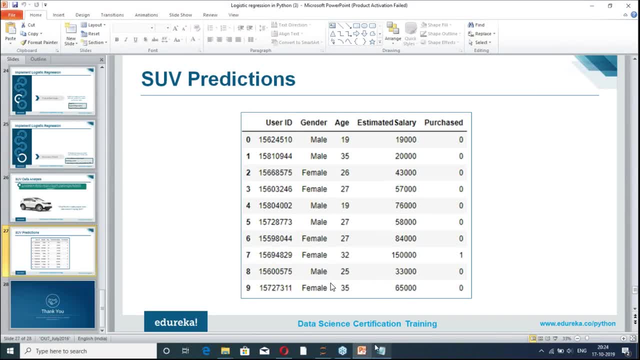 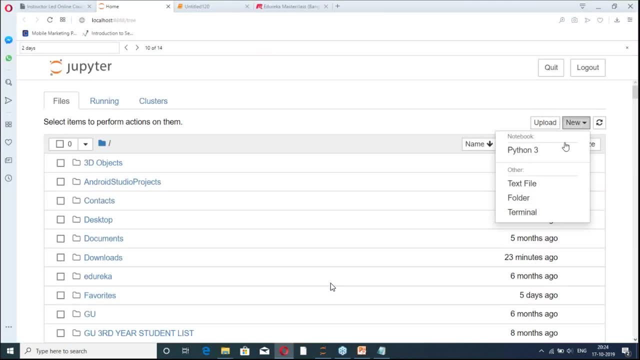 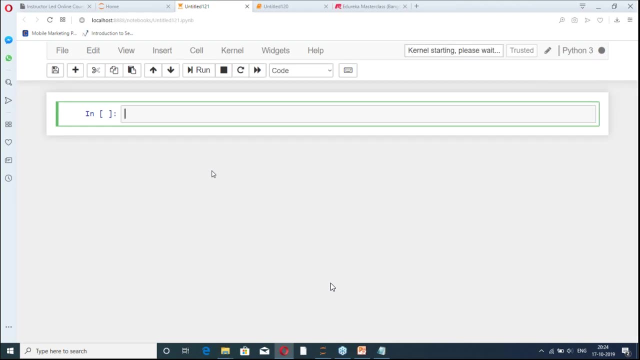 So we will be doing this down and we have little bit more time actually today, So what we will be doing, I will be taking you through some of these steps right. So, like some of you were. so what is the normal way you work with the SK? learn right. 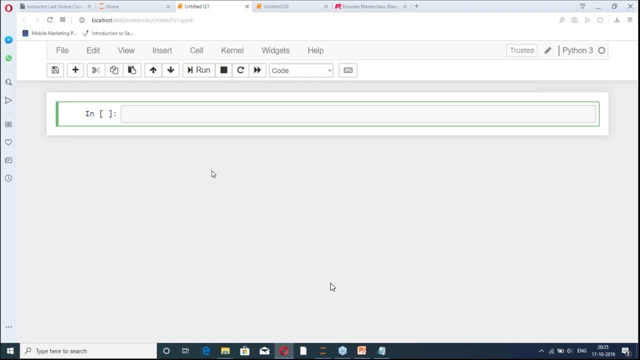 So I will be telling you the normal pattern of that, The normal flow for implementing any algorithm of machine learning. most of the algorithm would be implemented in a normal flow. So let's see what this flow we are going to have. So I will just write here: we will not execute code here first, and later on we will execute. 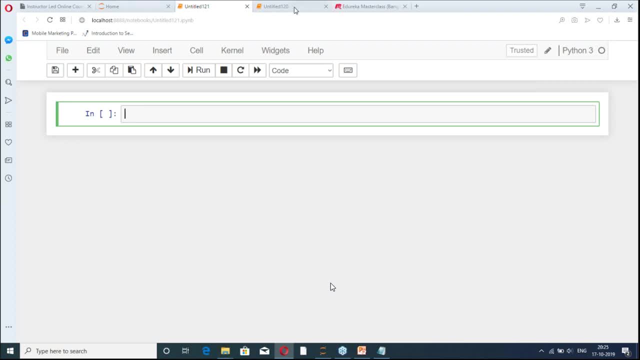 the code with the SUV data set. Okay. So I hope here I have read the data set Okay. So, first of all, what do we do? What are the steps? So I am taking you steps for implementing any MLL code using SK. learn right. 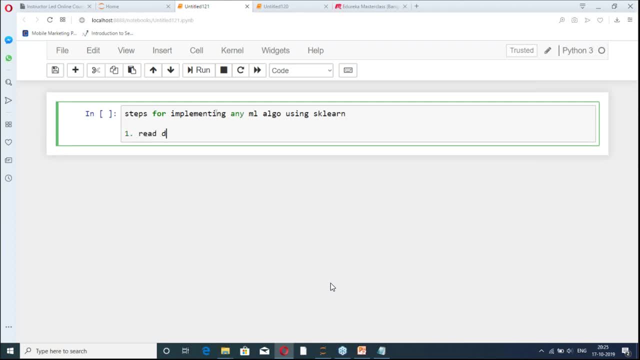 So the first step which you need to do is to read data set. and how do we read the data set? We write in code- mostly it would be pandas as PD- and then in some data frame we read it. So if I write pd, dot, read on this course CSV, and here we write the file address, file name. 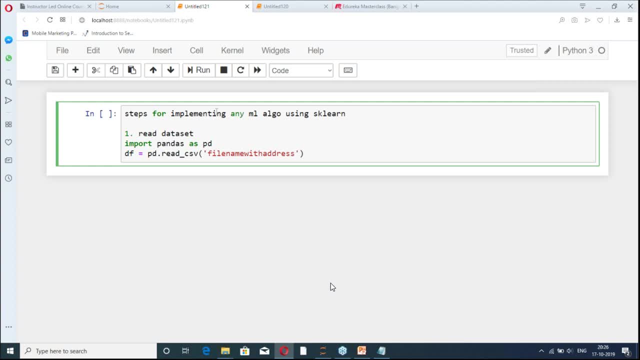 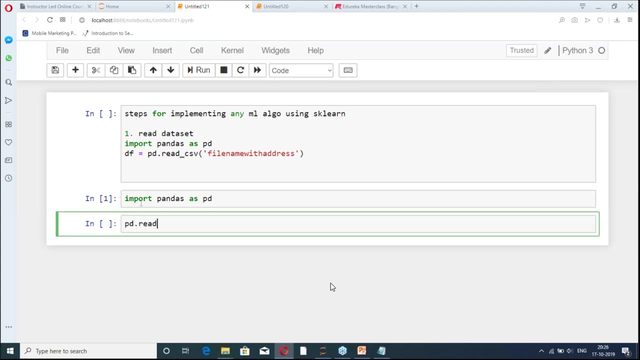 with the address, right. So this way our data set is right. right, So I will be. I will be showing you something as well. So, normally, what is this library? If I write here in port pandas as PD, and if I write pd dot read underscore, and if I press? 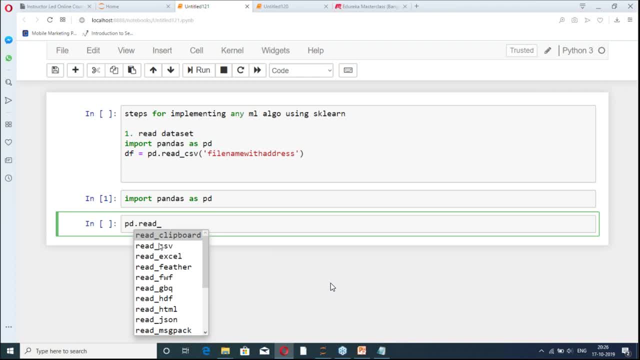 here tab, then you can see the whole list. So you can read from the field board, you can read from the CSV, you can read from the Excel sheet and lots of other databases, You can read SQL and tables and lots of other things, right. 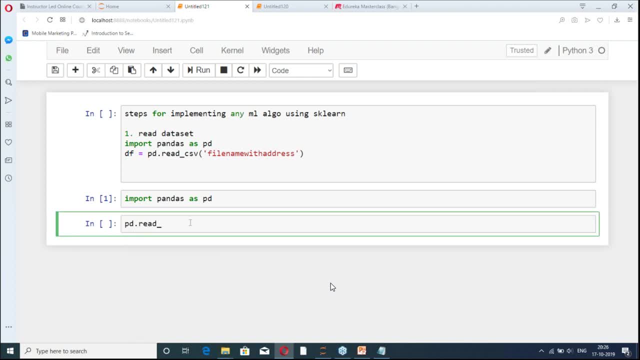 So there are lots of file formatted tech and it can read it for you in the table form, right, Provided it is a readable in a table form. Okay, So let's see here. So this is how we read the file. Once file is read, then what we do. basically, we have few steps right. 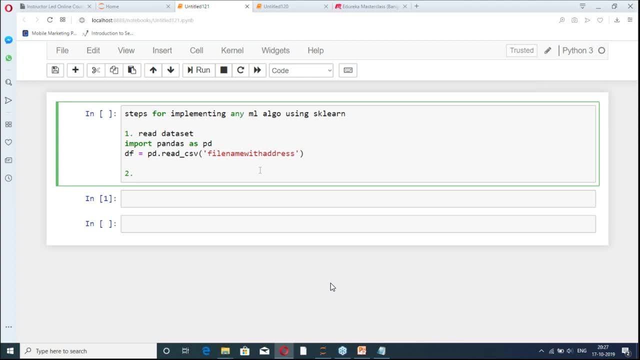 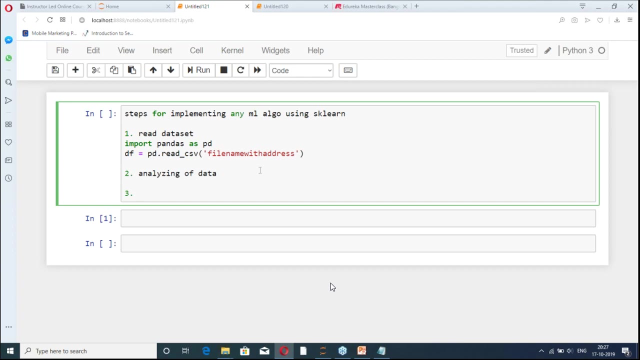 So we basically analyze the data right. So we do analyzing of data, So normally like printing, looking what are the issues might be there and all right. So this is I'm just leaving as such correctly. Let's say, you read the data, you analyze the data and you angle the data right. 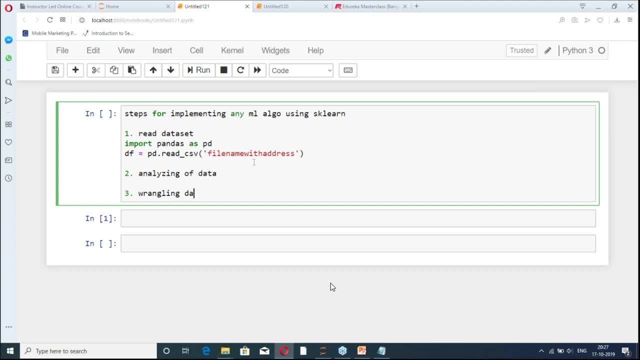 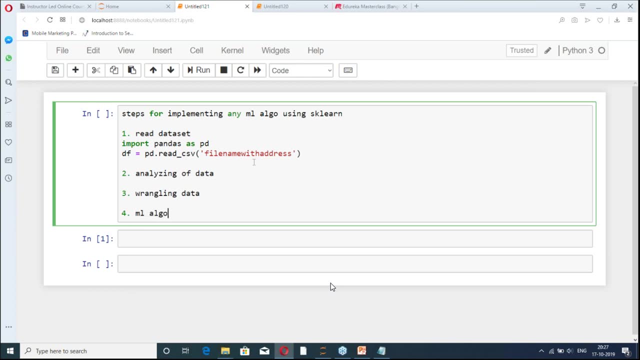 So analyzing Right, So you're angling the data you did. So these are like I'm just leaving. then you want to apply the MLL. So how do you apply the MLL Right? So first of all, you need to divide your data set. 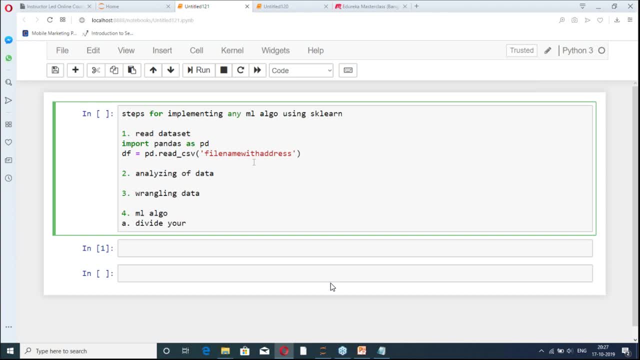 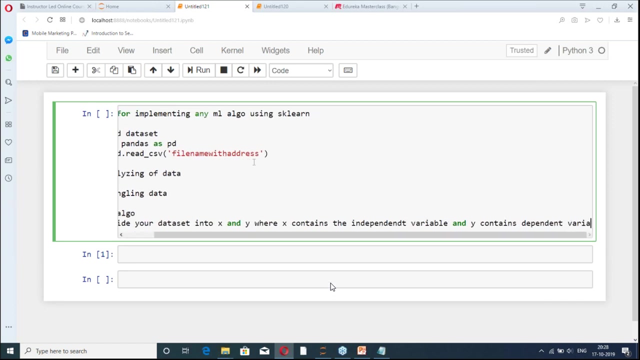 So I will write here a part: divide your data set into X and Y, where X contains the independent variable. Maybe spelling wrong, I'm not taking care about it. in the contains the independent variable and Y contains the dependent variable right. Or we can say output variable dependent or output variable right. 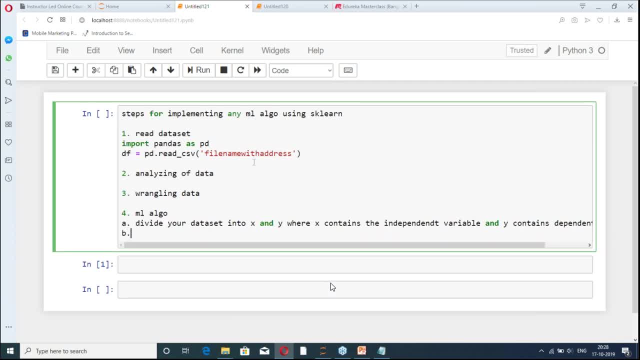 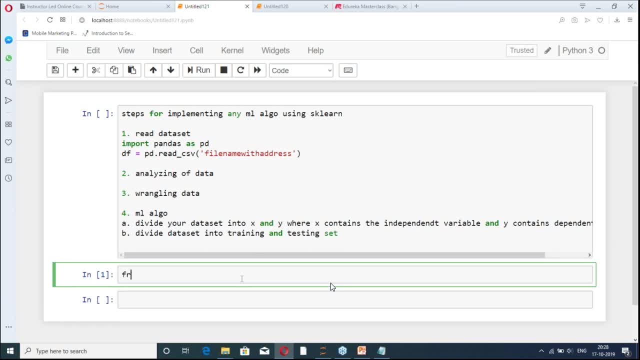 So how do we do that? So we have so normal pattern of the SQL and library is you will write from a skill and dog family, Right? So you like family name. then import class or function, right, Whatever the class of function you want to import. 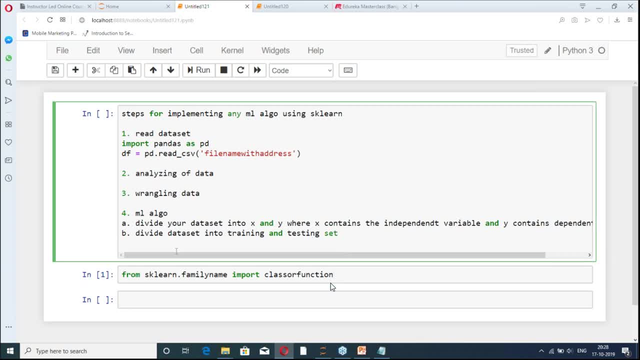 You import that right. So like, for example, if I want to uh divide the data set into the training and testing for that, I will import from a skill and the family name- here is model selection right and from this thing I will import. 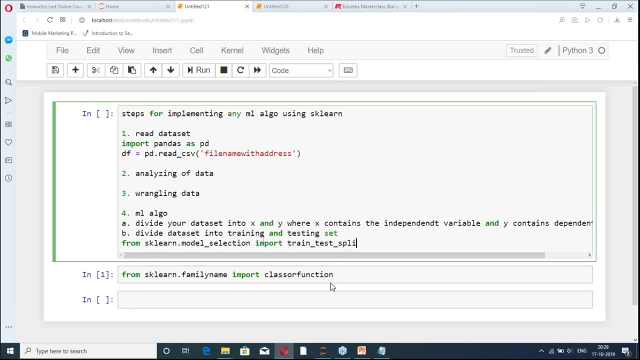 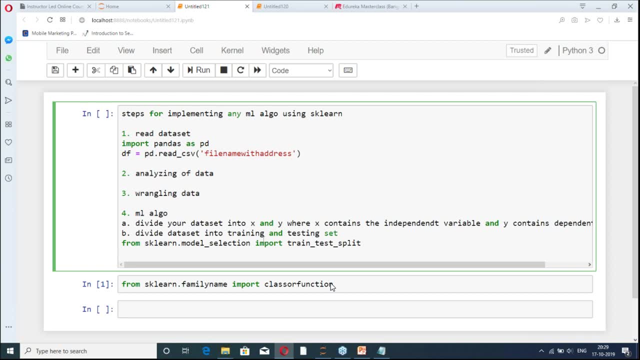 train test is clicked right. so this is the function, as you guys might remembering from yesterday class- for dividing the data set into training and testing set. okay, so, after this, once, once you, once you import this function, this is the function, right, then we will divide our data set into training and. 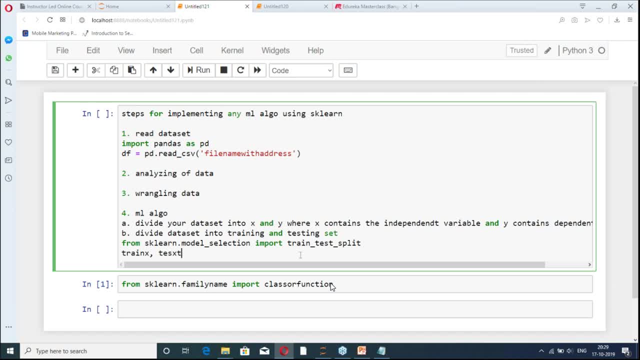 testing set. so what we do? train X, we write test X. we have trained Y, we write test Y, right? so these four values would be written and then we call this function which is trained. test is split, right? so initially I am showing you here normal steps which you can implement with any particular programming, any. 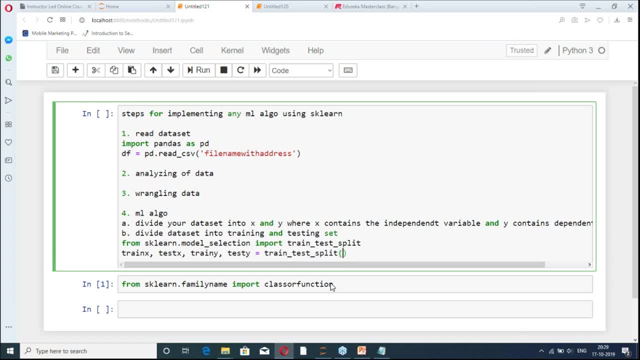 particular machine learning algorithm, right? so these are the you can implement with any particular programming, any particular machine learning algorithm, right? so these are the general steps. then you write here X. then you write here Y. then you write here test size: right, like how much percentage of the test data set you want to testing. 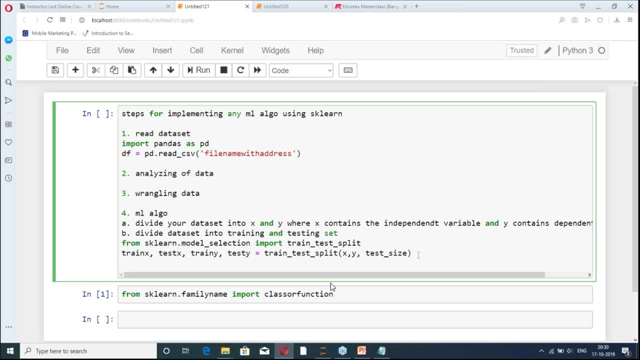 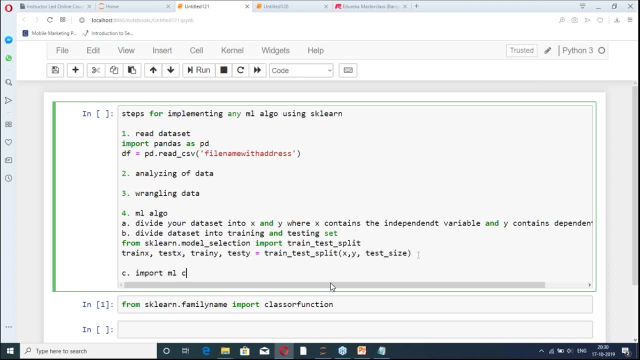 set right might be like 30%, 40% or whatever. once you do this thing, then what you will do next step: you will import ml class right, ml algo class, whichever it is, and again it will be following this pattern from a skill and or family name. import your class, so let's say so, what we write. 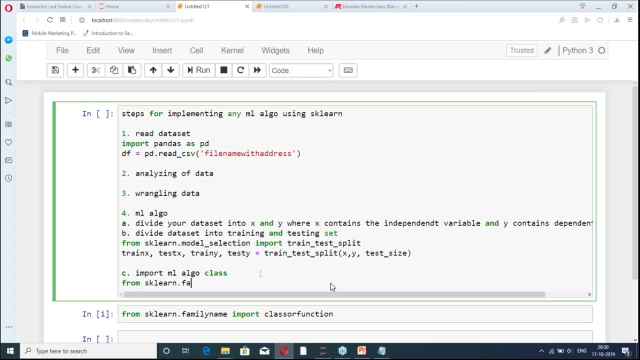 from a skill and or family name. so depending on which particular I'll go Vita, like yesterday we did linear regression. we write linear model here right, and then we import- I'll go class right, ml class. then we create the object, create object of ml, class ml and go class right. so how do we create it? we 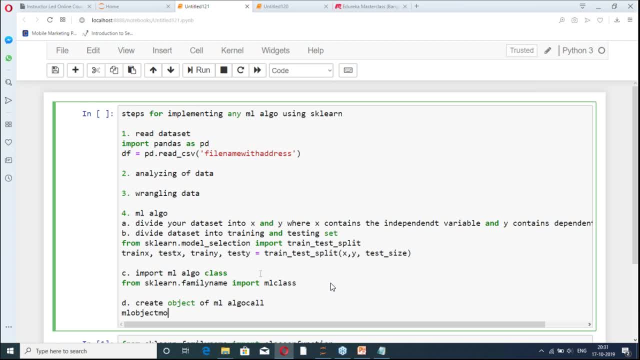 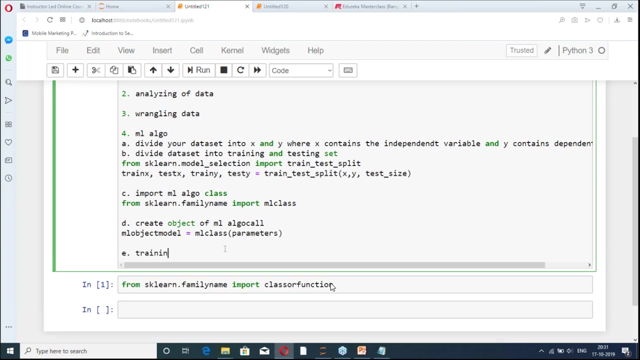 create, let's say, ml object or model. we can write also and we call here ml class, right, sometimes there might be some parameters which you need to pass. in many cases you won't need in many cases. in some cases you need to pass a parameter which you will be seeing. right after that. what is the next step? training the. 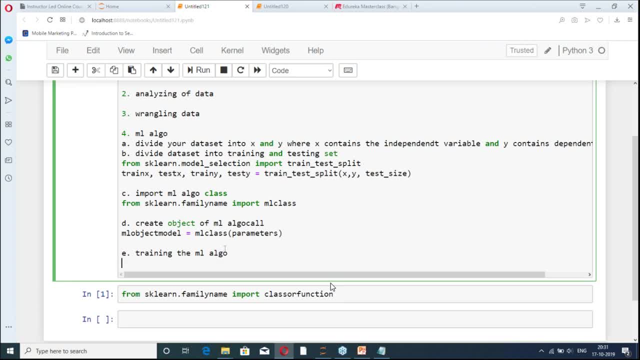 MLL code. how do we train it? we write here our whatever object we created here, right, so this is object we created. so we write here this object name. we call the function dot fit. fit function is saying basically train the algorithm. so how does it train the algorithm? here it will. 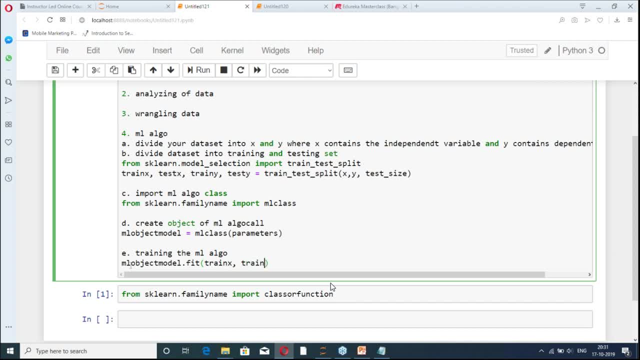 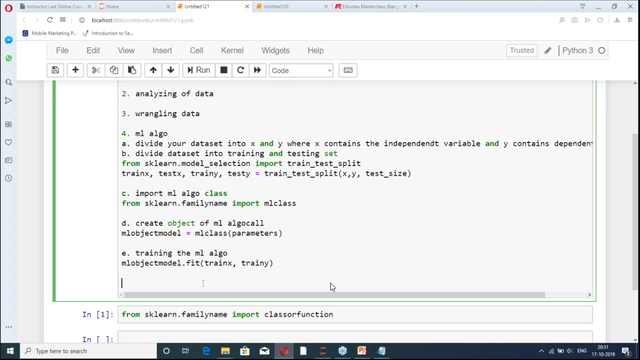 pass the train X and train by right. so basically you are giving the question as well as their solution. so once it get the solution in solution, then you predict out right. so how do you predict for the test cases? actually predict for the test cases? so how do we do the prediction? ML object dot predict is the 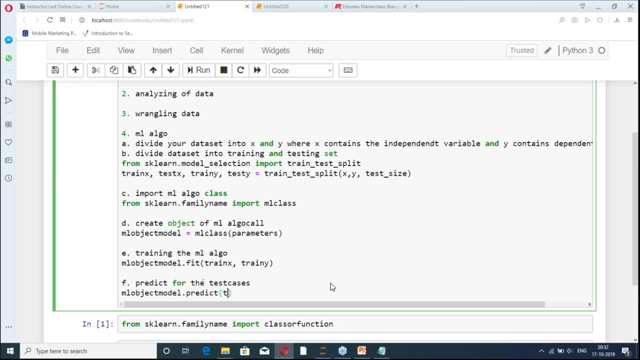 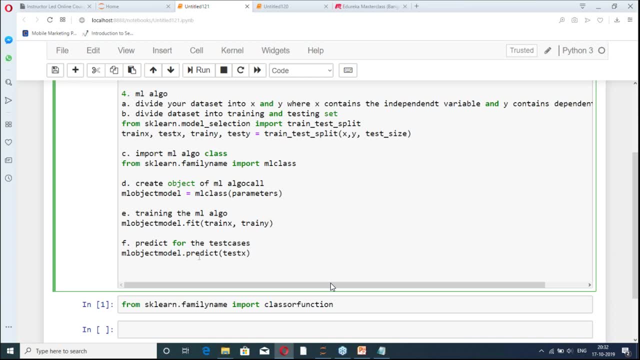 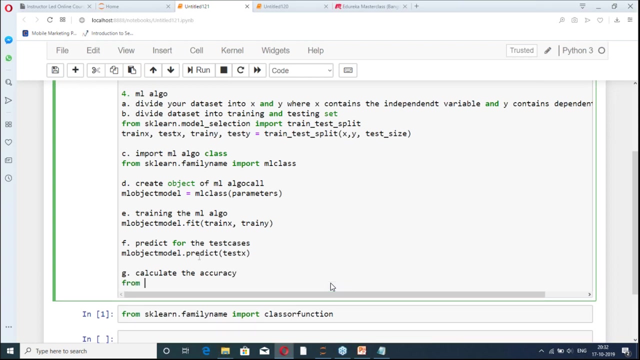 function which we use this, and here we pass the test X right, and after doing this thing we want to look the accuracy right. so the next step here for the ML algorithm is accuracy. so what do we do? we will. for that again, we need to import from SK. 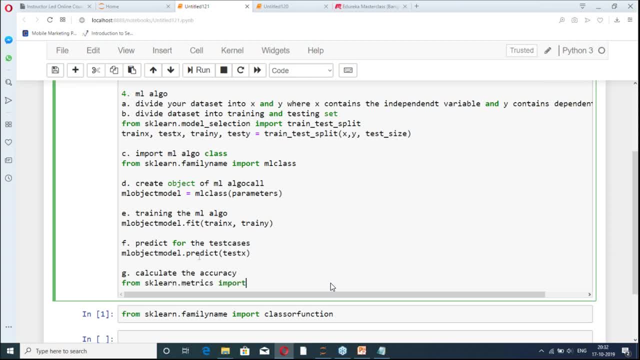 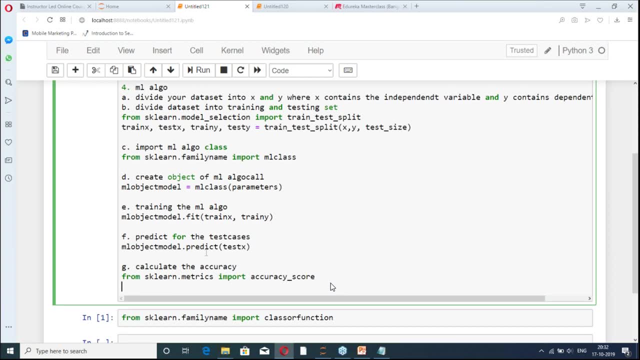 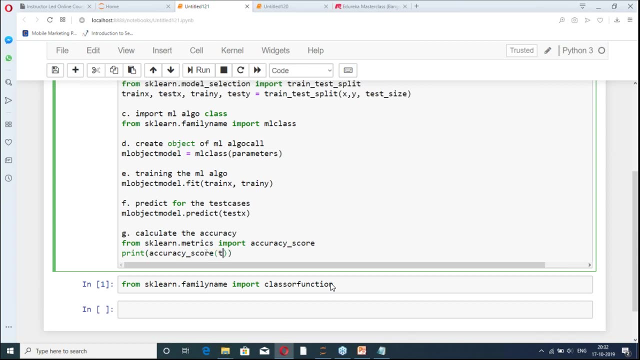 learn dot matrix. there are many different measures are there, so one of them- major- is accuracy score, right, so we call this function like we say: print accuracy score and we pass here word test X. sorry, predicted out output. we didn't store it actually somewhere. we need to store it predicted. 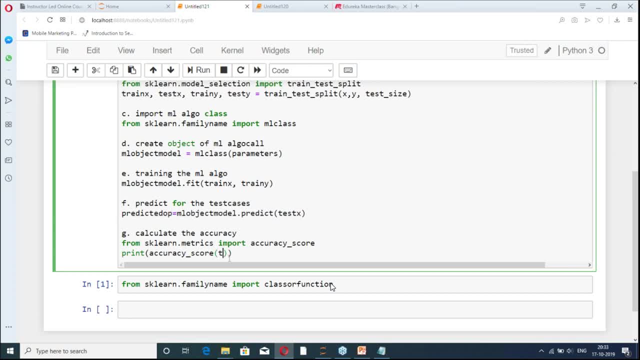 op, let's say, is our variable name. so here we say: what is the predicted op that we are predicting and what is the correct output that is in the test file. so it will give us the accuracy right, and once it is done then we know our model is. 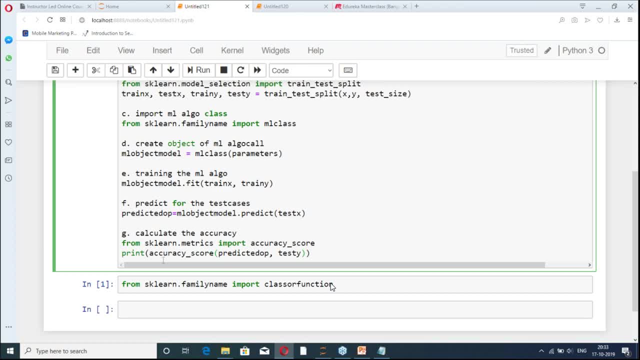 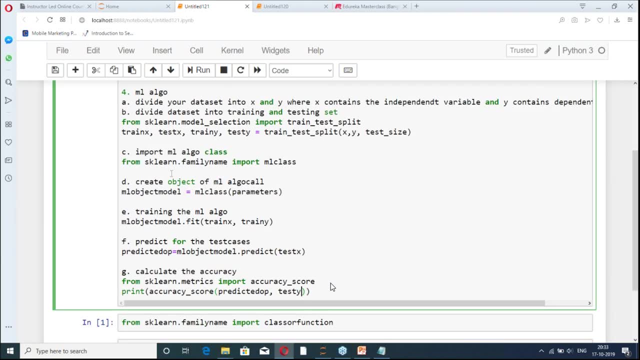 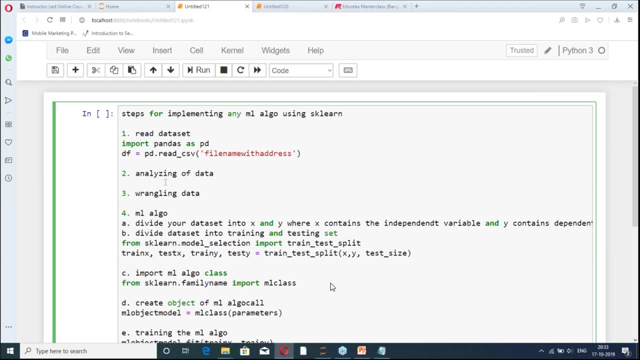 good or how good it is actually, how much, how good accuracy it is giving right. so, using this staff anywhere, any machine learning algorithm you guys can apply, okay. so I hope these steps are clear. now at least you get little bit basics with the we can say a skill, and as well, or the staffs which you can use. 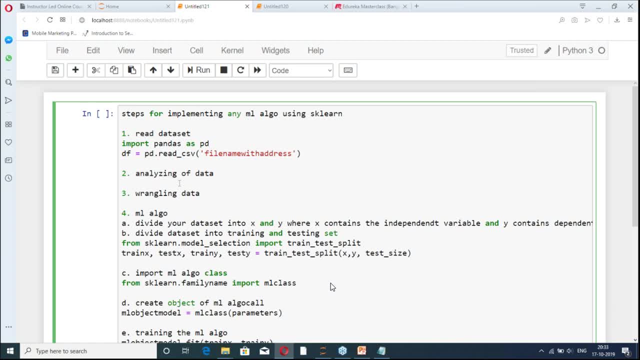 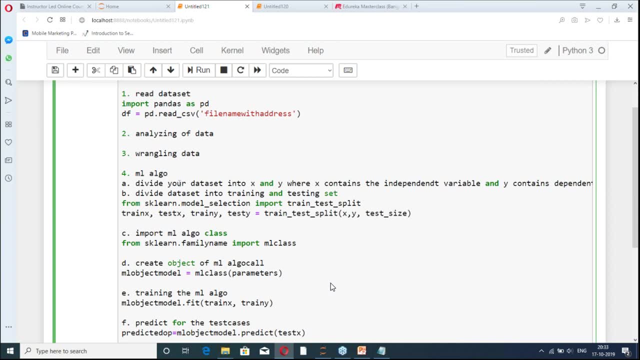 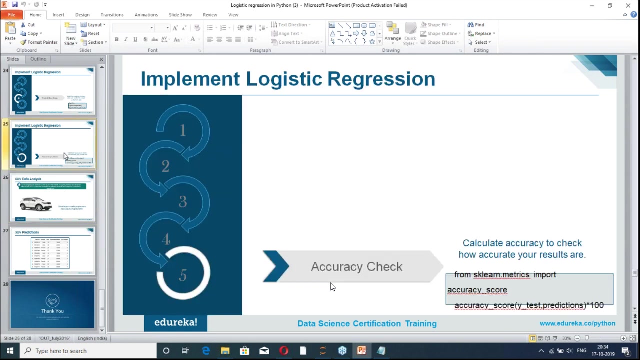 anywhere? right? so one question came from YouTube. GV shark is asking: what does accuracy indicate in Titanic data, right? so let's put this word on the slide and we need to know the accuracy of the data set, right? so in this case, we are predicting. the accuracy will depend. so this is a 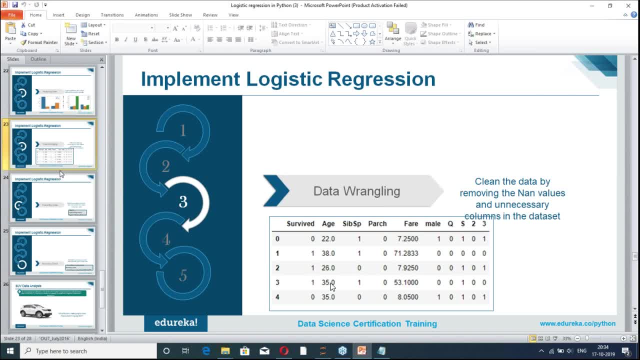 question which is we were discussing about here, right? so in this case, what you are predicting actually here is defined. so in this case, we were predicting that who will survive or who will not survive. let's say, this is a data set given. here, the first row is like here: this is given whether this person 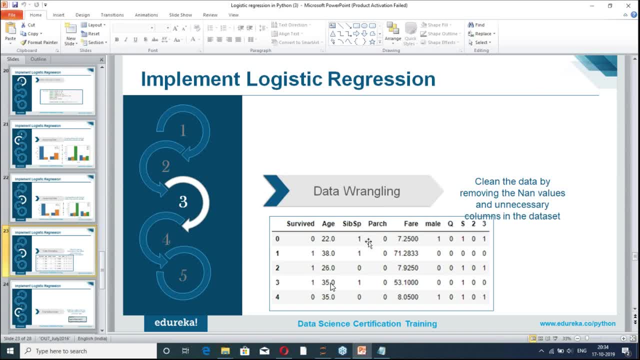 survived or not. age is this much. these are simply. this is basically if, if they and other values are there, right. so this is when you are applying your this model. what you did is basically you divide your data set into training and testing set right. so once you divided the 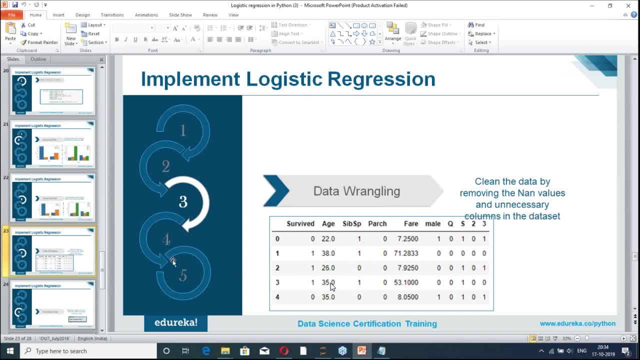 your data set, training and testing set. after that. after that, what happened? after dividing it, you train your model on the training set and then you test your model on the testing set. so, on the testing set, it tells you do not give whether a person survived or not. right, but you just give. 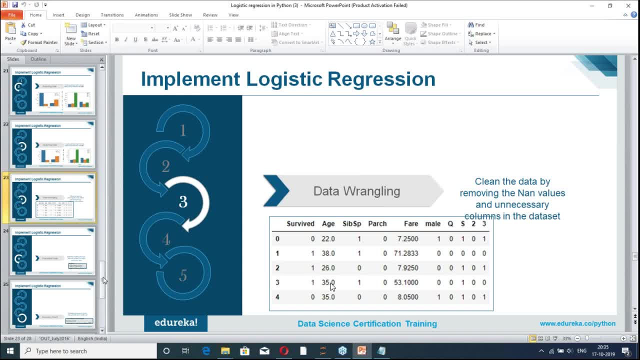 other variable values. then it tells whether survived or not. then how good result or how correct result it is giving of the survival of the person is what accuracy is telling in this titanic data set? right so i hope so. this question was asked by the gv shark. i hope so it answers. 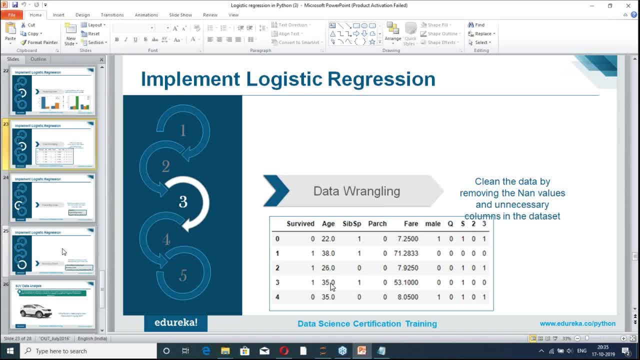 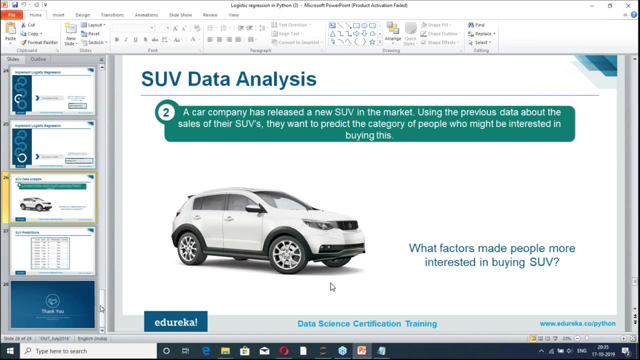 your question and shiva prasanna is saying: is possible you to use boosting algorithm in logistic regression? yes, it is actually. you can use boosting with lot of algorithms, depending what we are doing, right. but boosting doesn't mean here, depending what, exactly, what you want to do with the, what way you want to boost algorithm, right? so there, 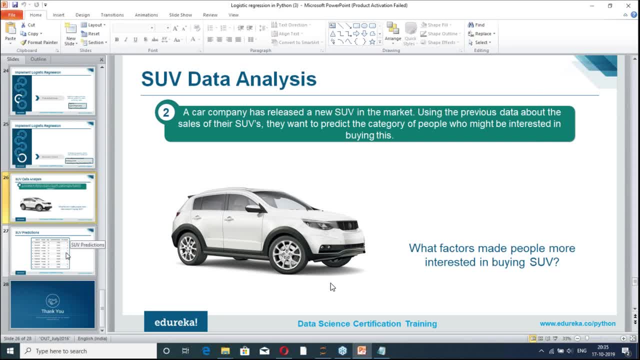 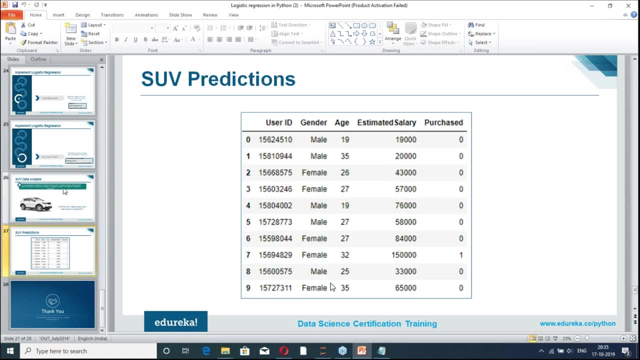 are different. different ways are there. so, depending what approach you are using, right, it will so like, for in some cases it will not be so what you guys can. so this is itself a whole topic, boosting and all. we will not go into detail here currently. right, but as such, you can say, if i 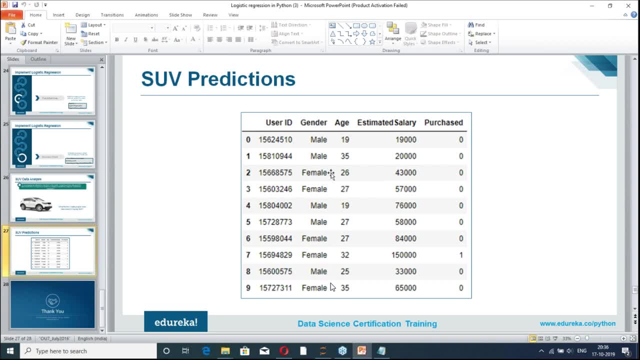 am just talking about because it will always give me one model, if it is. if you are saying that making different, different model right with the same data set, is not going to happen with the uh logistic regression, if you divide your data set into some part, then you do the boosting. 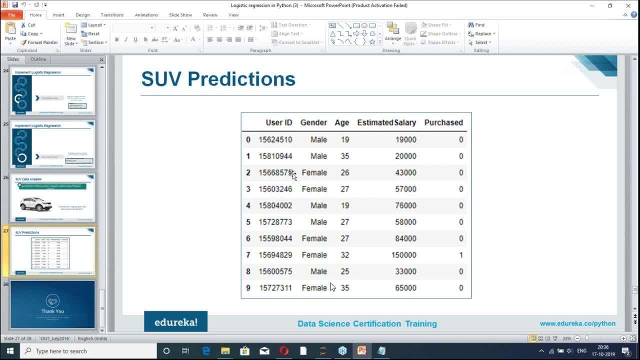 is possible, you can use this map right, but if you are doing so, there are different boosting techniques. so one of the techniques- like where you have, you know, make multiple models, definitely maybe multiple models of logistic regression. so if you have the same data set, you will be having only one. 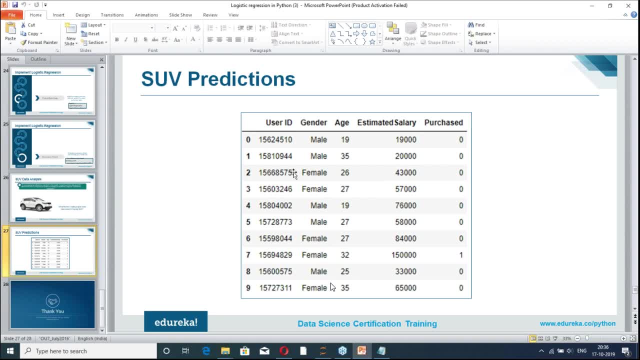 output only right same model always you will get which is the best model. but if you make some, if you take different, then you can get it. so asif is saying: can you please explain the parameter of logistic regression? okay, there are, we will. we will not go into that much detail here. we can't actually. 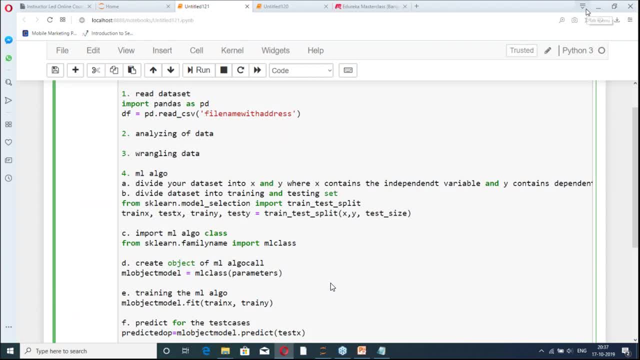 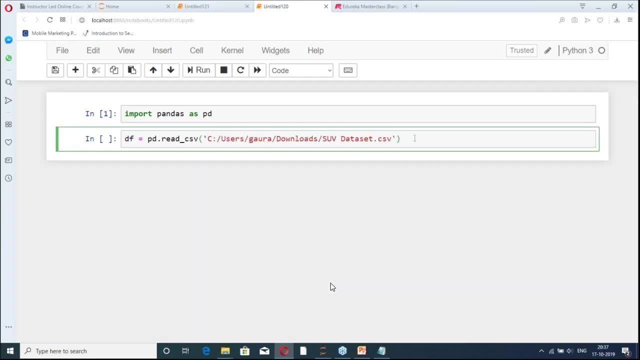 during the classes. it happens. we will keep currently in a simple way. we will keep it currently in a simple way. so for that, actually, we need to understand the whole. so this is, there is two things. one is mathematics behind it, right? so we see the simple equation. 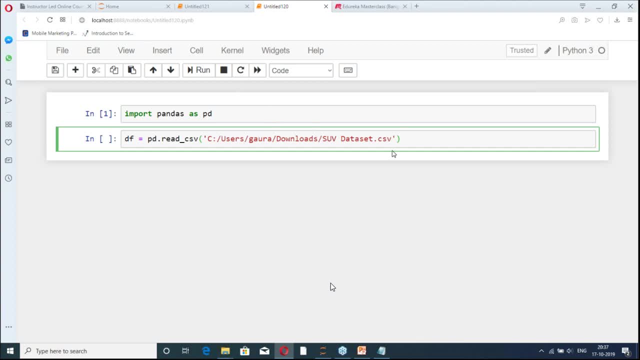 but we didn't see how the whole training is happening actually in reality. what are the, what are the things which are being used, or what is the mathematics exactly is being used to find out the right parameters. right, that is, to find out the threshold value, to find out the exact. 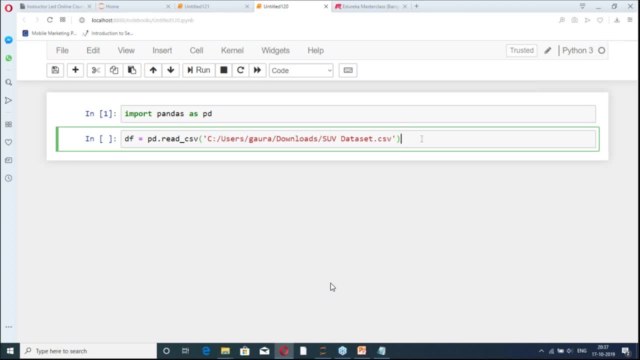 curve equations which we were using here, right. so that is we have not done. we are doing it more of the application point of view. but, yes, there are these parameters also, which is okay. we go more in depth of the mathematics which is currently out of the scope of this. 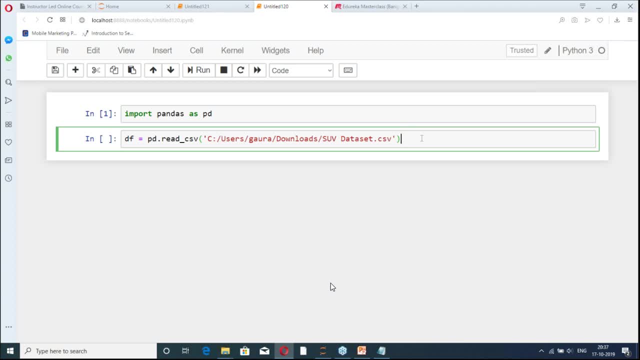 small lecture currently. okay, so let's go ahead. so one person is asking: how can we check how many families, uh, this skill library has for that? you just uh, there is a documentation. official documentation is available for sklearn. you can just google it. you will get the whole list, whole document. you will get. you just need to. 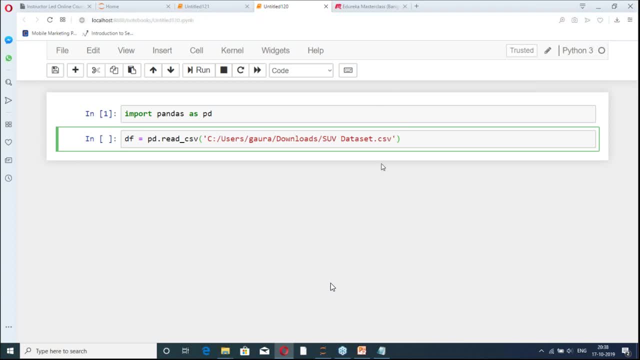 write a scalar: everything you will be in front of you, okay, so let's implement this SUV case. so we are reading this data set and this was stored here, so let me write here the F dot so we will see exactly. first of all, what are the top five rows? right? so we see top five. 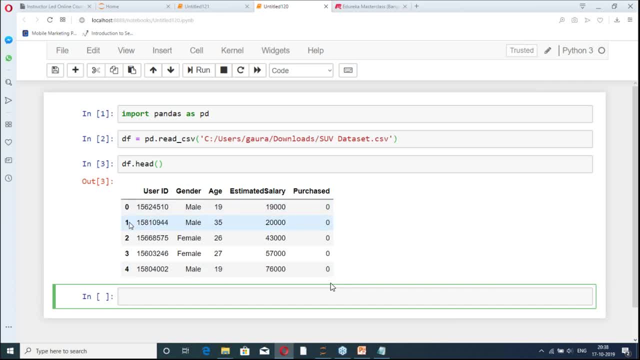 rules. these are the top five rules we here. we have like user ID, we have gender, we have age is given, estimated salary is given and whether person has purchased or not, it is given right. so if person has not purchased, it is zero. if person has purchased in the 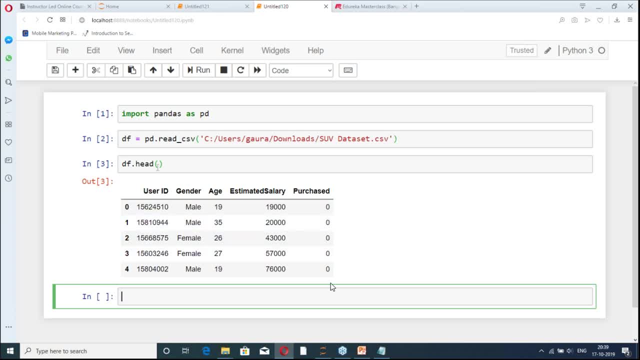 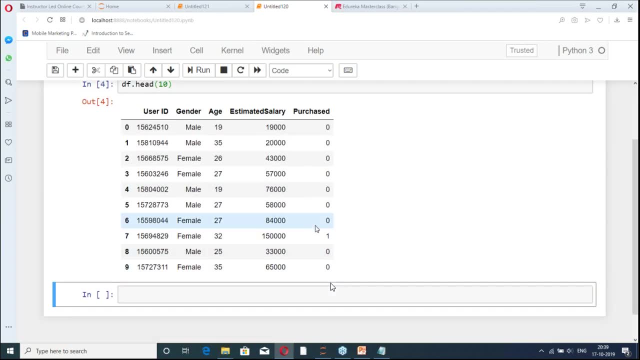 past. with this one we are taking right. so let's say, if I want to take more than five, let's say, if I want to see the top 10 rows, then this way I can see top 10 rows here. you can see, I am getting one more, one value here at least. 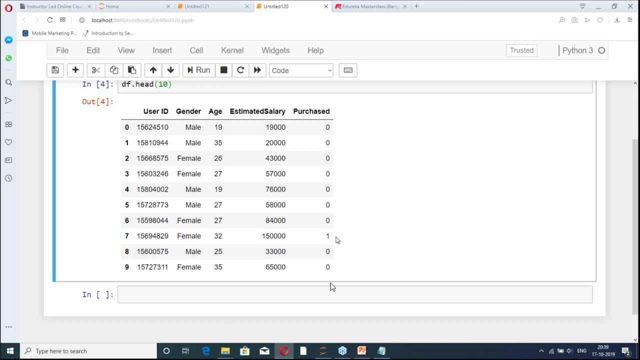 which is the person where the person has bought the car. okay, so this way our data set is, we can look exactly also if there is any. so one person is saying: kindly provide the data set, then we can practice. so I, you can get it on the website of as you like. if you go, I do. 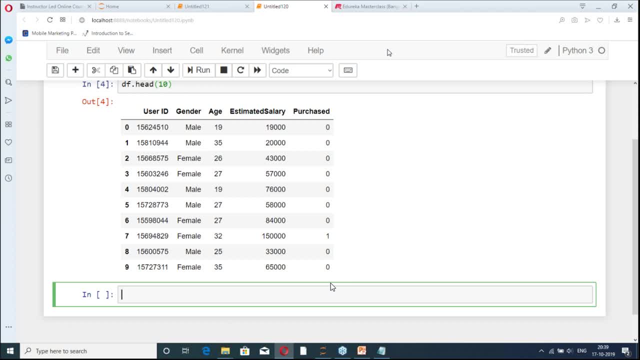 record or call. you, write as you with data set or maybe if you google it you might get it actually right. so it has been mailed to me directly by: I do as you are cutting and but that data set you can get on their website as well, okay, or even by googling out, so you 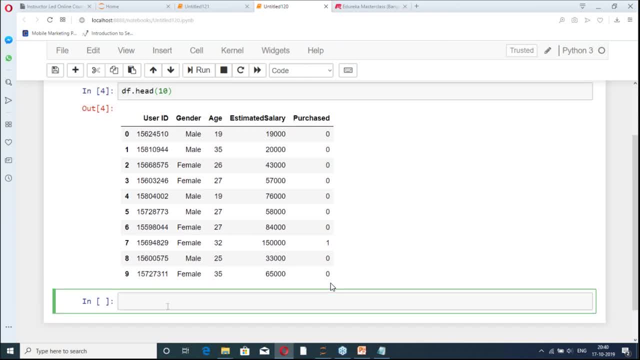 can get it easily. this is open data set. so yeah, so this is a data set. here we have right. and now, if I want to see exactly how many roles are there and how many columns, so I can see here there are four hundred entries. are there right? so first it is user ID, which. 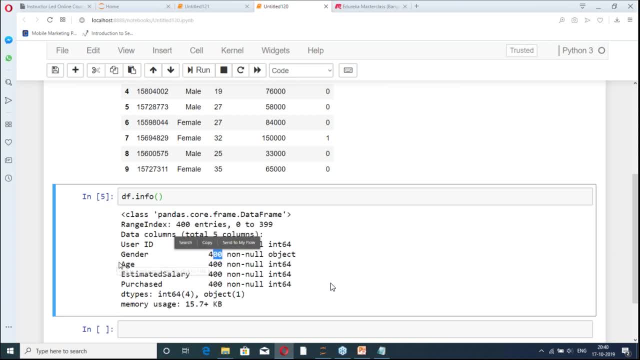 is having four hundred value next to the sender, which is four hundred value, age, four hundred estimated selfie: four hundred values are there? purchase four hundred values. so what we can say? we have to build four hundred rows and each of these column has four hundred entries. it means we doesn't have any null value, right? if you were having any null value here, it? 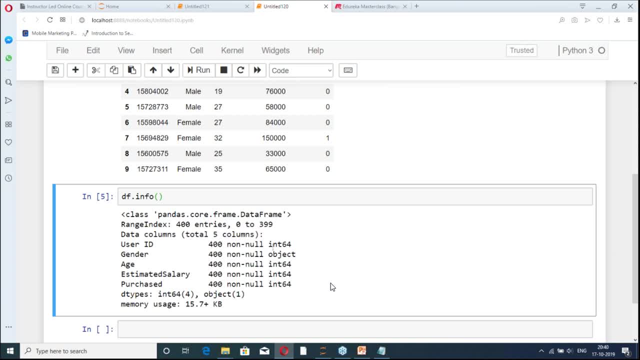 was written, or itself, for me null. and here it is given. what is the data type? like integer data type, object here data type for this, this is integer data type again, and so on. right, as well, as it is showing us how much memory it is taking. 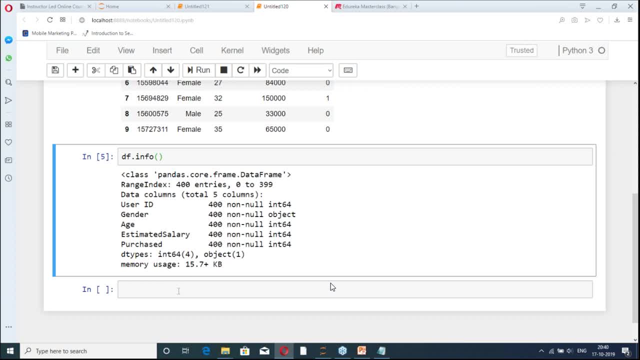 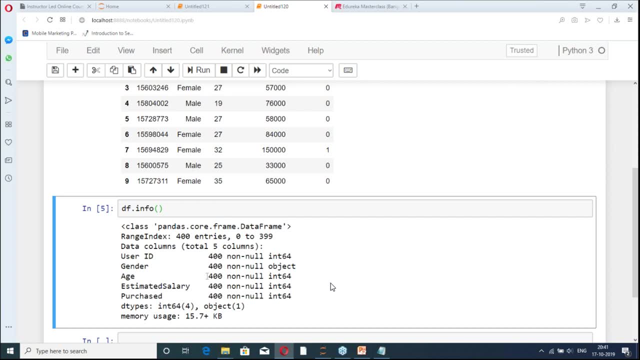 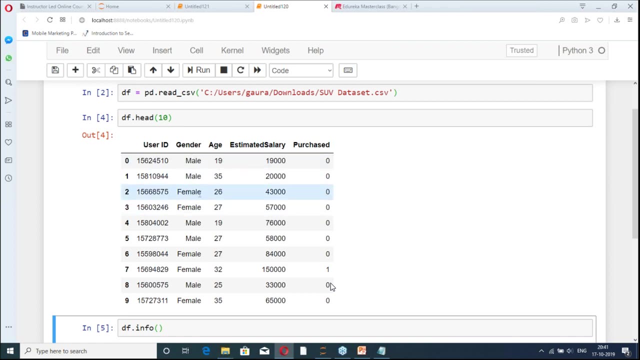 So this is the data set here. Okay, now, after reading this data set, so there are, now we need to. so this is clean data set which we know already. otherwise we might need to work around this. so, keeping things simple, even though gender might be important variable as well, right, so we need to analyze in reality. 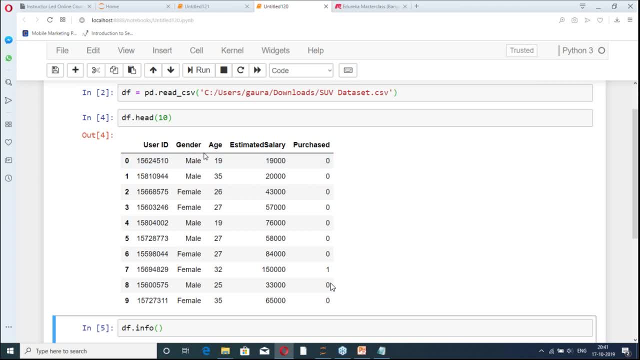 properly that which which variable are important or not. but in this case let's keep it, make it simple currently so that we can focus more on the logistic regression Or classification rather than looking on analysis and other parts. let's take up those variable which are a mathematical variable or numerical variable, like age, estimated salary purchase. 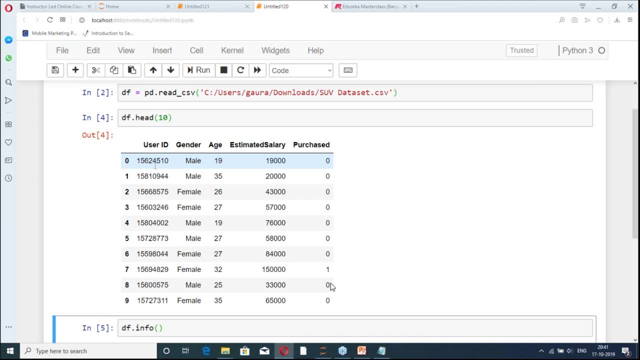 user ID. shall we take user ID or not? then some of you might already understood it properly that user ID must not be taken by so, because it never matters whether person will call by a car or not- on the basis of some random number user IDs- It's kind of random number right which has been allocated as whenever he or she visited. 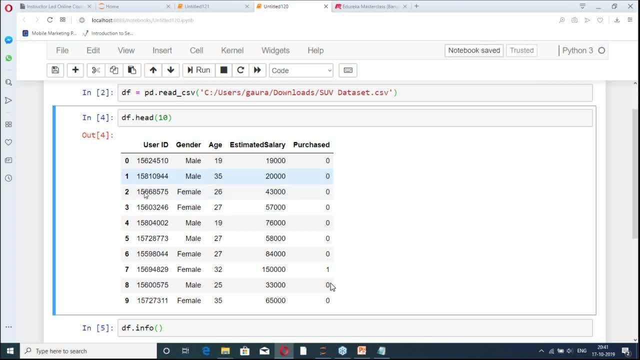 the, let's say, your shop or whatever day you were able to get the data set into your system. right, it is just a random number, completely. so user ID we doesn't need to take into our analysis. gender we can take, but currently we are just keeping it aside to keep it simple. 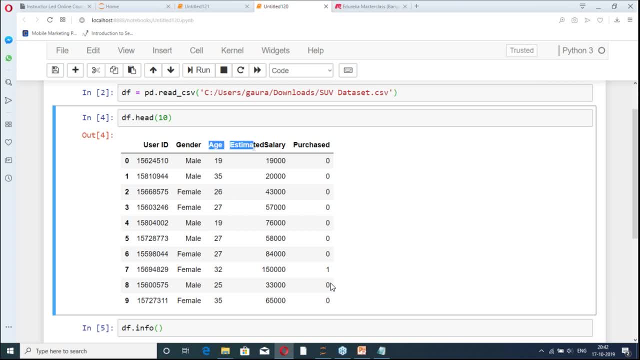 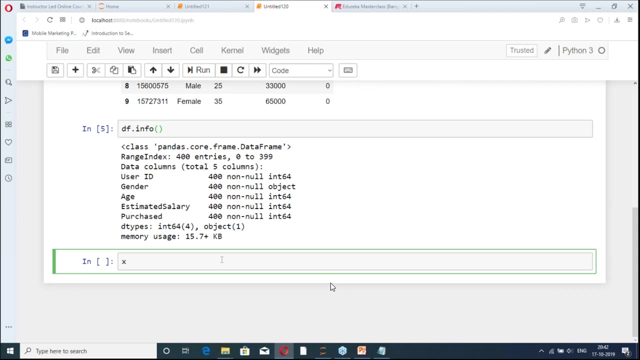 so we are going to take our input variable or independent variable as age and estimated salary And the output variable we will take as a purchased variable, right, or that is our dependent variable. we can say OK. so how we can take, there are many ways we can take, so some ways you guys might have. 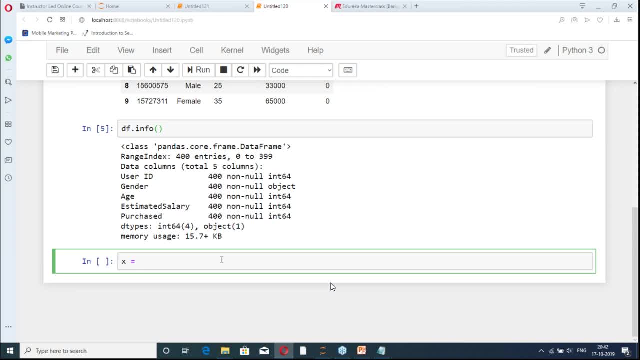 seen already yesterday. I can do it by writing the column names as well, or I can use a function which is I log function. So I use the I log function Here. I tell From which column to which column I want to, so here if I'm writing call, and so before 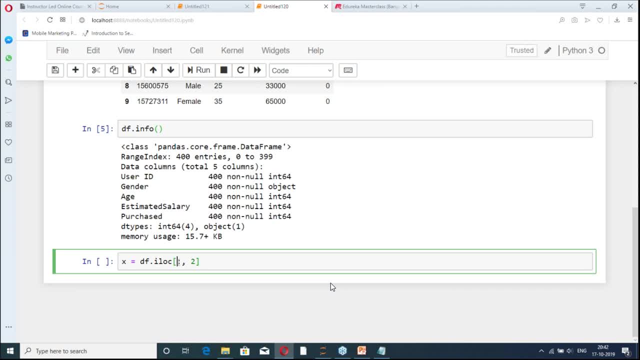 the form I test which row I want to keep in my data set. if I want to keep all the rows, I will write here: column right. it means keeping all the rows and before comma right and after comma I test which which column I want to keep. so I am saying from the second column. 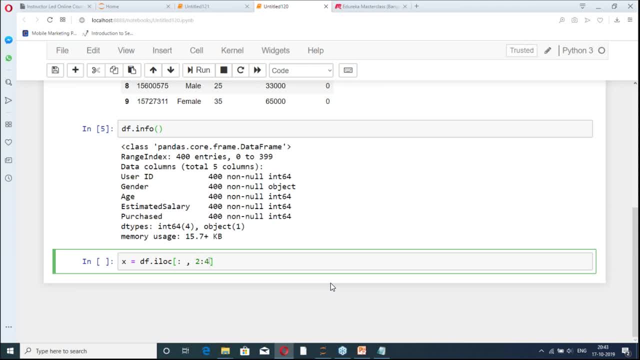 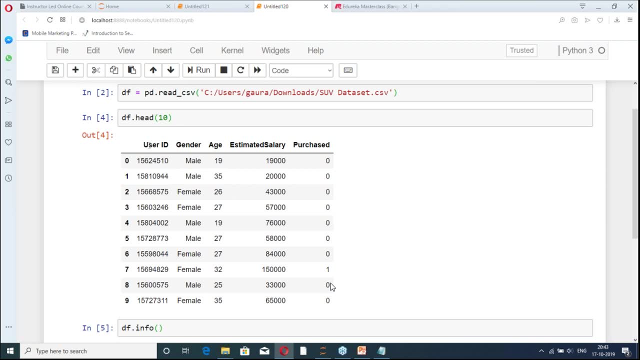 it should start until fourth column, but fourth will not be included. whatever I write after calling it is not included. So it means second column and third column, Which is my second column. This would be treated as the red column, first column, and this is my second, and this is my 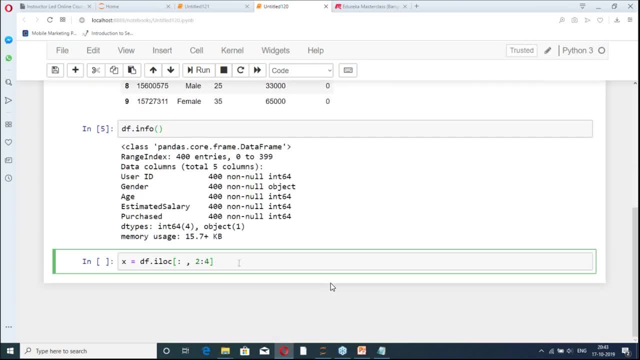 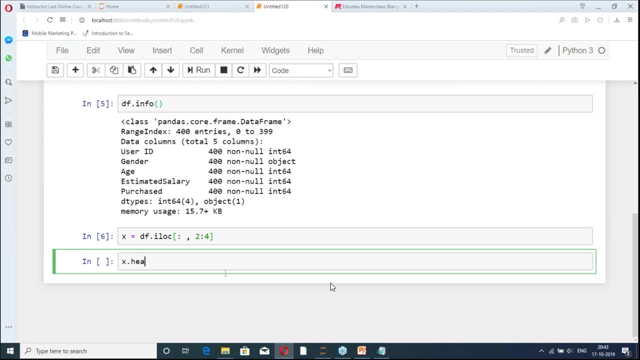 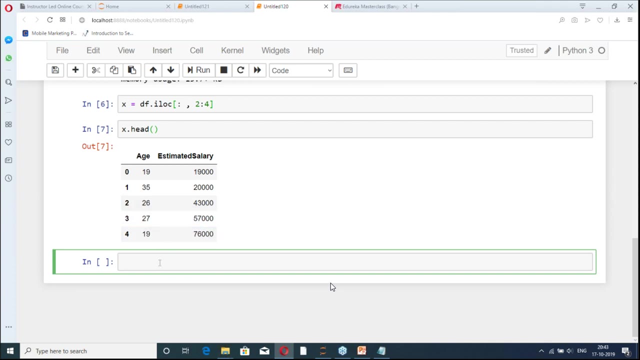 third column- So these two I am keeping in my acts- right or input variable, so we can take these and we can look also at stock head right, so we get these values right: age and estimated salary right. so we got all these two columns. Similarly, we can take the output variable, which is we can do in any ways we can write. 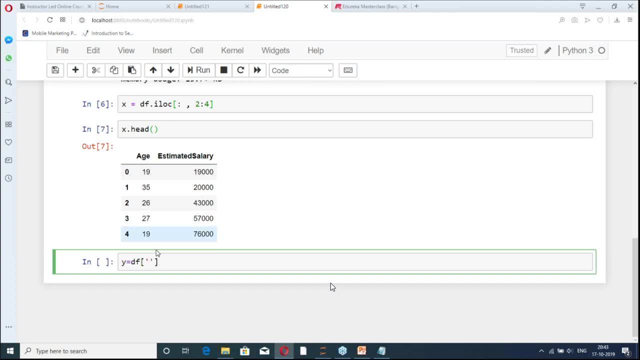 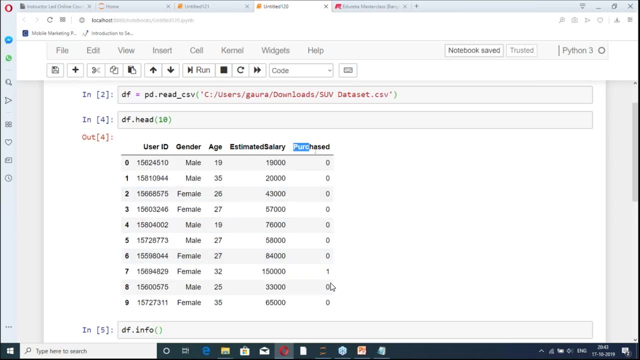 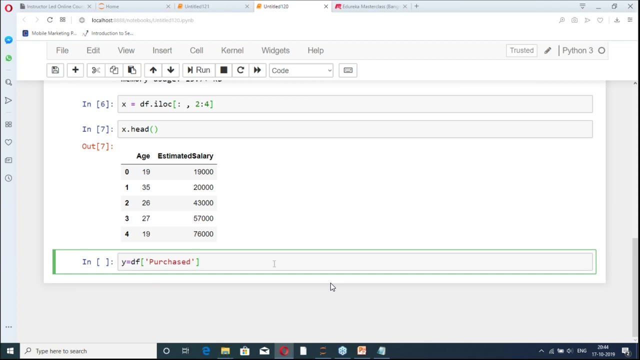 directly column name here or we can use again I log function also. So let's say this time we are taking the by using the column name, which is purchased. I will just copy paste the name of the column right. so if I show you top five rows from: 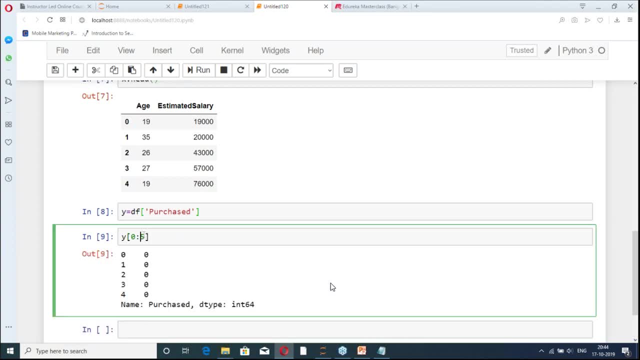 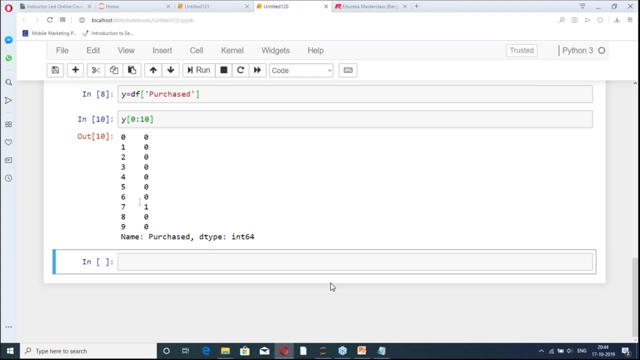 zero to five. these were their output. values were zero, zero only, but if I show you top ten, there are one value is one as well. Right, so we get our data set. now, what we want to do, as you guys might remember from these steps which I showed you earlier, that next step is basically dividing my data set. 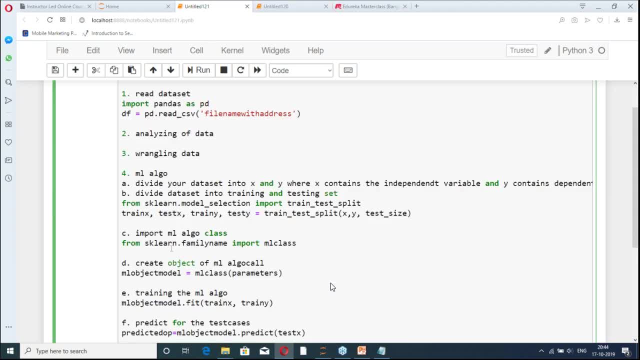 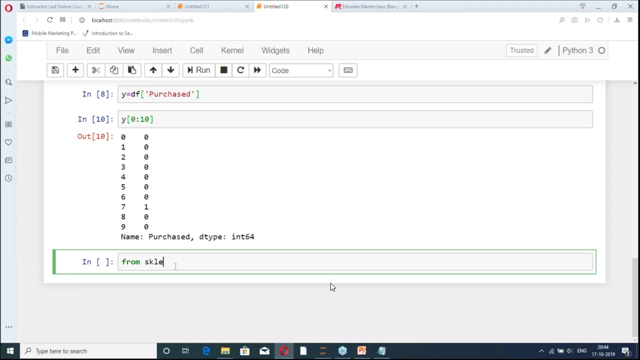 into training and testing part, right? so you see here what was this tap I showed, right, so we did this thing till here, right now, what we need to do: dividing our data set into training and testing set. So how do we do this? first of all, we need to import from SK learn dot model selection. 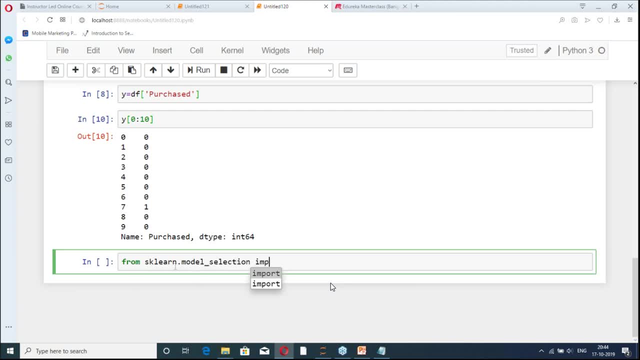 we are going to import our, that is, our train test split And then we can divide our data set into train X, train Y, train X, train Y. so it is doing late auto completion actually, so it has added extra here Right: Train X, Train Y. 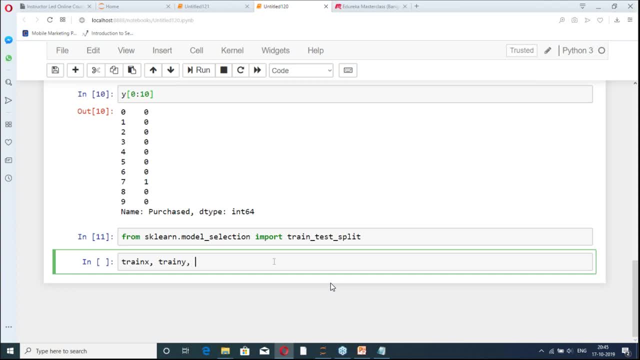 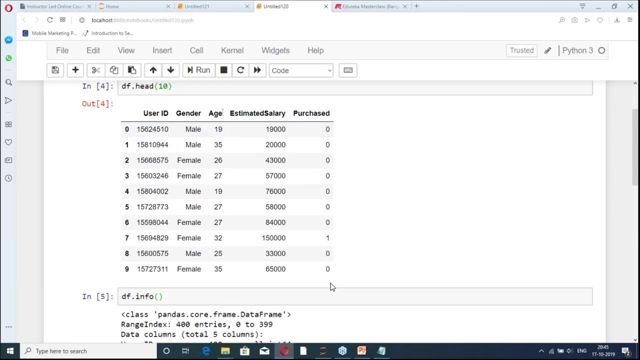 And after that, okay, one person is saying Rowan is saying we can make male as one and female as zero. Yes, definitely, we should do this in reality. that is, we should keep this column as well. right, and in reality we should look exactly all of these columns one by one. that is there. 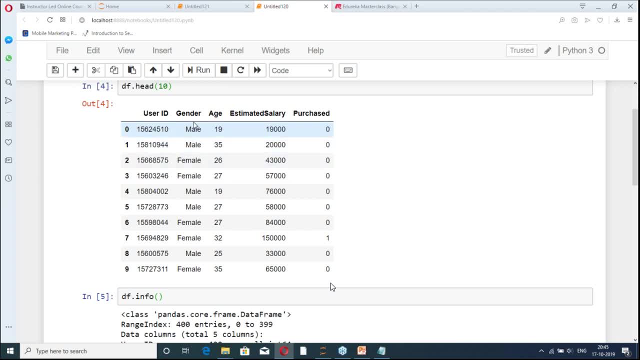 any column out of them which is not useful at all. it might not be mathematical, but it might be very useful at the same time. It might be mathematical- let's say eight- but it might be used as completely. in reality, when we do the analysis, we are keeping the analysis part of the actually here, right, but 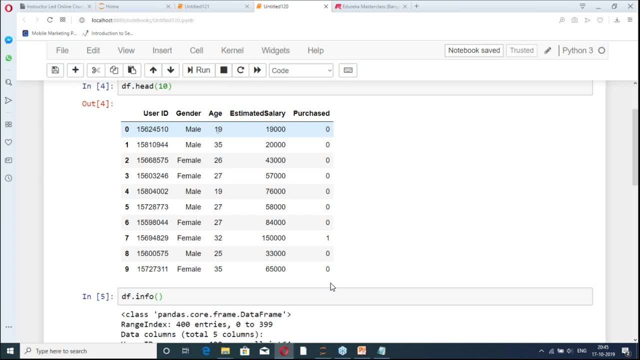 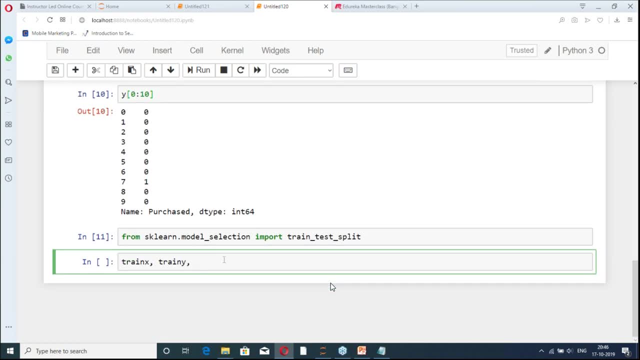 when we do the analysis, we need to exactly look for each and every column properly and definitely, if it is not into the numerical form, we need to convert it right. so but we are keeping it currently just away, the analysis part, because we have not done the pre-processing. 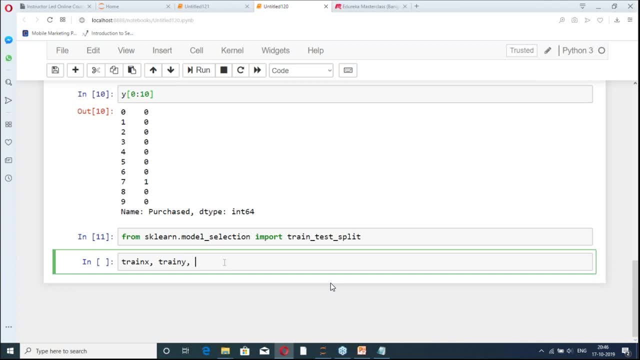 and all here. a lot of people have not studied, So we are just keeping it simple, Right, Simple way. So we do train x, train y, sorry, the first thing will come is the test x. after that train x, the thing will come, the test x, then we say train y, then we say test y and then we call. 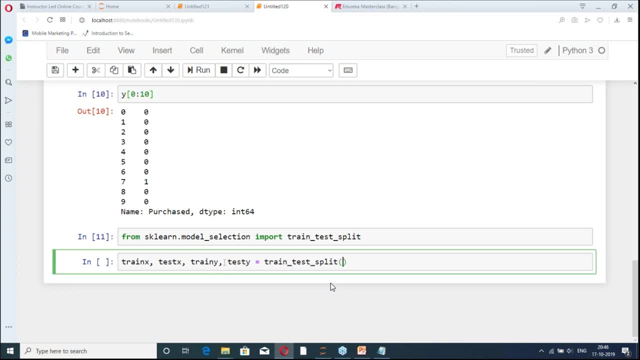 this function, which is train test split. we pass here x, y, we tell what is our test size. we can take anything. Let's say this time: Out of total rows, we have 400, right? so out of 400 rows, let's say 100 rows. I want to keep. 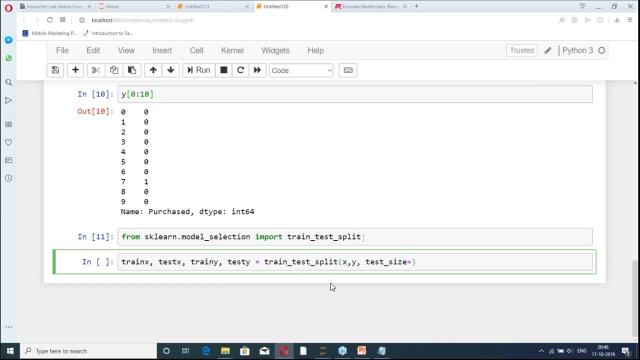 for the testing and 300 for turning. so in this case test size will become 25 percent. so I write here 0.25. right, we execute this code here. so after x. so here we divided our data set into two part, that is, training and testing part. right, okay, so again. so now I'm 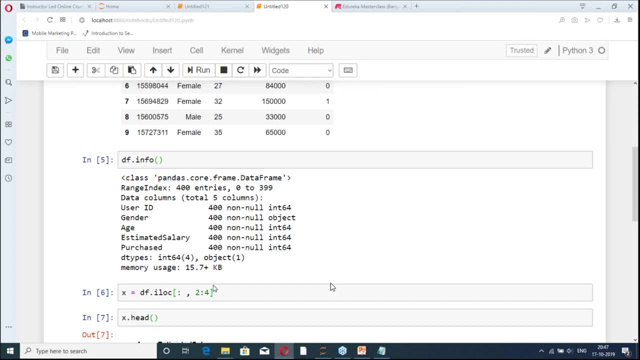 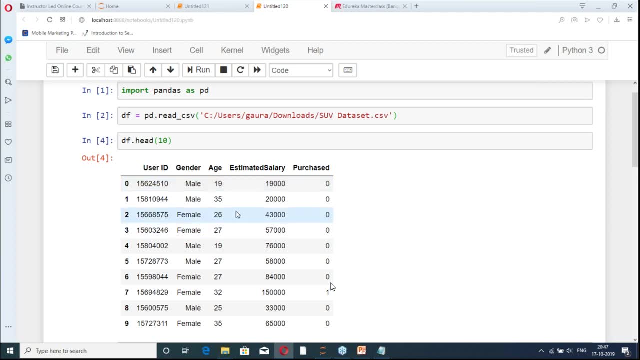 thinking I should show you few pre-processing stuff as well. so one thing you see here: age and estimated salary. actually, if I do not do, our result might not be good, it might be so much bad. so at least here we should do something. so what you see here? the age value. 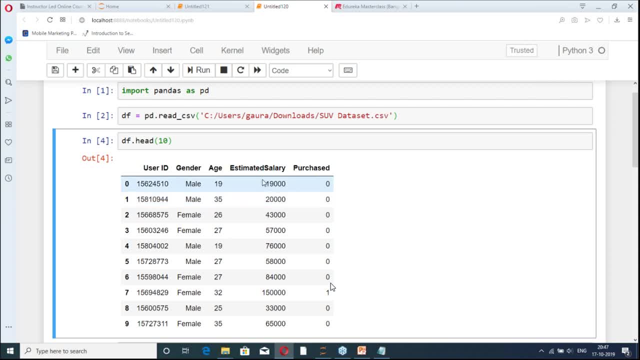 would be changing only from 0 to 100, while salary would can be changed from 0 to crores, millions, billions and all right. so there is so much variances there into my estimated salary column Compared to the edge column, age column. so what would happen in this case? because here 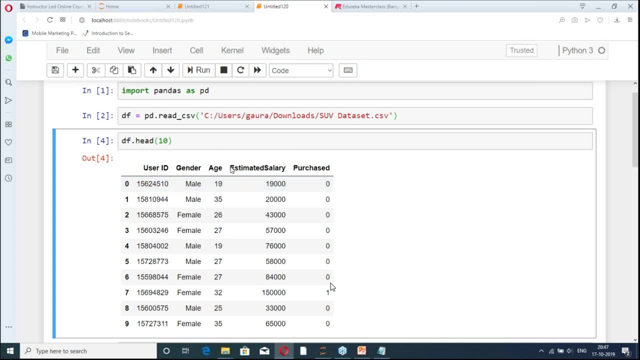 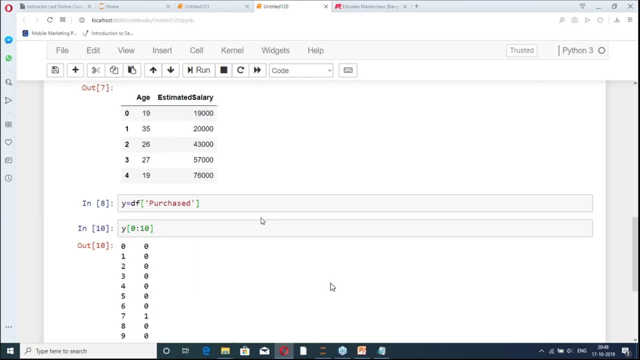 we have, the more variances, so estimated salary will become a dominant column compared to age right. so which is which we do not want to right. so what we can do is we need to scale them down or up. we can normalize them right, so we can use any method for scaling. so we 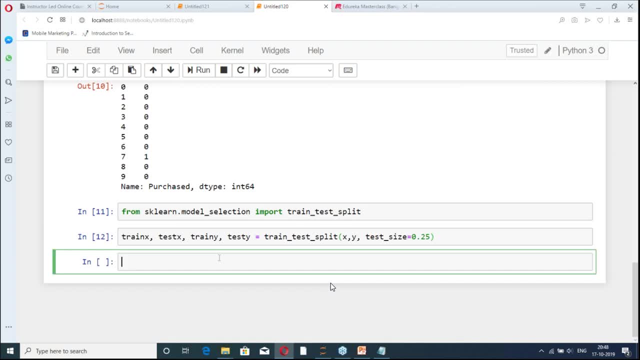 use feature scaling. so we are going to do feature scaling now and we will do the standard scaling. So So let's first do what it brings the mean: to remove the mean from the data and make the variance equal to one right of the data set. it scale them in such a way, such that 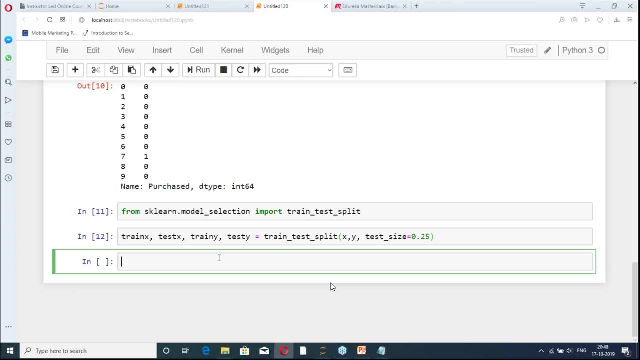 mean is removed from the data and the variance becomes unit right, unit value. so this is what we are going to use. so for that we have from a scale on, we have pre-processing library from which we will implement. Okay, So we have a standard scalar right and using this we are going to scale out right. so we 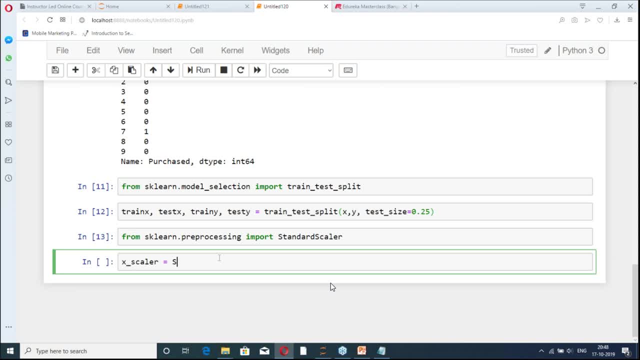 create an object and scalar is equal to standard scalar Right and using this we do the X-Train scaling. so we do X-Train scaling by calling this function X scalar. we call dot fit transform Basically, So. So basically it is scale down in the correct form by fitting down and then transforming. 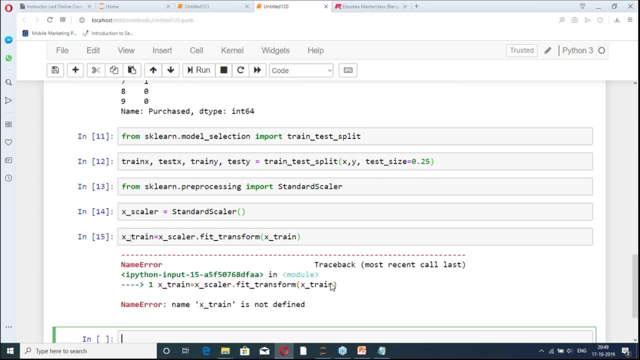 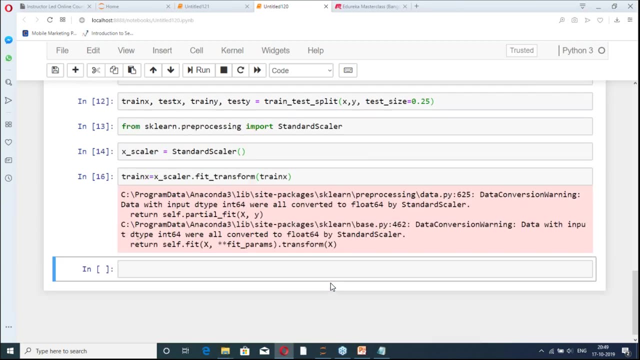 down. sorry, this is not X-Train. this is a train X which we have taken here. Here also, we need to write it as a train X. Okay so, we did this thing. similarly, we do for the test access as well, Okay So. 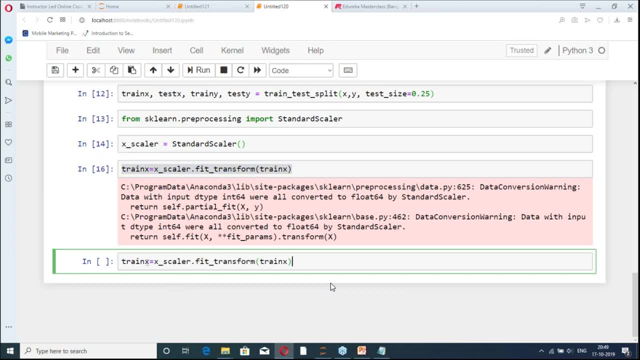 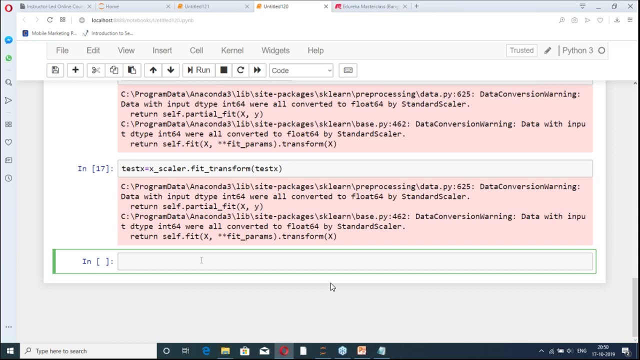 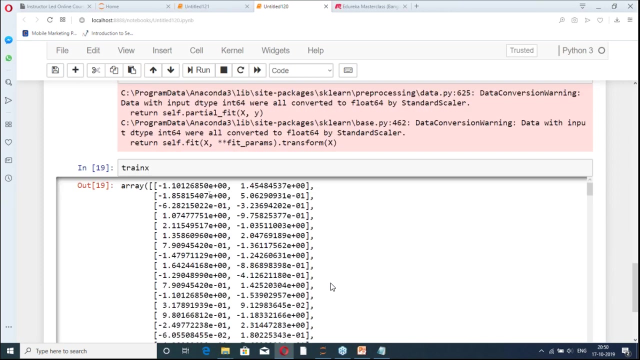 So, after doing this thing now, so our data is scaled, scaled down properly. so if I show you train X, dot add, Sorry, So this would be my numpy array actually, So you can see it is very much around, you know, near to zero, to one right, so you can. 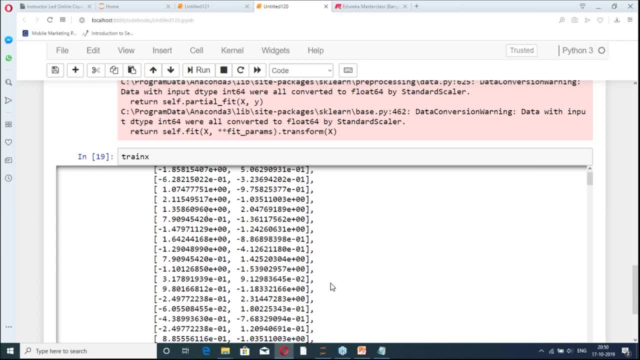 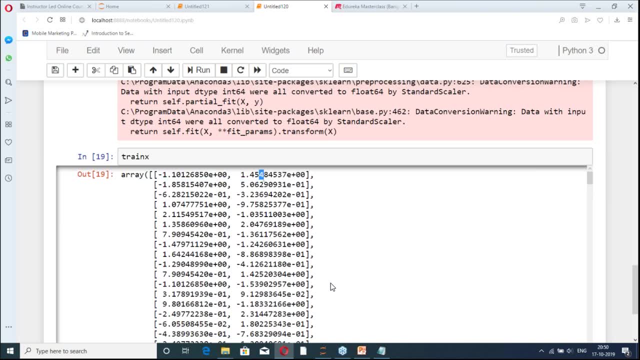 see minus one or one around very few values you will see which are very high, but mostly you will find is very much closer to zero, to one, and you can see- this is second column- is for what purpose this second column? it was our salary right, that is estimated salary. 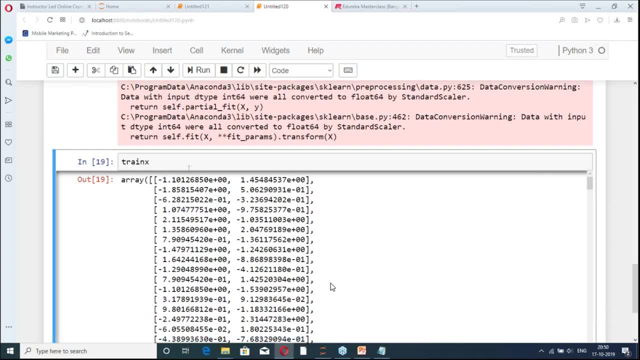 and this was age column right. So here, if you see, this is my age column, Okay. So this is my age column. how the values has changed and this is the central column, right. so these has been scaled down so much, Okay, so that it will not impact much, so both have the same impact on the final output, right? 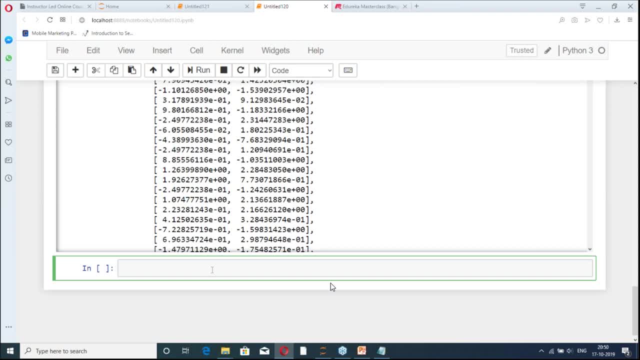 so we are giving it equally importance. otherwise, because there are more variances there in this entry, so it would impact more, right? so here now we are going to make our logistic regression model, Okay, Okay. So here we are going to do a scale and dot again. this is in the linear model family. 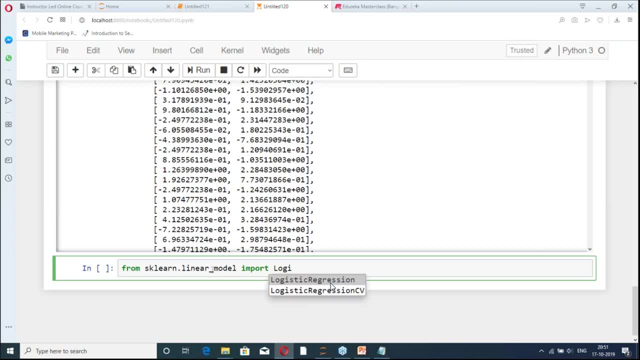 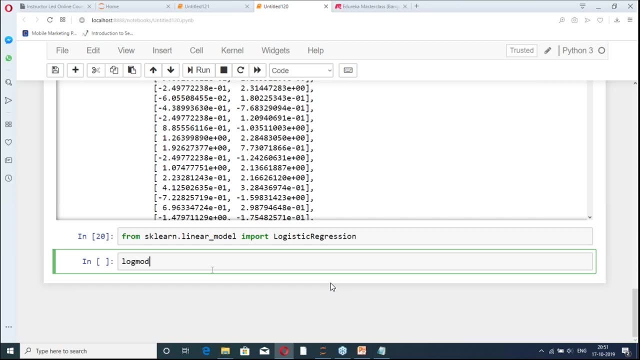 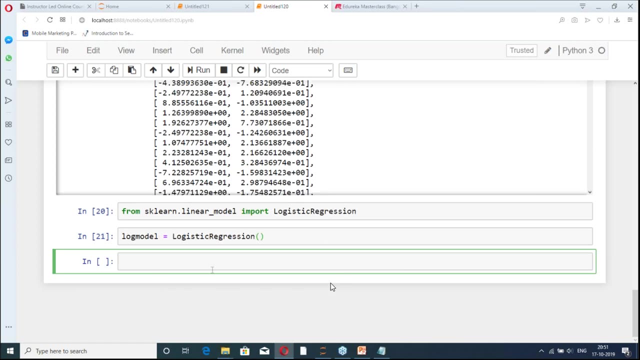 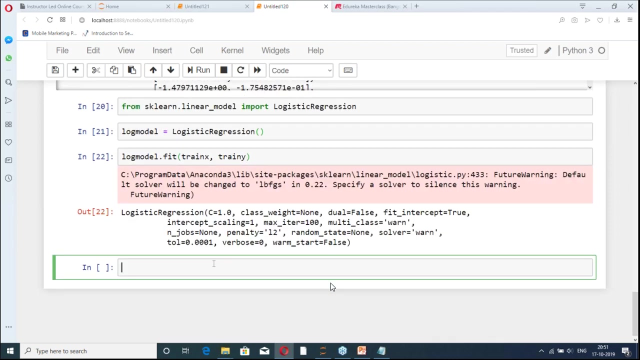 import logistic regression, right. so after that we create its object, let's say log model, we call it and we do here logistic regression, and after that we can do the fitting dot: fit. we pass our train axis, Okay, And the train line. So model has been trained and now we will be doing the prediction, right, so let's say predicted. 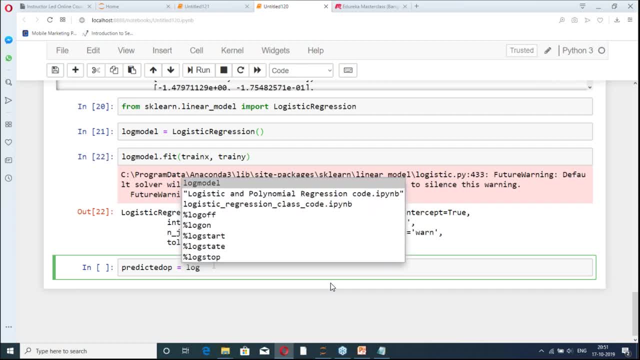 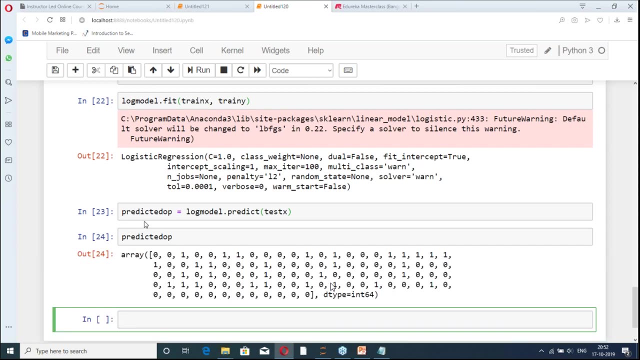 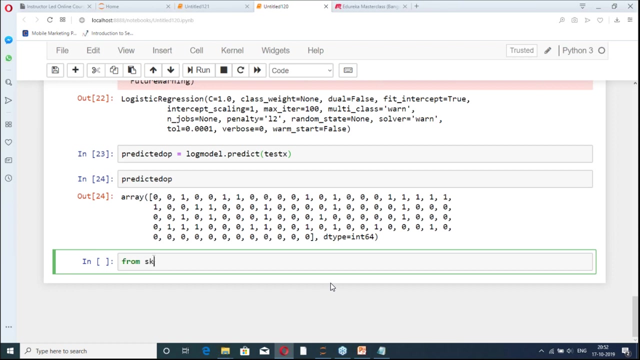 output is equal to log model dot predict. and here we pass the test x and we do the prediction here. so we write here normally, prediction here. Okay, So you can see these are the different values which has been predicted. but now we want to calculate accuracy, so we write from sk learn dot matrix, import accuracy score. and if you 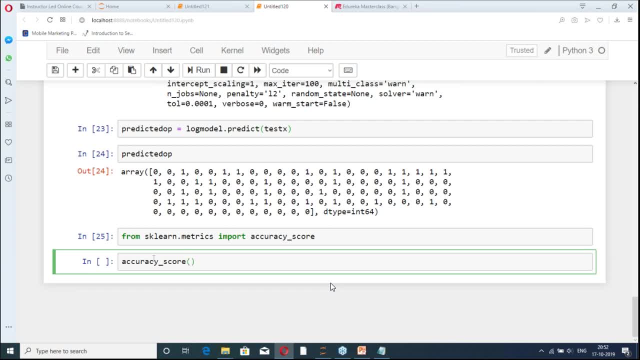 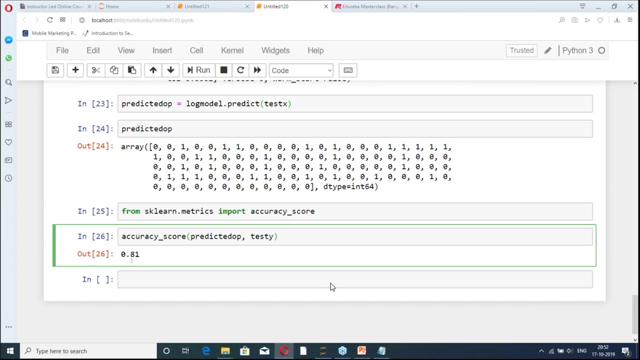 write here accuracy score and at the same time we pass here what is the predicted output and what is the correct output. that is test one. Okay, And we see here it is coming: 81 percent accuracy. right, so this comes out of one sort of one. 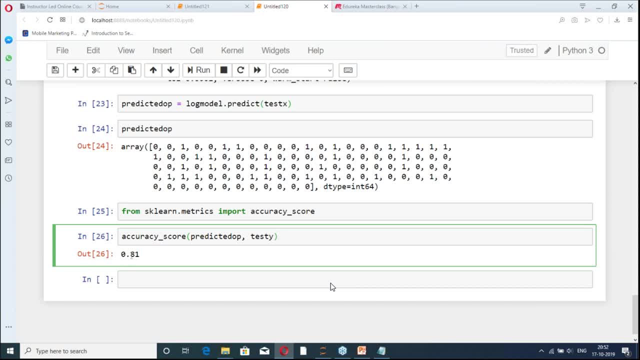 it is coming as point eight, one sort of hundred. we can say it is 81 percent accuracy, right. but after doing thing, this thing, you might be interested in knowing exactly how many correct values has been predicted for one and how many correct values has been predicted for zero sometime. what might be the cases? cases might be there, like you know, like it. 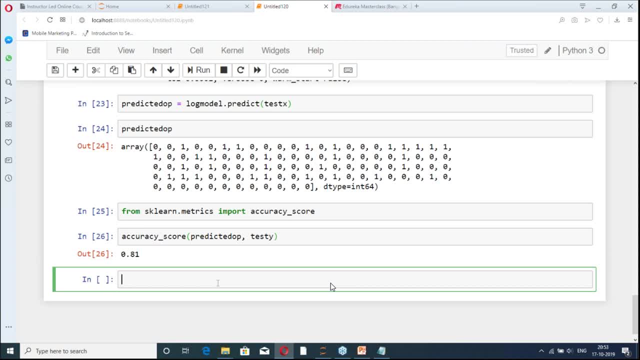 might happen. let's say in my data set if I have lots of zeros are there and very few one are there, right. and let's say out of hundred only 81 goes zero and the 90 values were one. so it predicted all value is zero on its. automatically it become 81 percent accuracy. right, but it 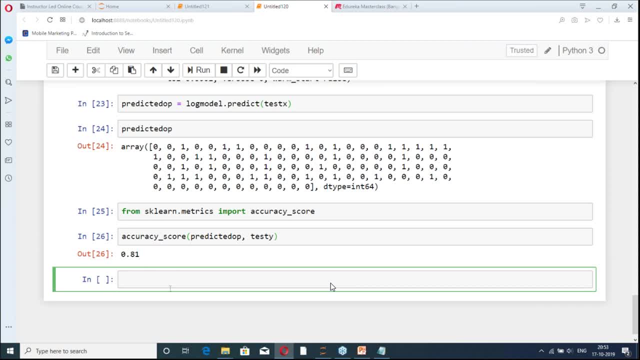 didn't predict even a single value which belongs to class one correctly. so if you want to exactly know that which class has been predicted, how many values correctly has been predicted in which class, then for that we have a confusion matrix. So if you want to exactly know that which class has been predicted, how many values correctly, 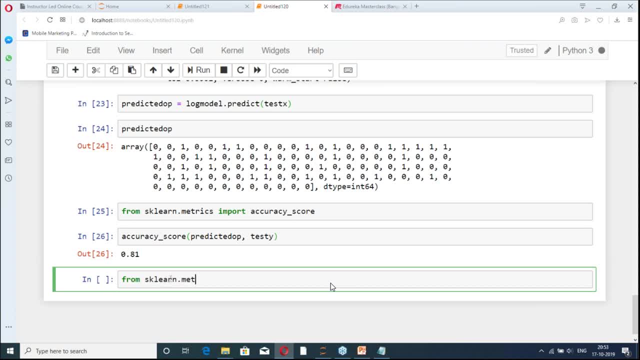 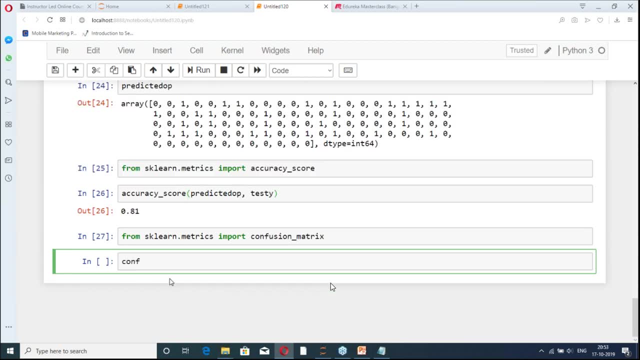 has been predicted in which class, then for that we have a confusion matrix. So if you want to exactly know that, which class has been predicted, how many values correctly has been predicted, how many values correctly has been predicted. so again, for drawing this thing from sklearn dot matrix, we import confusion matrix, right, and then we call this confusion. 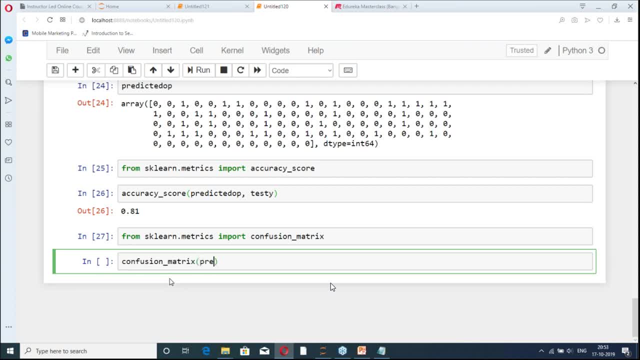 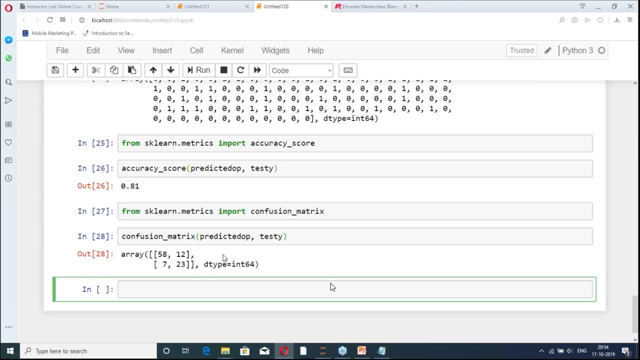 matrix function. we pass again our predictor output and then we give also test y and here you are seeing this particular metric is being printed right. so there seems to be question in the webinar. So, um Jay Shankar 2 is asking: is it kind of log? which thing you are asking kind of? 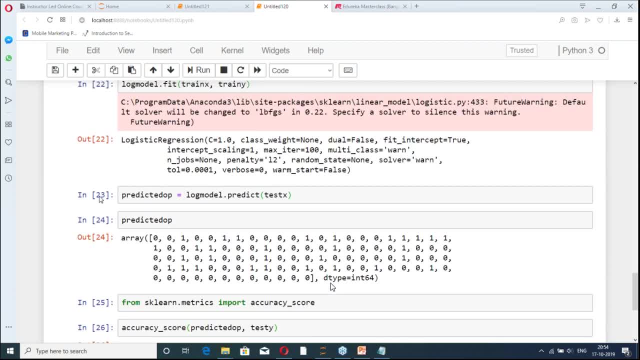 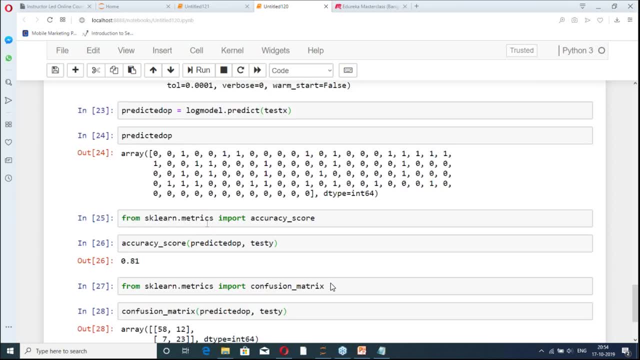 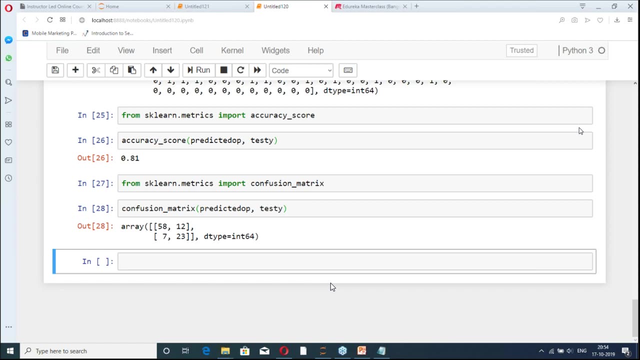 law, which particular line number are you asking? this log model, this logistic regression? okay, normalization, this is, yeah, you can say no, this is- there is a formula for that- actually the form life. if there is a scalar, we call it as a scalar, we are calling it as a, we are calling it as a standard scale. so there, 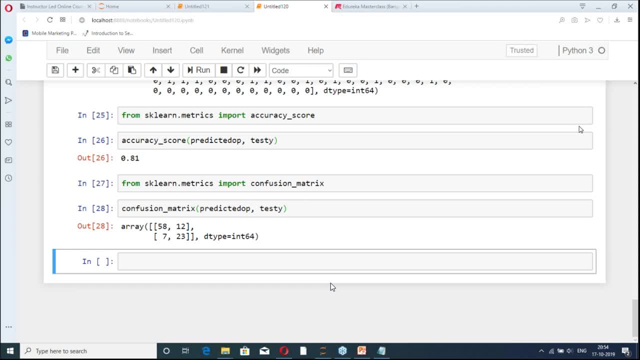 are different method of scalings. are there, right? so one is not? normal normalization. is there, then, where you normalize your values in between a particular range, like maybe in between 0 to 1, and other ways? are there, right? so this way, do what actually this you can think, as this particular method is not? 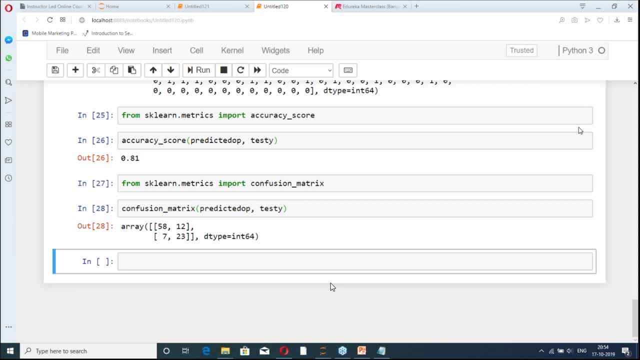 doing the applying the log actually onto this, but there is a for that and formula is actually X minus mean value divided by the standard deviation of this particular value, so that the standard deviation become one and it the mean is removed from the data side. okay, does it answer your question? is it clear? okay, great, so 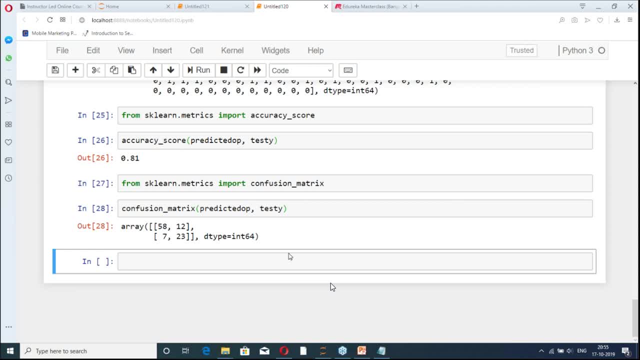 here. let me see. if any other questions are there, then we can apply the here. let me see. if any other questions are there, then we can apply the aware CBRT all spiral to safe right. so Shiva persona is asking and we can. anywhereiatayoii right. so Shiva persona is asking and we can. 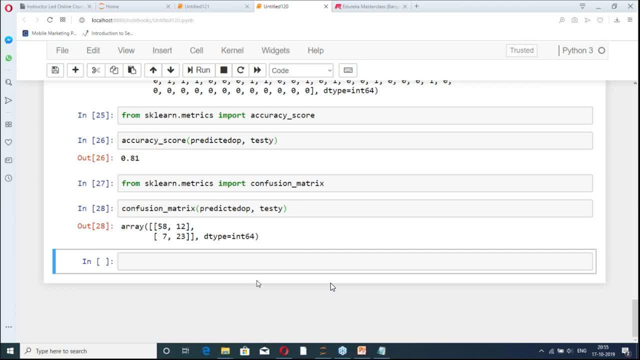 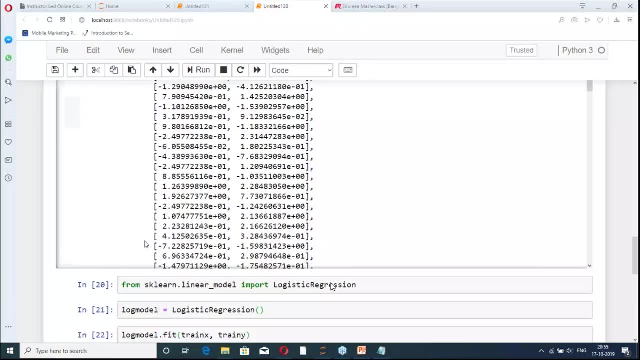 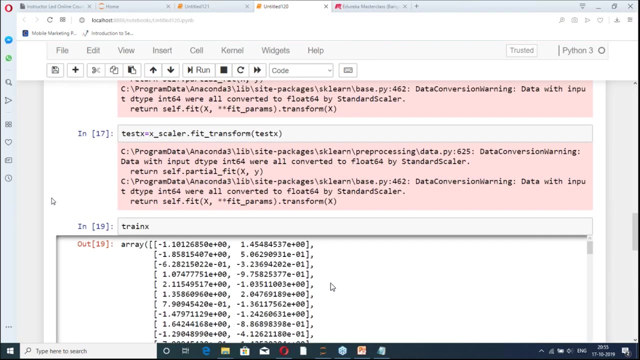 apply a lor cbr grips fiber to st beschüssing animalPU board sithalli. you see there are different, different effects, because I'm going to the Well, Shiva do está��. but each of these scaling factors have their own impact on the dataset which you can observe. so each of these scaling factors have their own impact on the data set which you will get. so it is not like that, just if I have to to reduce. 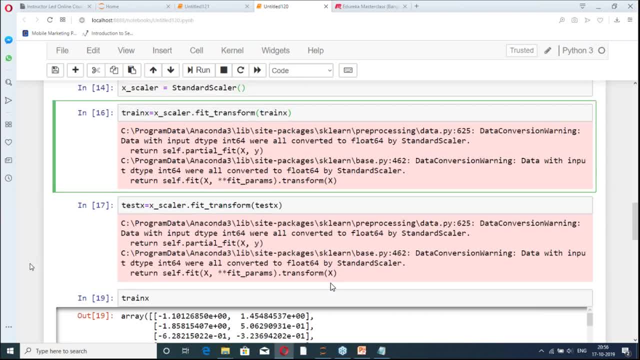 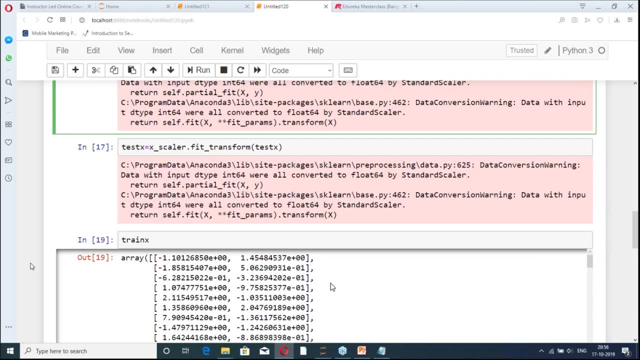 There should be proper way that you See there are different, different impacts. we can't go into the detail, for each of these scaling factors have their own data set which you will get. so it is not like that. just if I have to scale it down, then I do 10 times 5, root over 8, or I take the log values and all. no, it is not always the. 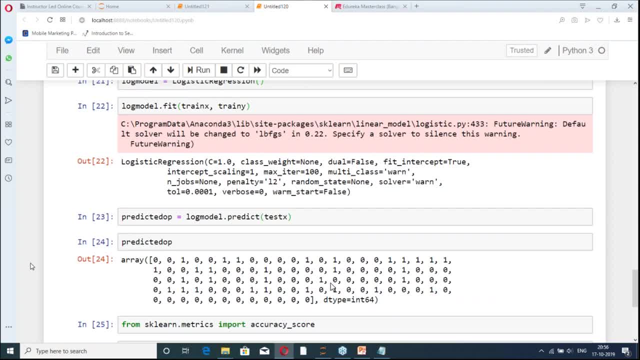 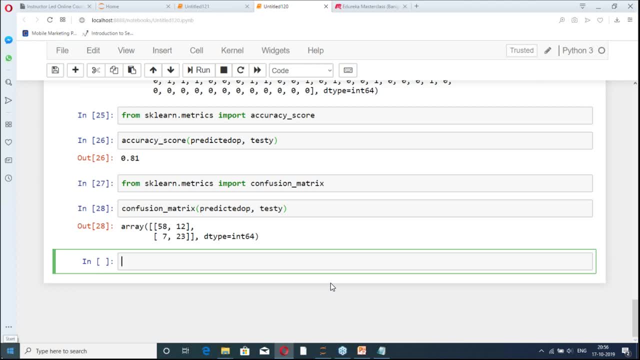 case? right, there are proper ways. are there right? we can't go. this is in much detail, but if you go, when you will go into the lectures, you go, then you might be studying this thing in very much detail. there are proper reasons why this particular method, when to use this. 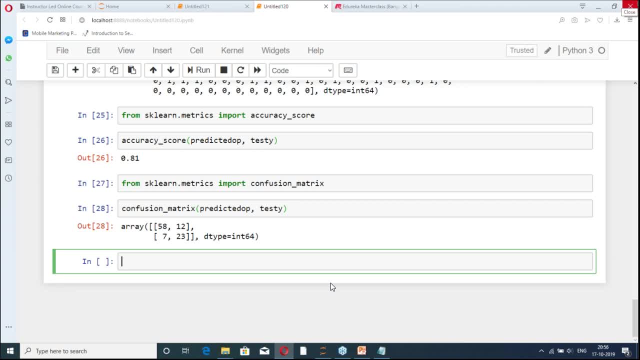 particular normalization right. it is not like using plain law is still. if you use the law, you know the range would be still would be different, variance will be still different for both the variables. but carrying this skill and method which we have used the way, it is bringing it to one variance only for both of them. okay, great, so let's go here. yeah, so. 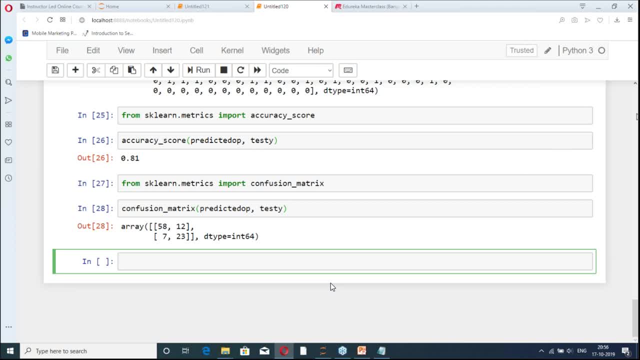 this is what we have printed: confusion matrix. So what the does this confusion metric is doing here? so this is showing. this confusion metric is showing this is the zero value and this is also zero. so we write this as a zero. this is as a one. 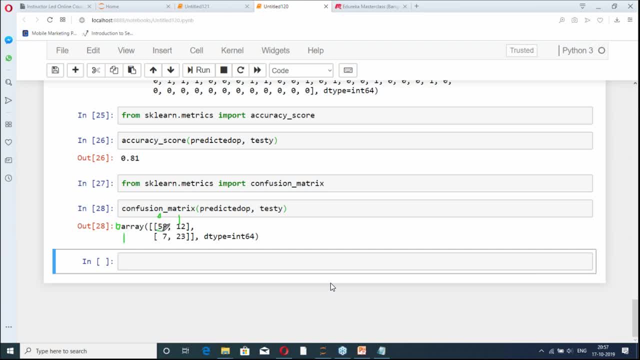 so one and this row number is a one. so what does this particular value is showing? this is showing that. so this row is showing what is the expected value and this is showing what is the predictable value. so it is showing how many value are expected to be 0 and has. 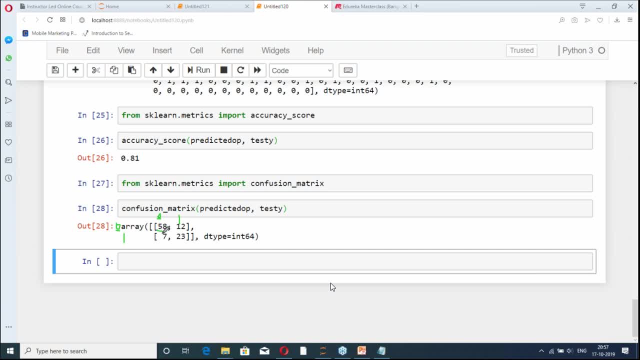 been predicted as 0 as 58 values. right, and how many values? it was expecting to be 0, but predicted as a one is 12 value. so you can see there were 12 such values, which belongs to 0, but there has been predicted as a 12.. 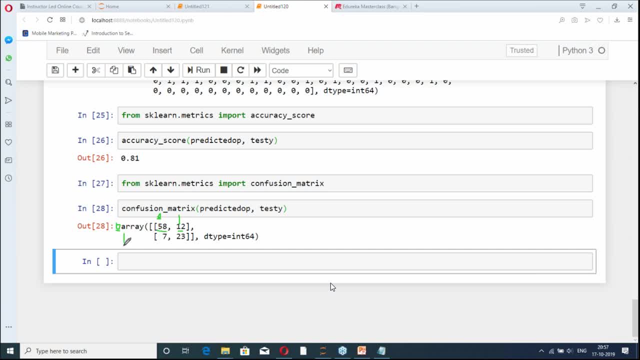 Right, so this is for the 0th. similarly, if you look the data points which belong to class 1 and predicted as zero means wrongly classified, there were 7 such values and the values which belongs to class one and predicted as a class one, there are 23 values. 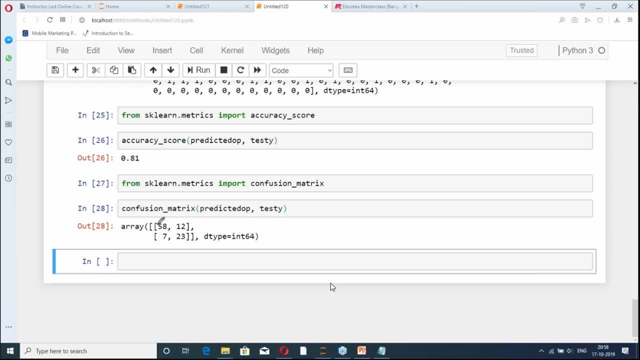 So what you can see- diagonal values here- is showing the correct values, right. So 58 plus 23 are my correctly predicted values, right, And this 12 plus seven, these are my wrongly predicted or misclassified values, right? So, with the help of confusion, matrix. 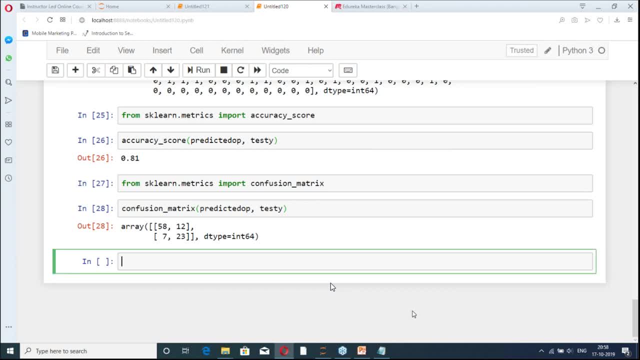 you can see exactly that your model is not biased towards any particular class, right? So you can see how much biased your data is or not. okay, So I hope so this is clear to all of you guys, right? So Farun Sharma is asking: 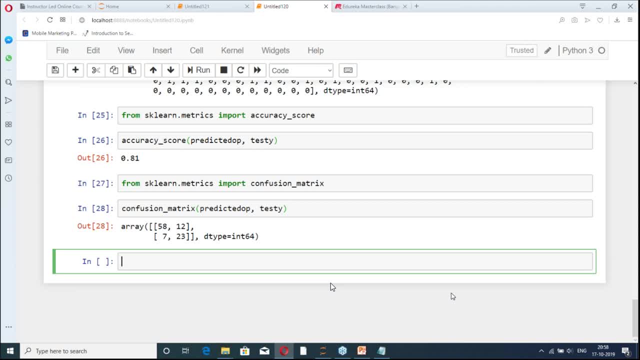 difference between min-max scalar and normal scalar. There are many different scaling techniques out there, but we are not going into the scaling technique currently in this session, Let's see. So this becomes a completely a different topic. that is, we discuss in the pre-processing techniques, right? 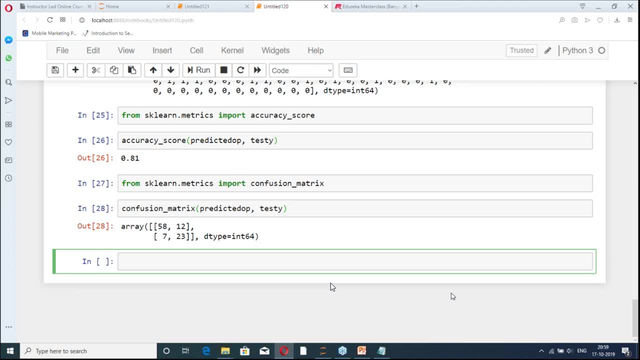 So currently, let's, maybe the Azure Agate team might design one module especially for the pre-processing, probably in the future. then there we'll be discussing in the detail, okay, Or during the courses. you can get these as well in the detail there. 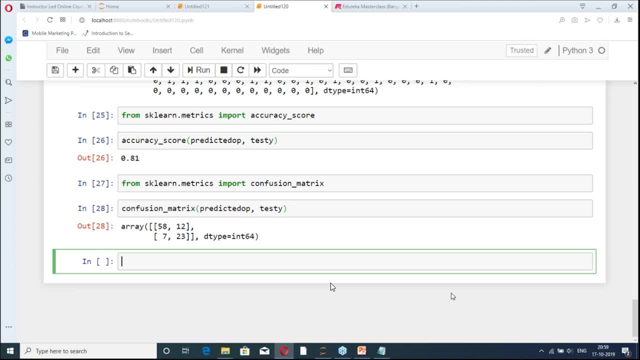 So let me see if any of you have any question or doubts related to logic. Just got the question of logic regression which we studied today. No query, No question, Great, Okay. So Jaishankar, Usually, is asking: what is the conclusion here? 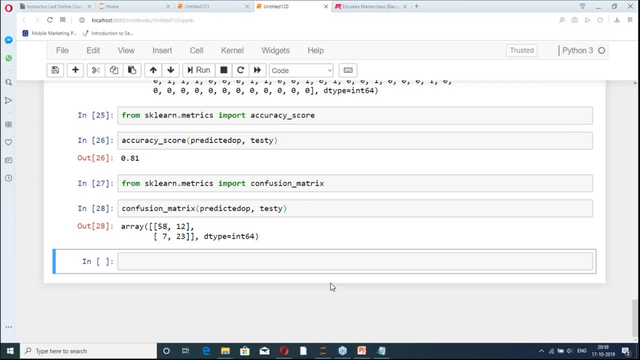 After the country, confusion, metrics. So conclusion here: after the country and metrics, is, it seems like okay, so if i have to do, let's say now i can do this, uh, this as well, if i want to find out further that how nicely my zero class has been predicted. so i can write 58 divided by 58. 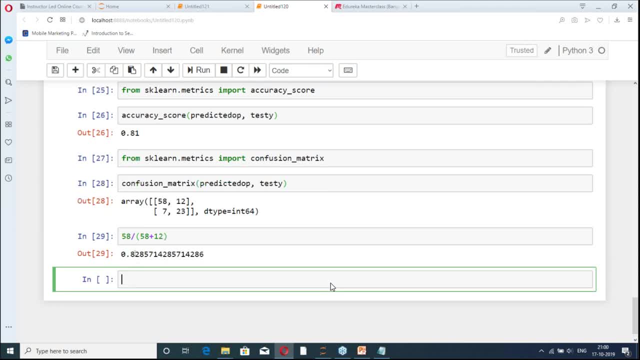 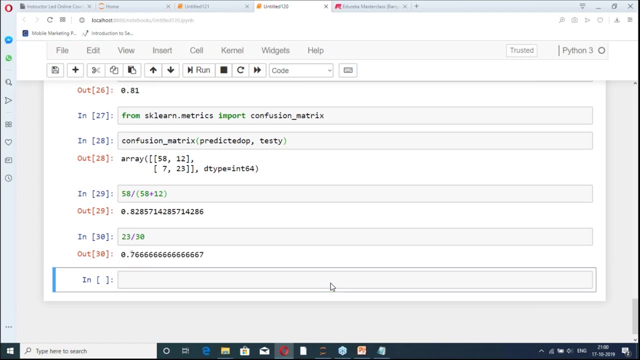 plus 12.. so i can say for the zero class the accuracy of prediction is 82 percent right and similarly for the, i can do 23 by 30 and for class one prediction probability is 76 percent right or prediction accuracy is 76 percent. so by looking into the confusion matrix you can not only so. 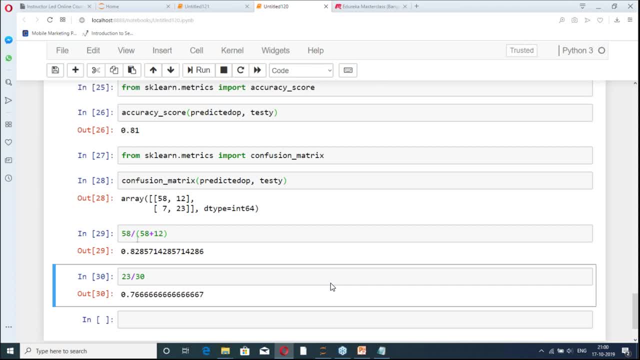 it's not only you see what is the overall accuracy, but for each class you can see how nicely your model is predicting the values okay. so that is the conclusion here: that this way you can look exactly for each and every class how nicely it is predicting and sometime it is okay for you. 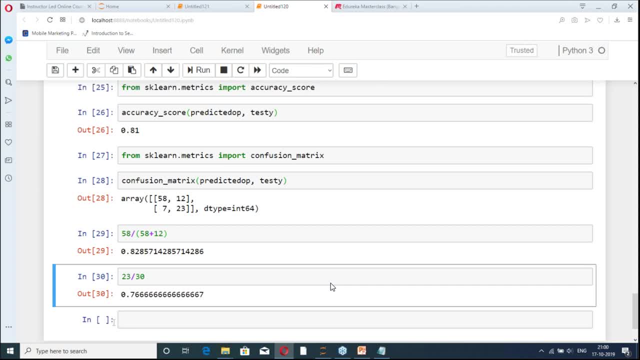 let's say: it is okay that if it predicts, let's say: let's say: if you are talking about a particular disease, right. let's say there is a particular disease. if you predict that disease as a one, right. let's say: if you predict that particular disease is happening, then a particular medicine. 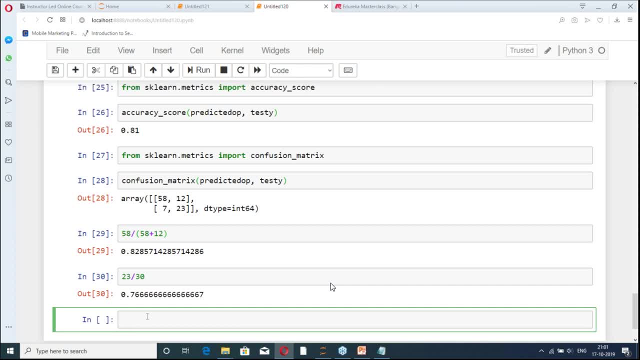 would be given to to the patient right, and if you do not predict it, then medicine will not be given to the patient right. so let's suppose this is such a disease that if a patient doesn't get the medicine on time then he will die right. but if there is some people, 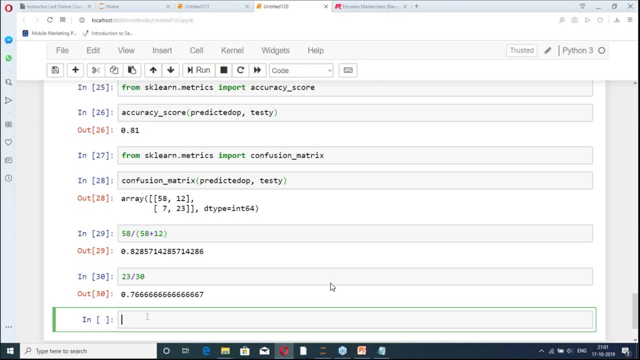 who get the medicine and even if they are not suffering from that particular disease, and if they get the medicine, is it's okay, right, they will not die. and if nothing wrong will happen, let's say there is no side effect of the medicine. so, in this case, what you would like to, 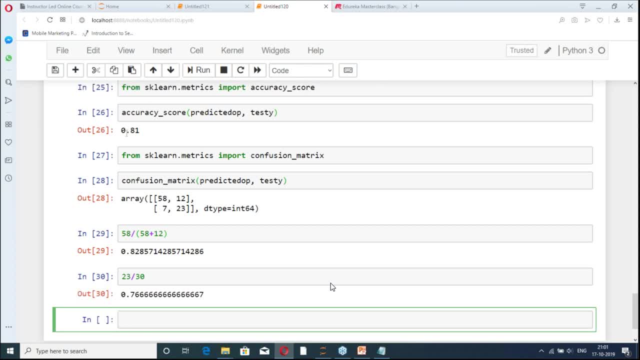 have in your system. you might not be looking at very good overall accuracy but you will look that for the for those cases where the patients, where the disease is there to a person must be 100 accurately predicted, right, those classes object should be predicted 100 accurately. it is okay if 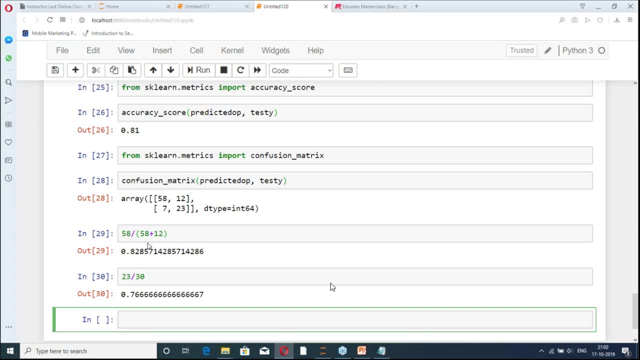 a person is not having a disease. if it is not, if it is predicted as a disease, it's fine, but if the has a disease, he must always be predicted as that he has the disease, right? so by using the confusion matrix, you can look into the details of all these classes, that how, for each and every particular. 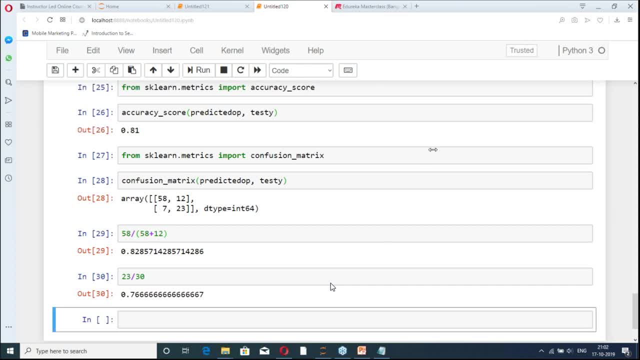 class prediction is being made okay, so i hope so. it is uh clear, jay shankar and jason racing as test data is 25 percent and accuracy- we got here and accuracy may be very or go better for different percentage of tests. is it something like that? yes, definitely. 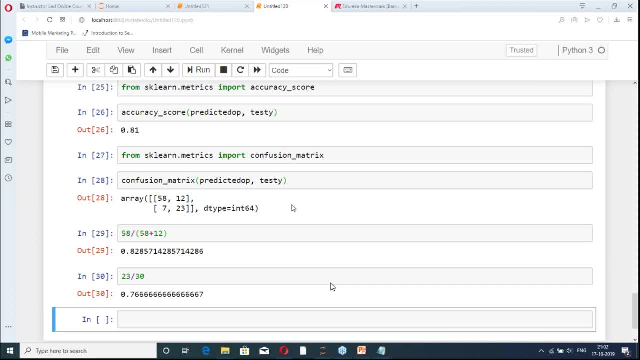 it is something like that exactly. you got it correctly. so this is a normal way we are dividing our data set actually in when you will studying them into more detail and when you will go more advanced way. then we will not do our training and testing split this way we are doing here. 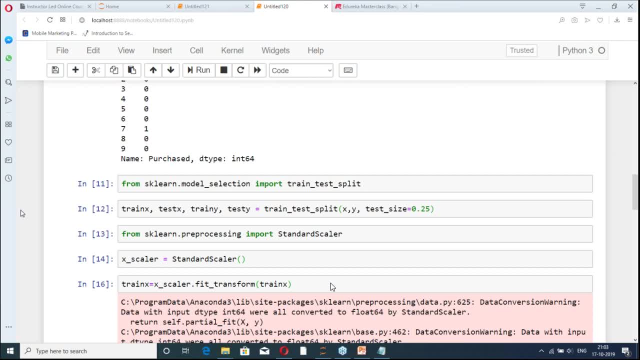 right, we will be having some better ways. there are different ways are there for dividing the data set. so, for example, sometimes even it may happen that you know in training data one particular class data is so much another class data is not much available there, while other class data is. 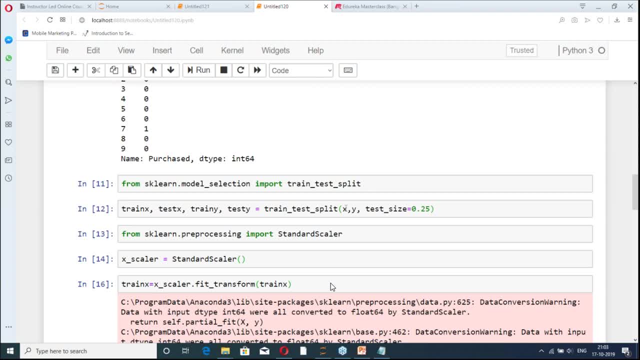 available more in the testing data set. so in this case this is not a good reason of training and testing side right, so we need to do it properly. so there are different methods. are there right and similarly here also that if you have the different testing set data set. 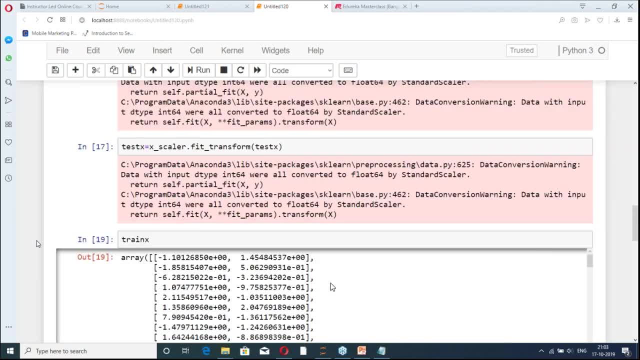 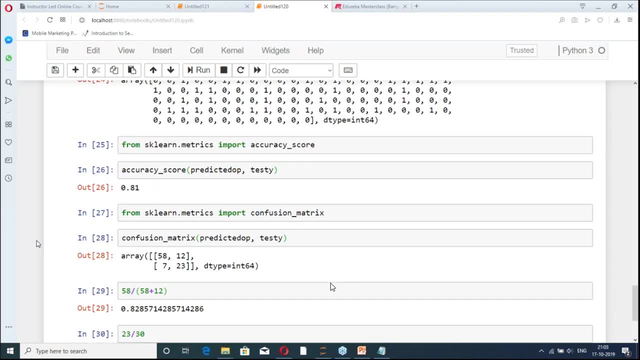 you might have the different accuracy and all. so that is why, when you will be studying little bit in more advanced way than you will be knowing, there are different methods. are there like? one of the method is a cross validation method, so we will not go into this detail, but one such method. 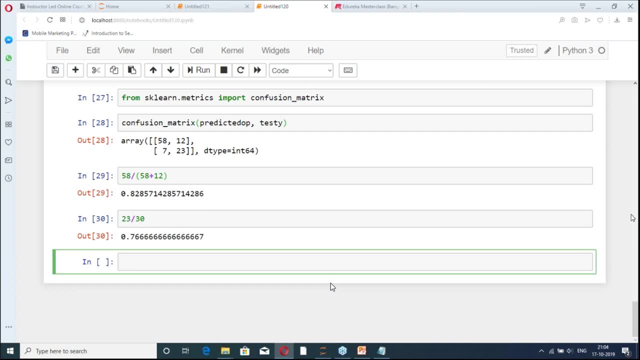 is cross validation to handle this problem which you are asking actually, and there are other things around. so i really appreciate, uh, the way practical way you are under thinking all these things. okay, any other question? yeah, okay, thanks a lot. yeah, you're welcome, jason. any other query do we have guys? 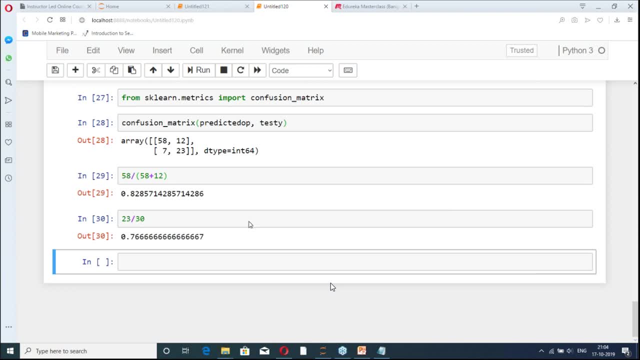 okay, no queries. webinar is trying to sing. thanks. yeah, welcome, suresh writing. thank you very much for excellent session. yeah, thank you for appreciating suresh roy- great session. yeah, thank you for appreciating roy. okay, guys, so we will finish the session if, since i will be waiting for. 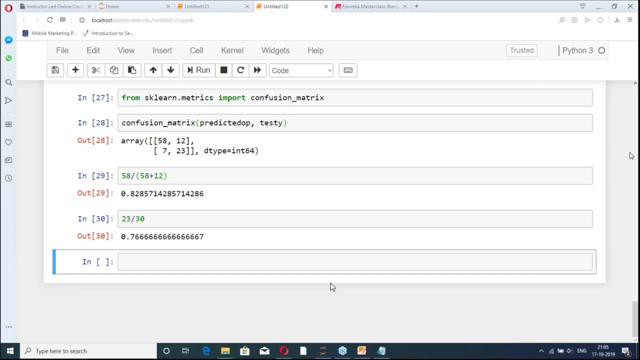 few more seconds, let's see. if there are any questions here of queries, we are getting here, so we will finish the session. if there are any questions here of queries, we are getting here, so we will finish the session. if, since i will be waiting for few more seconds, let's see if there are any. 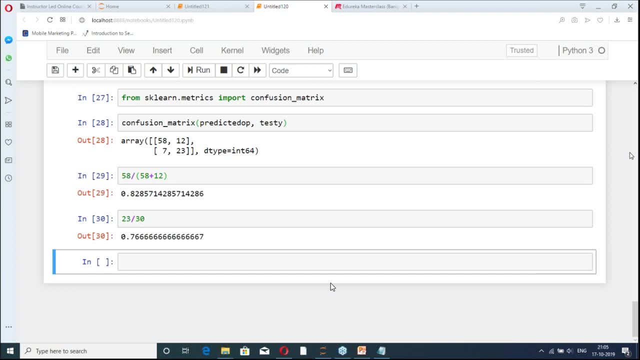 questions here of queries we are getting here. okay, thank you. thank you for the writing. great welcome guys. so let me see if any question is there from youtube. so thank you for joining today. so we will finish the session. so bahru will saying: classification report: important or not?